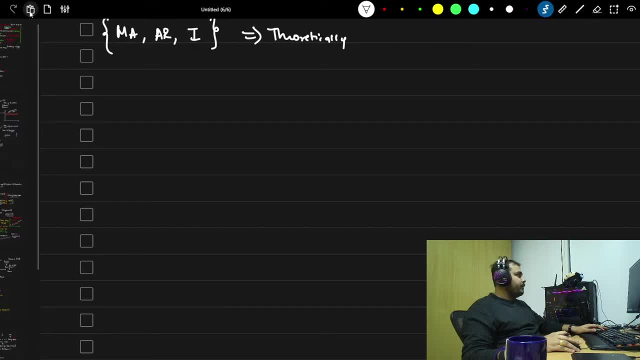 I'm just going to write the agenda of the sessions today, So let me know once we are finished. So the agenda of today's session is that, the first thing that we are basically going to complete, we are actually going to talk about Arima, and 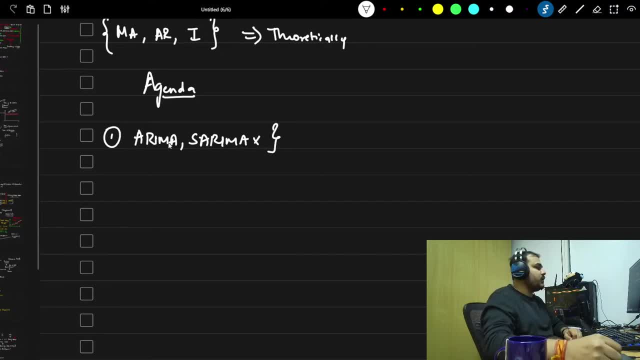 Sarik Maps. Ok, So these two things we really need to understand. what exactly it is ok And and with respect to this, the first thing that you are going to understand is something like Auto Regressive, Auto Regression. 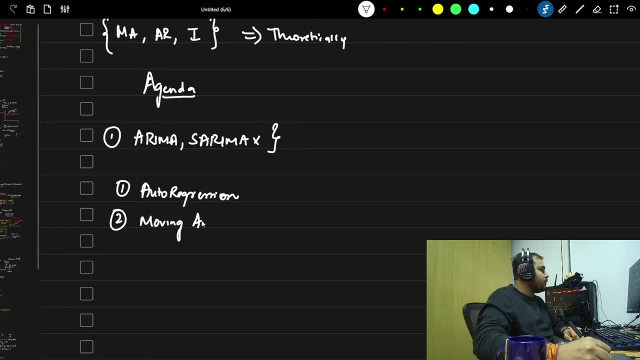 second one is Moving Average. the second one is Moving Average, which we have already discussed yesterday. the third one is something called as integrated and then, in short, we will try to discuss about ARIMA. so ARIMA, AR is nothing but this moving average is nothing but this, and integrated is. 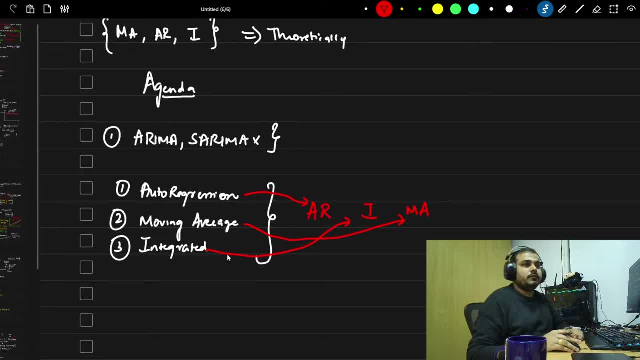 nothing but this. okay, so I hope everybody is clear with this. you can take up any data set. that is not a problem to do it from your side: auto regression, moving average and integrated. so this all things we will try to cover with respect to this. there will be more three topics that will be: 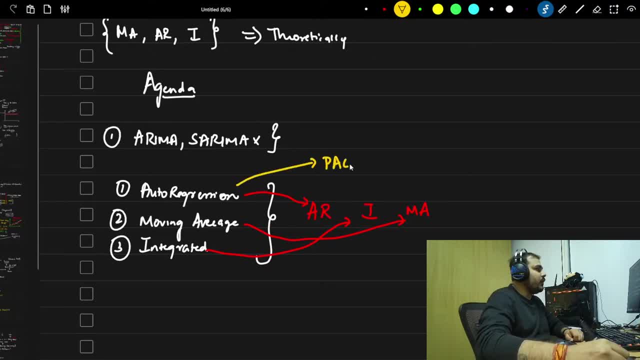 coming. auto regression is usually done by a graph, which is called as partial auto correlation. moving average is basically done by auto correlation plots, and integrated value can be found out by differentiating. okay, so we will try to find out all these three values and based on that we solve our problem. so just let me know whether you have. 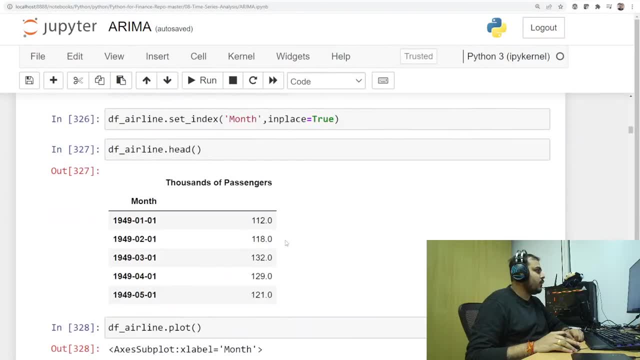 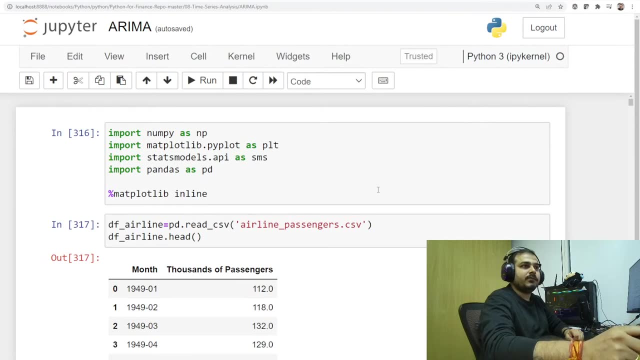 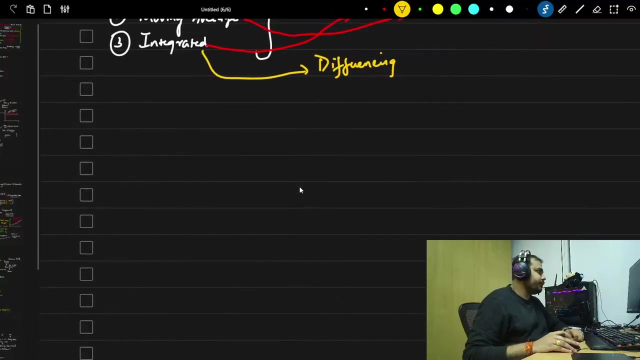 downloaded this or not? right, everybody is downloaded this, downloaded the file, so everybody downloaded the file. just give me a quick yes so that I can start. my voice is audible, guys, I guess you okay? so let's start quickly without wasting any time, okay? so first thing. first let's understand what exactly we are trying to do with. 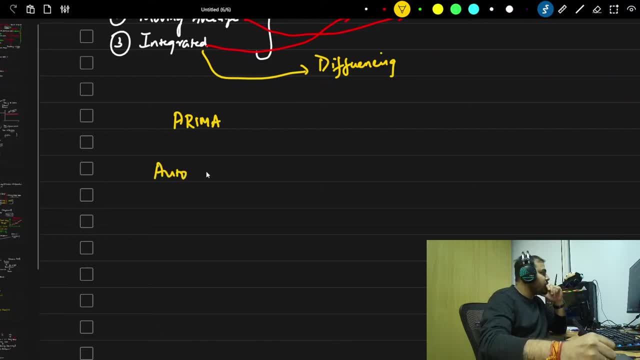 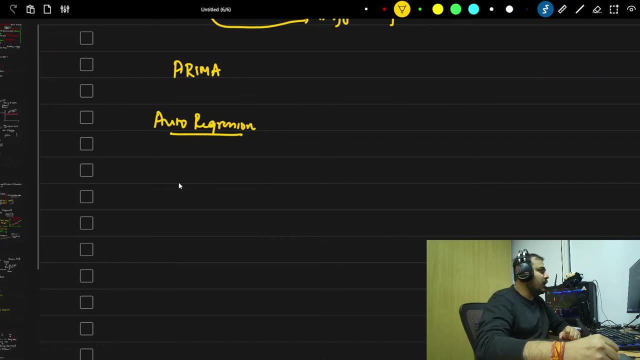 the help of our EMA model. first of all, I really want to discuss about auto regression. now, in the case of auto regression, what happens? is that okay. in the case of auto regression, what happens is that suppose I have a specific, let's say that sales of sales of all onions- okay, so suppose I have a. 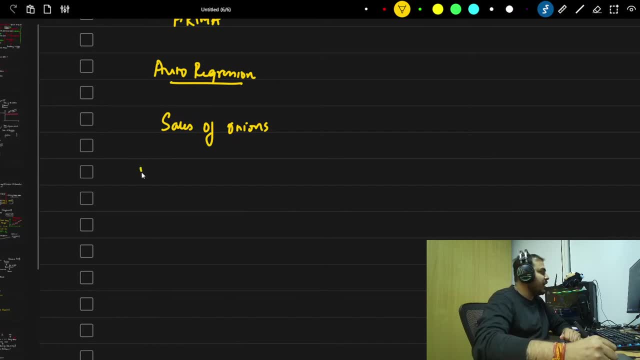 data set which is basically giving every month: what is the sales like for Jan? I have this many sales. for Feb, I have this many sales. for March: I have this many sales for April: I have so many sales. okay, so if I consider that right now it is an April month, so I will basically write. 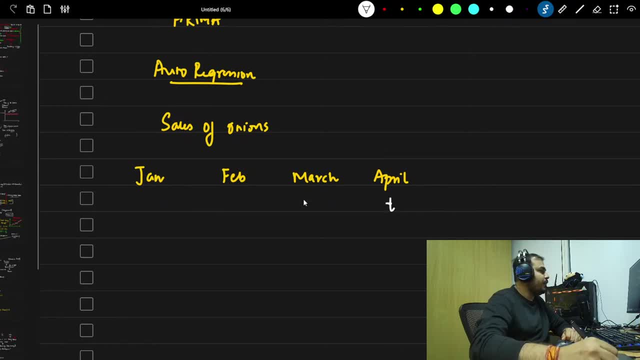 this as my T timestamp. okay, this will basically be my T minus one timestamp, and this will be my T minus two timestamp. this will be my T minus three timestamp. now, with respect to auto regression: okay, so over here you can see regression term is definitely there. okay, now in auto regression, what it does is: 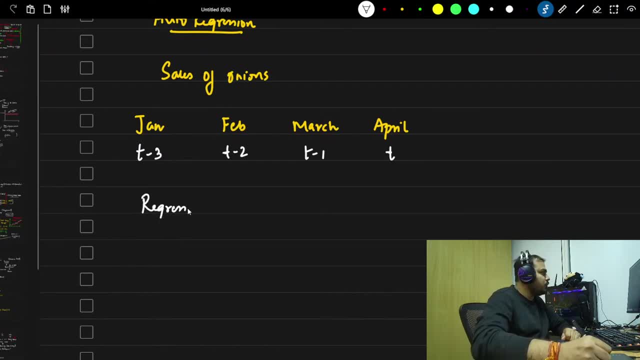 that it's just. we are just trying to apply some regression algorithm and regression algorithm in order to- in order to find that what may be the sale in May month. okay, so let's say, if I move towards May, at that point of time, this T will now. 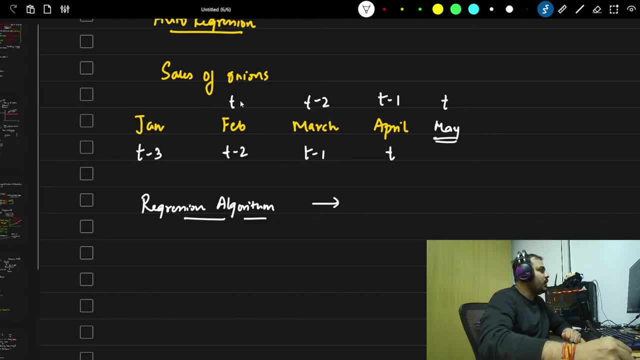 this, it will become T and this will become T minus one, T minus two, T minus three, T minus four. if I say my K value is one, one, two, three, four, suppose if I say my K value is four, that's basically means I am actually going to see the previous four months. that is T. 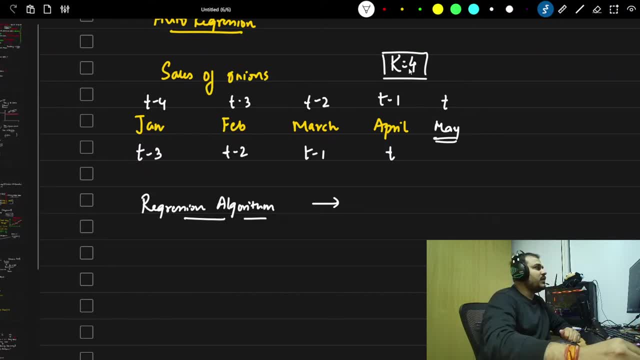 minus one, T minus two, T minus three, T minus four. okay, so this is nothing, but this is called as lags, okay, lags. in short, what you're saying is that, yes, I am going to refer to my previous data in order to find out this particular May. 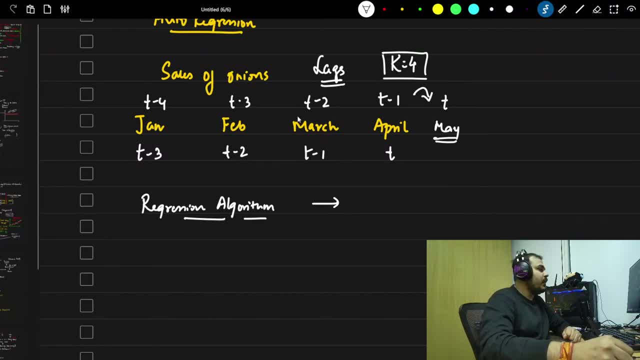 month. how much may be the sales of the onions? okay, and remember there will be an indirect or direct impact. let's say, Jan month may bring some kind of impact to the May month or probably February month may have some kind other kind of impact. March month may have another kind of impact. similarly, April month may have some 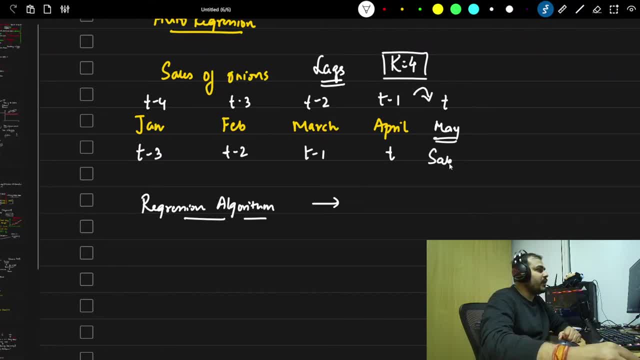 another kind of impact, or with respect to the sales prediction. with respect to the sales prediction- okay, it may be some or the other things- let's say that I have one year data, I have five years data. okay, let's say, at every time in in that, you see a, you see a kind of 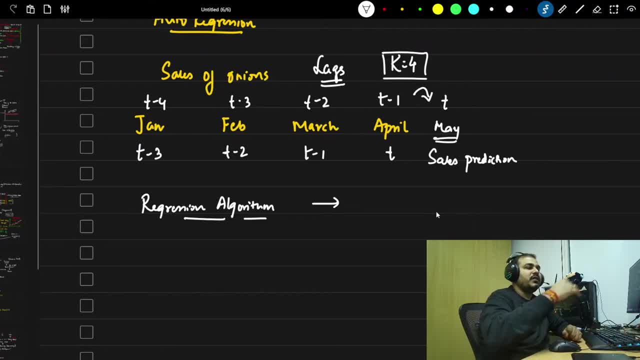 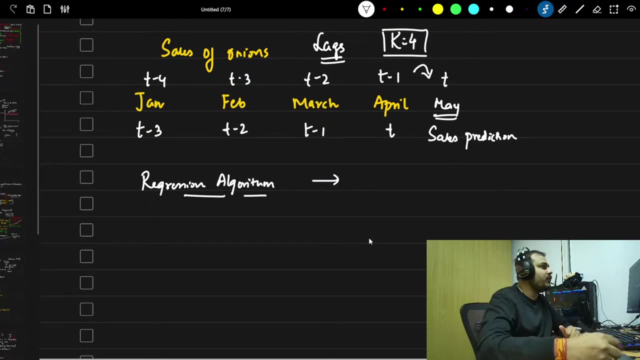 behavior, that during the month of Jan or Feb, the price of the onion is actually increasing. okay, so those kind of situation may definitely happen. okay, now in auto regression, what it says is that you are just going to use the previous, previous lags data and probably you're actually trying to find out what may be the 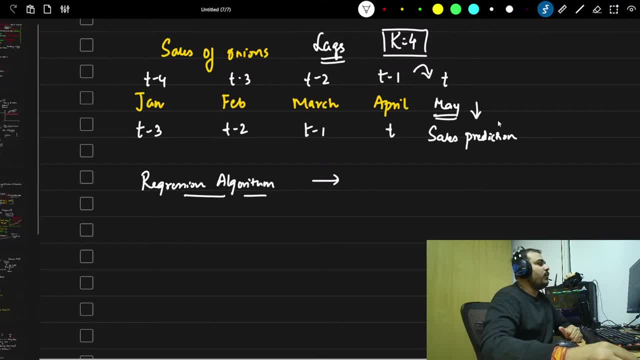 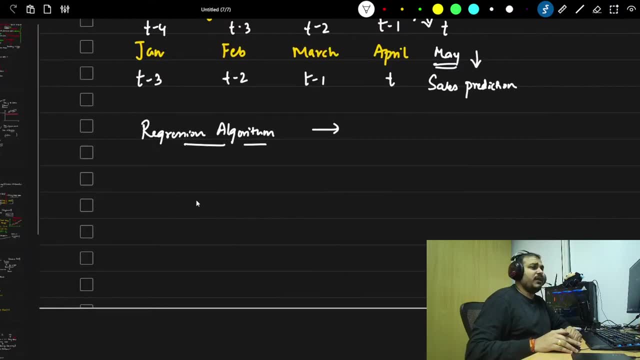 current sales with respect to the current month. so in probably, in order to calculate May sales, I will definitely prefer looking at the previous data. now, if I come with respect to an equation, let's say, let's consider only three months. okay, so suppose this is Feb, this is March and 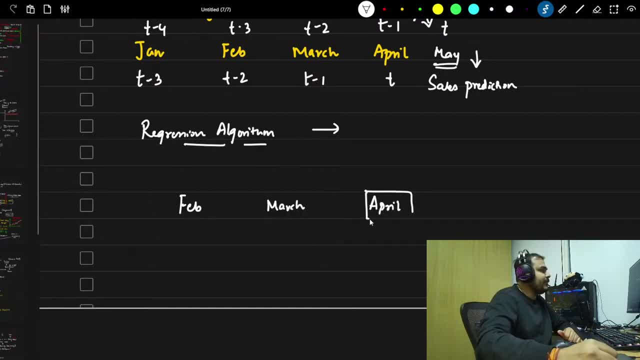 this is April. can this experiment start if I have three months data and then work it out? now? let's say we can control February month may have and direct impact on April month. okay, let's say that the next month may have the moving sales for February and so these. will depend on the data bag, since that you're using five days data on this morning, daily, and the closing date of the month may be accepted- has great effect over the following days. let's look at this moment. okay, so let's say this is Feb, this is March and this is April. 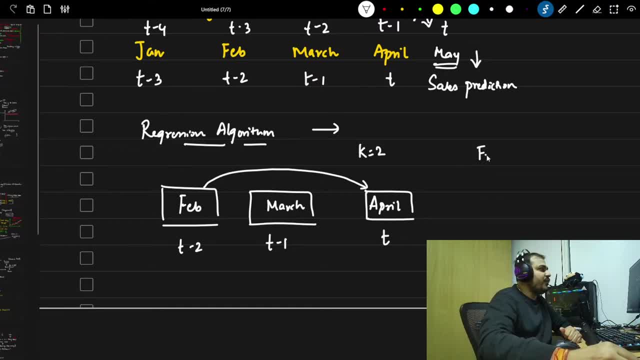 okay, suppose these are my three months data I have, let's say, my K-value is two. I want to predict past one data for one year data. what i see is that when february the sales of onion was high, probably in april also it may be high. okay, like this kind of behavior. the another behavior is: 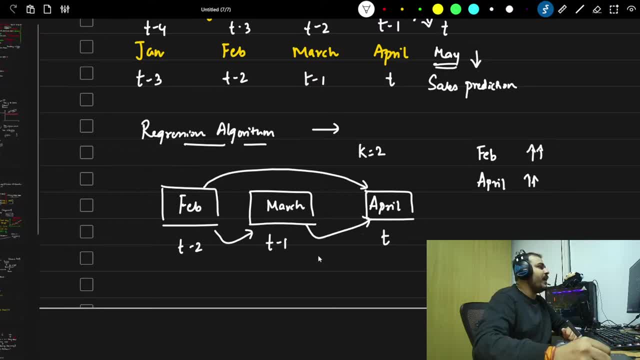 that february may be impacted to march and march may impact april april sales also. okay, so there may be some correlation between this also, and there may be one indirect correlation from directly from february to april. okay, so this kind of scenarios will definitely be there, but with 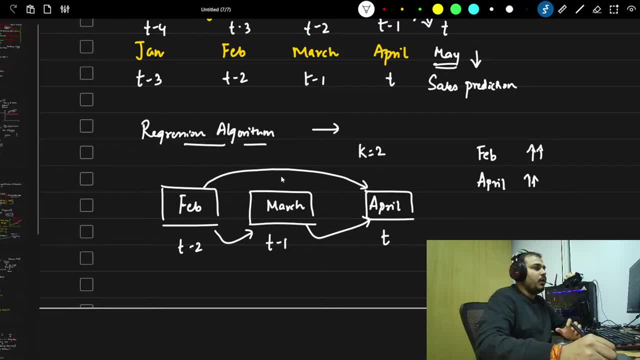 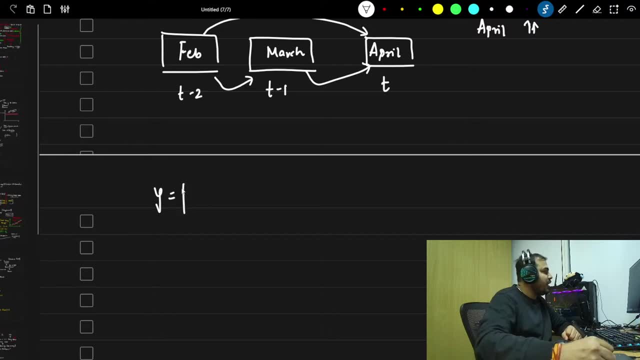 respect to auto regression. what it says is that, as you know, regression algorithm. what is? what is regression algorithm? regression algorithm, simply, if i probably try to create this kind of equation, b1, x1 plus b2, x2, right like this, up to b, bn, xn. so this is what is the linear regression formula. we 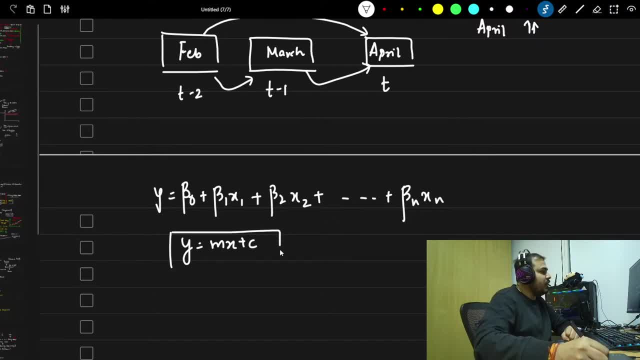 can also write it as: y is equal to mx, y is equal to mx, y is equal to mx plus c. right? so this equation, this equation, almost same, right, so this kind of equation also we can apply with respect to timestamp. okay, now suppose i change this equation a little bit. let's say this: 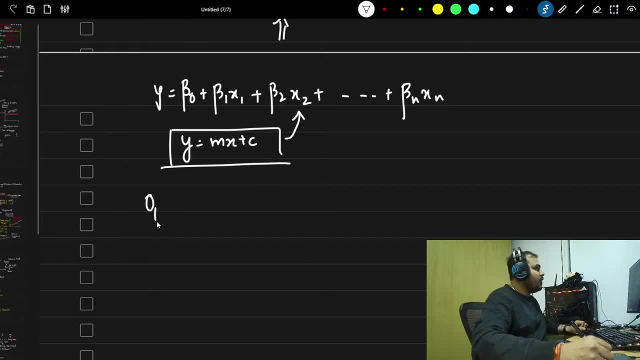 is my y. let's say this is my onion sales of onion sales with respect to time t. then what will happen? i will have on constant beta 0. let's say this: beta 1 is with respect to onion sales in t, minus 1. similarly beta 2 with: 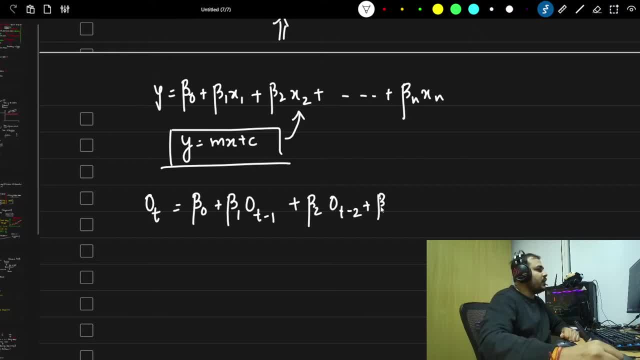 respect to: with respect to onion sales t minus 2. with respect to beta 3: onion sales t minus 3. okay, let's consider in this scenario: i just have taken two months, so i'm not going to write this- beta 3, ot 3, ot 3. okay, so this will definitely become my equation with respect to an auto regression, where i'm focusing on the previous sales and trying to predict what may be my current sales of the onion, or i'm trying to forecast it right. so this, this, 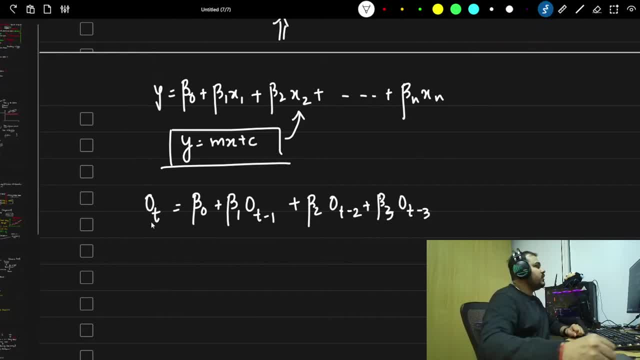 this way of this, this way that i've actually written, this, can actually become an auto regression algorithm. okay, now, the main thing is that how do i define my k value? whether the k should be 2, whether it should be 3, whether it should be 4, 5- that we'll try to see, and how we will be able to find it out. there is an amazing 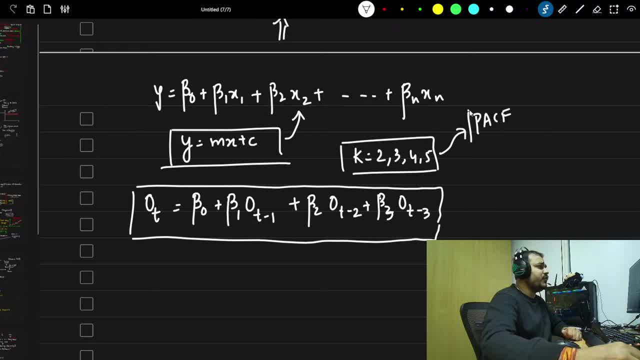 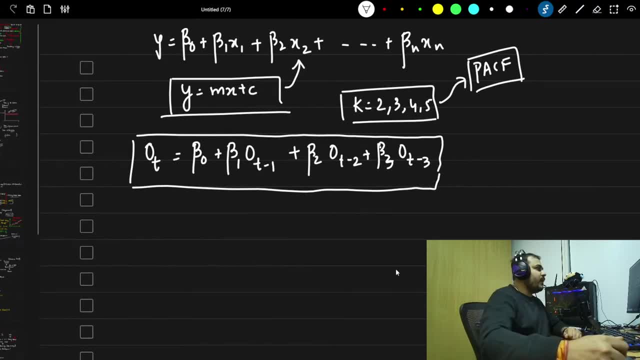 a diagram which we, which we specifically use, which is called as PSEF- partial autocorrelation. now, in partial autocorrelation, what it says is that this values that you will be seeing, this is a coefficient. this coefficients will define that how much this sales is impacting. O of T. 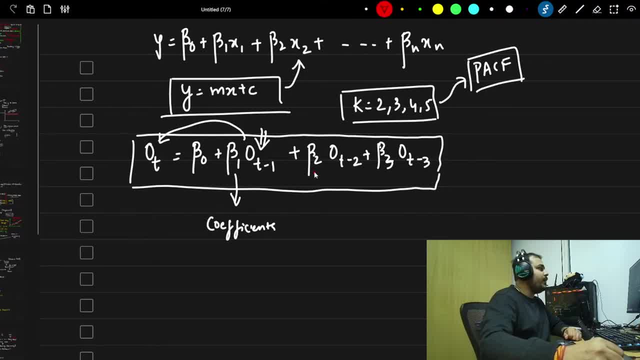 okay, based on this coefficient value. similarly, if I talk about B2, this will be another coefficient and it will basically indicate that how much O T minus 2 is basically impacting O T. okay, similarly, this will be another coefficient which will basically say that okay, how much it. 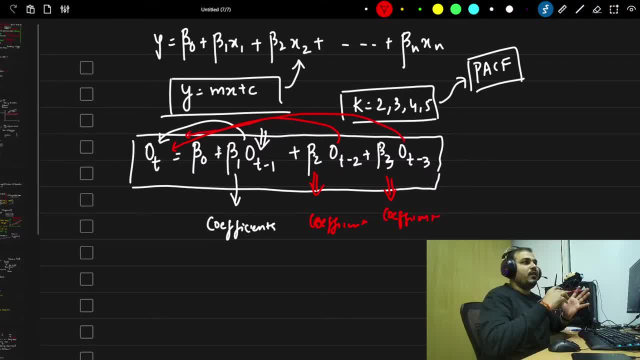 is going to impact O T. okay, so this, this kind of coefficients are there which will basically be adjusting its parameter to definitely tell that, based on the data that you have like, how much is that lag related to the current timestamp which is basically impacting the sales? okay, 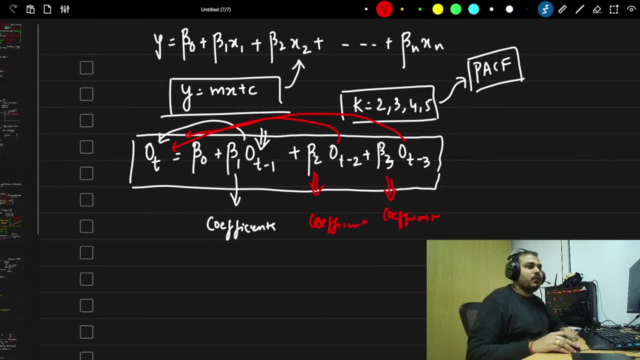 everybody clear with this. can I get a quick yes, if you are able to understand? yes, yeah, I know it is a new setup, so I'm trying something new so people may talk about it. so are you able to understand this, much or not? okay, perfect, now let's say that. 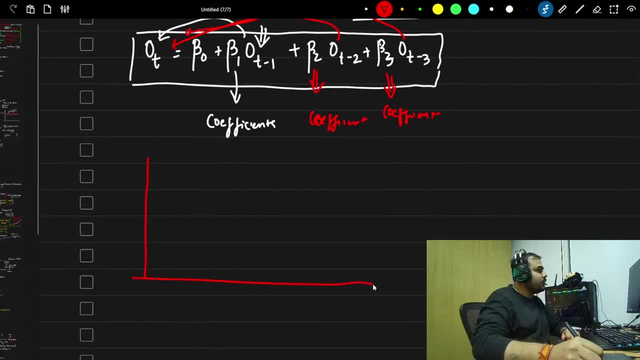 my plotted graph looks something like this. let me just show you. suppose. my plotted graph looks something like this. this is with respect to my lags. okay, I may also have a negative correlation. okay, lags basically means timestamp. okay, so if this is one, this may be two, this may be three, this may be four, this may. 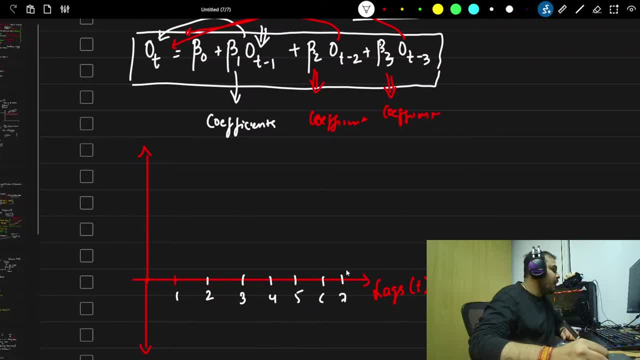 be five, six, seven, eight, like this. okay, now let's say that I'm able to. I have a 12 months data and my probably the k value may be twelve, it may be thirteen. it I. I just have a specific dataset and I really want to find. 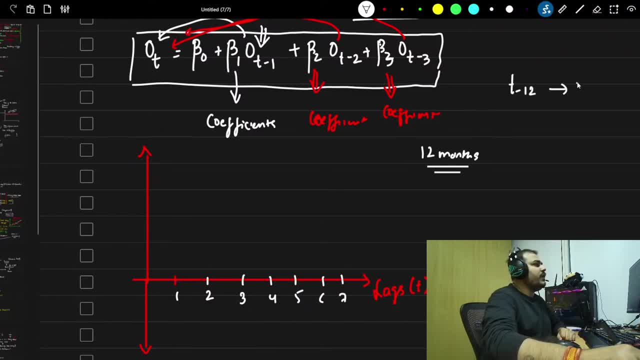 out the relation with respect to t minus twenty two t, or I want to see t minus eleven with respect to being the minus ten with respect to t. like this, I will try to see it from t minus two to p. let's say I'm just considering. okay, now what may happen is that, as soon as 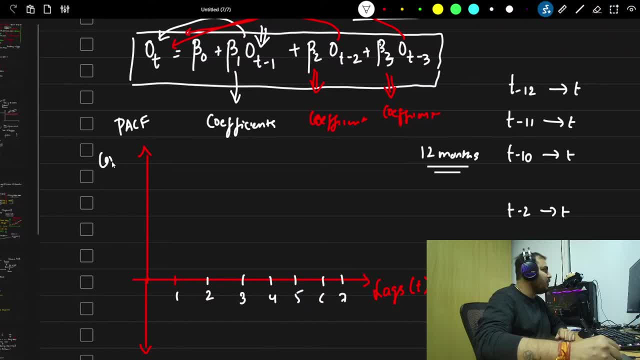 I plot this PSEF. this, basically, is giving me a correlation from a specific lag to the current timestamp. so what may happen is that i may probably get one kind of graph like this, i may get another kind of graph like this, i may get another kind of graph like this. let's say, i will also get 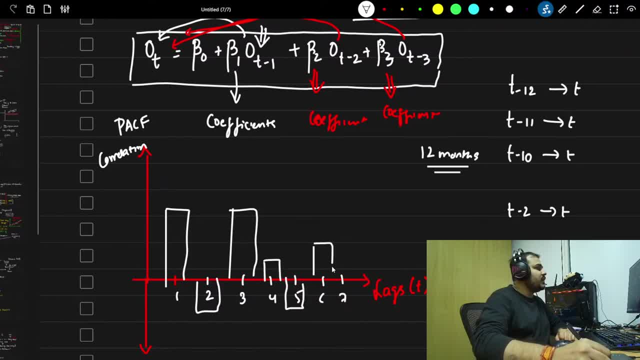 one more graph like this. i will also get one more graph like this. it may also come like this, like this: we are going to get many, many graphs. apart from this graph. it also specifies some kind of range. now, what is the specific range? you'll be able to understand, suppose, if i probably draw. 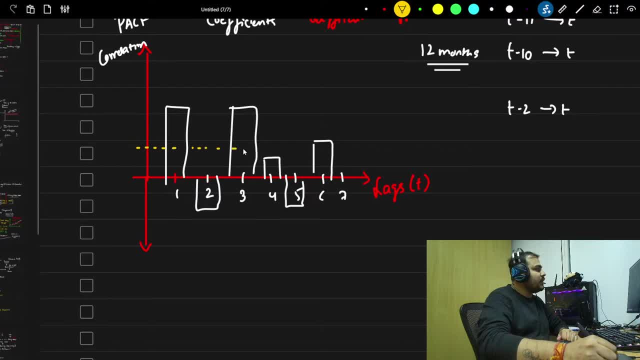 okay, suppose, if i probably draw like this one line, this line basically specifies the upper bound and the lower bound. the upper bound and the lower bound basically specifies that if it is crossing this upper bound or if it is crossing the lower bound, that basically means that this timestamp has some kind of impact on the current timestamp, and definitely it will be. 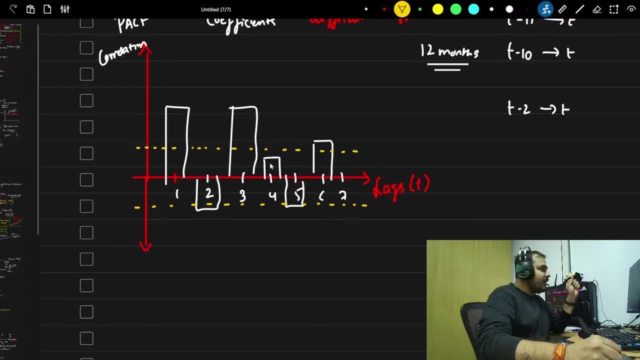 useful in calculating the sales. okay, if like this kind of graph, if it is below, if it is below this upper bound or lower bound, then what it is going to consider that they don't have any relation with the current time step with respect to the sales data. that 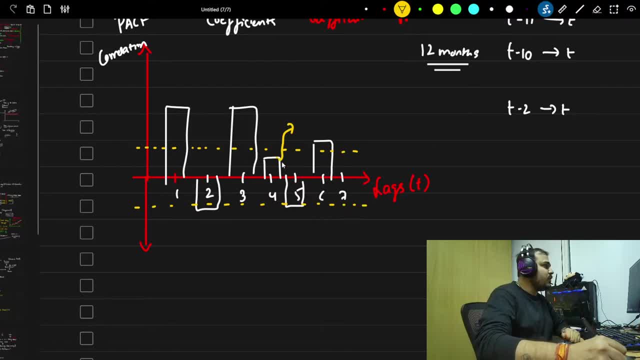 is presently there. okay, so this will not have because it is below the lower bound. so no impact. okay, no impact or no relation. you can basically say that there is no such correlation between them. similarly, over here you will be seeing that this is very, very high, so definitely this has some kind of impact. this is also, it can be. 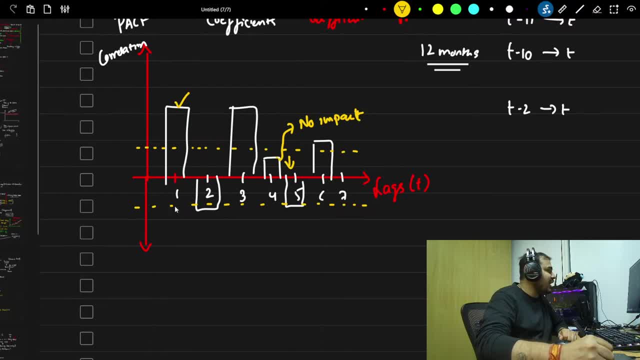 a negative correlation also right, and it is always below this line. so you can see that it is crossing this yellow dot line which is for the lower bound. so that basically means this will also have some kind of impact. this will also have some kind of impact, and this will is just in the border. so this 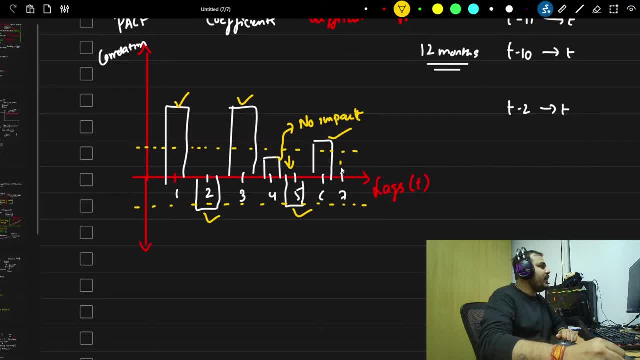 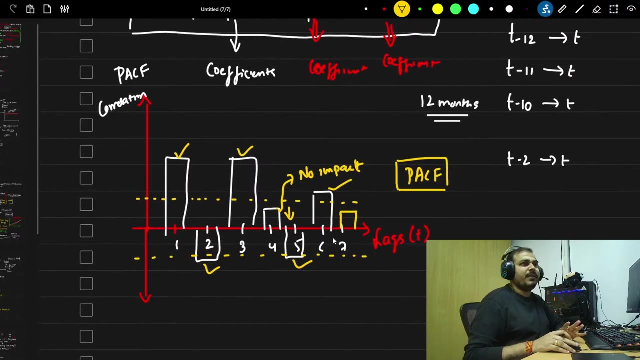 will also have an impact. this will also have an impact. any line, any, any, any correlation that is below this or below this, it will not be considered okay and there will probably be no correlation. so this graph is basically called as PACF graph. okay, partial autocorrelation, which we will also see. 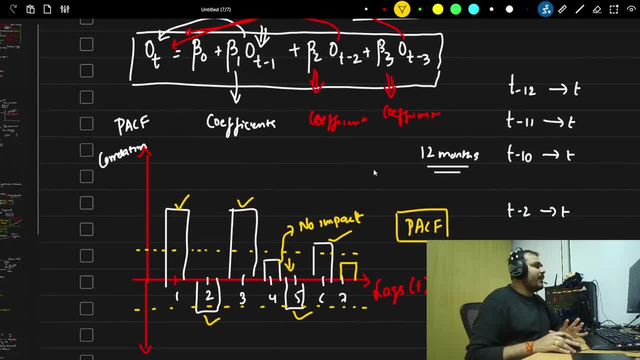 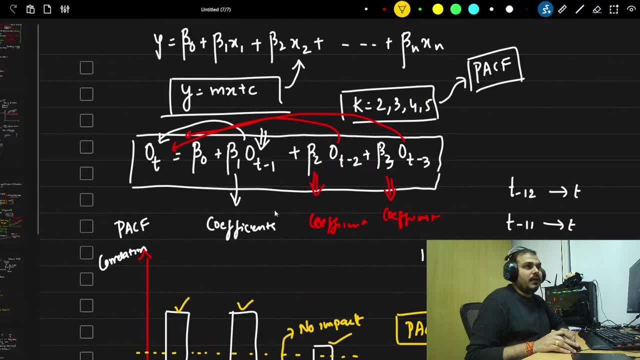 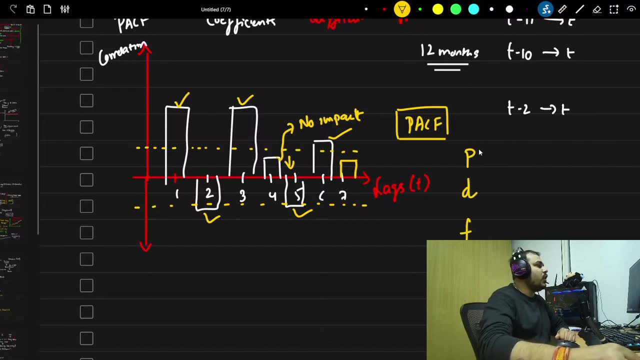 practically how to implement it. okay. so this I hope everybody is clear. so always remember: with the help of PACF graph you will be able to calculate the autocorrelation. now suppose if I say that there are three values that we really need to find like pdf I'll talk about, sorry, pdq. 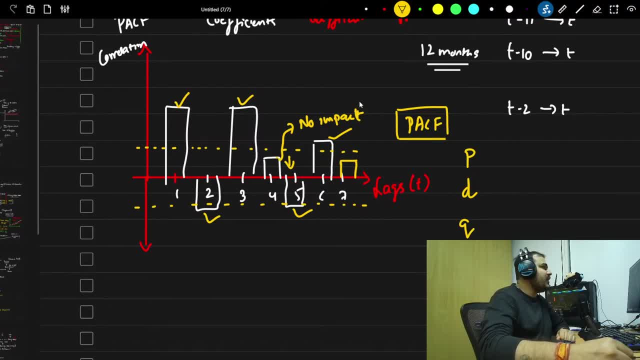 now this p is determined by this PA graph. okay, so here you will be able to see that how many, how many lines are above this? like suppose this is one point which is above this upper bound. then I have one more point which is lower, which is below this upper lower bound, right? so I can count one, two, three- this is not there- four and five. so 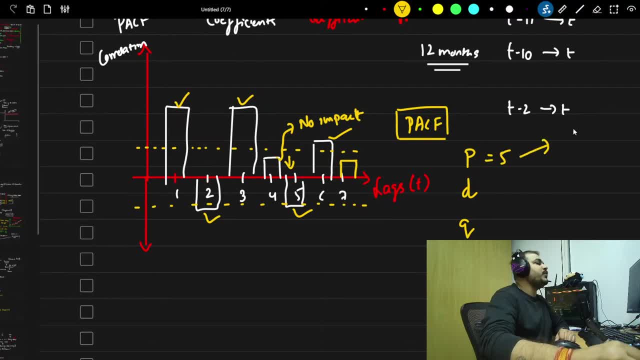 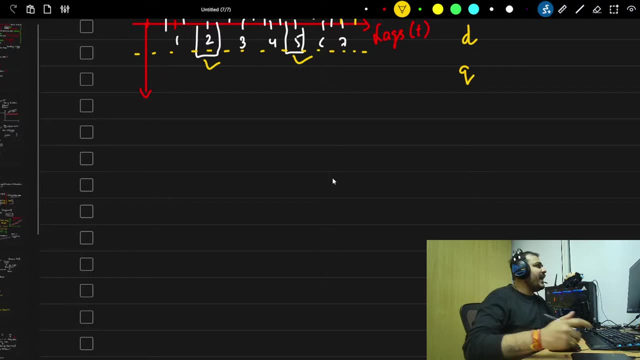 till five, I can set up my p value and basically experiment with my arima model, right? so this p is basically determined from this PACF graph. okay, this is very much clear, which I will also try to show you practically now. let's say that I have a specific data set. 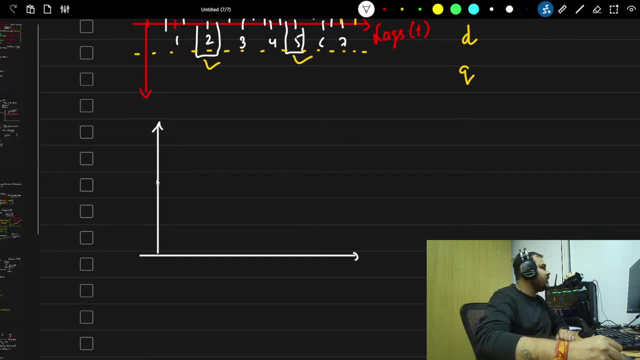 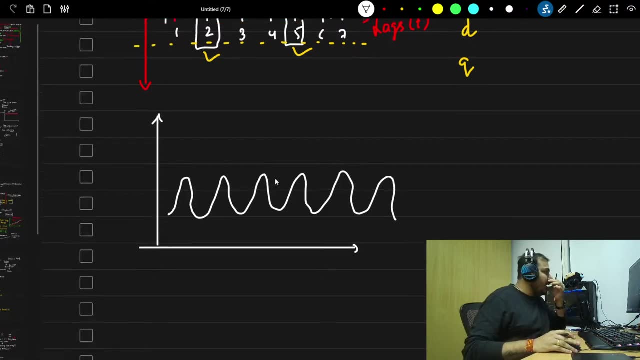 let's say, I have a specific data set and this is a kind of seasonal data, like this seasonal data. now, with respect to seasonal data, you will be able to see that when I probably try to create a PACF, when I probably try to create a PACF, 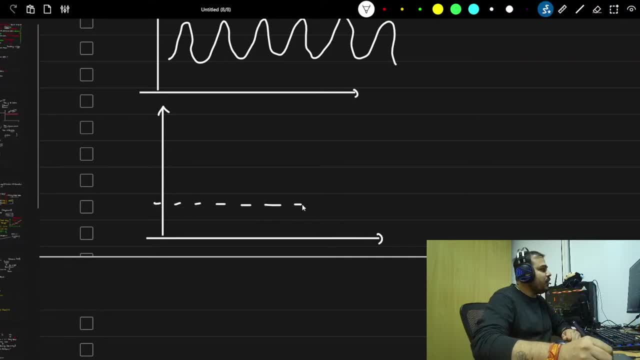 graph. then what will happen is that, suppose this is my upper month and this is my lower one. apart from the first point, every other point will be below this, like this: and suddenly, on the twelfth one, it may go a little bit high. like this, it may go a little. 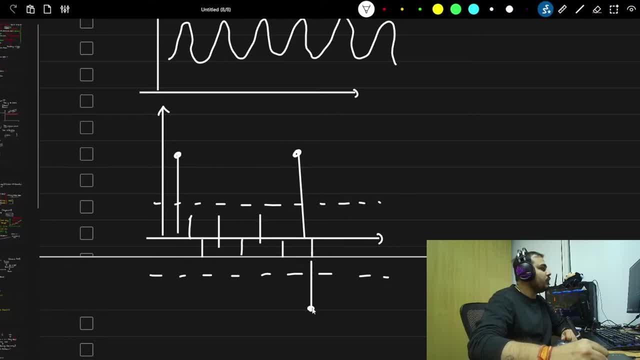 bit higher, it may go in the negative direction also. okay, now, what does it basically indicate? this indicates that, okay, it is a seasonal data, so that is the reason. right on, on a specific interval of time, you'll be seeing the value very high, and on specific interval of time, you'll be seeing a value very low. so you'll be. 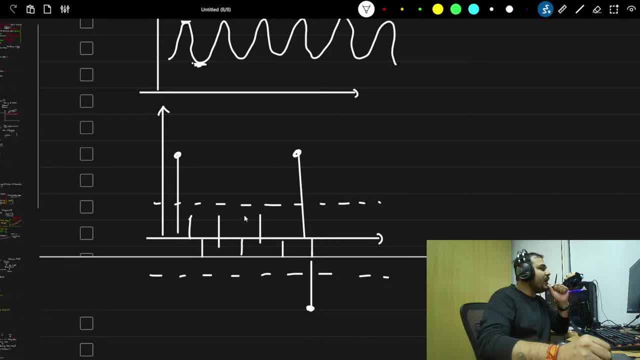 seeing that all these data points will be below this lower bound and upper bound. okay, and at one specific time, probably after 12 time stamps, you will be able to see if I am considering monthly 12 months. in the case of seasonal data, you will be seeing that it will be crossing the upper bound or it. 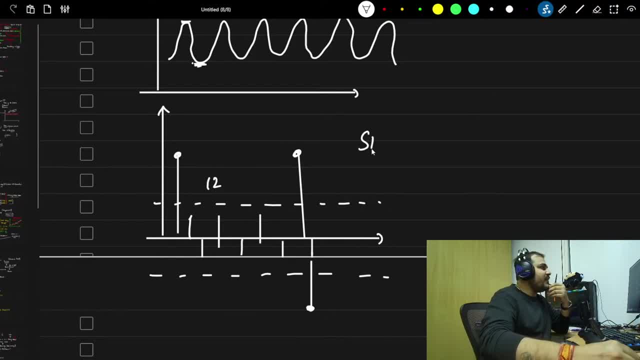 will be crossing the lower bound. okay, so this way, we basically have to apply another algorithm, which is called as Sarimax. okay, now, in Sarimax, what all information we provide? we provide our PDQ value. apart from that, we also provide seasonal PDQ value- PDQ value along with the season value, like 12. 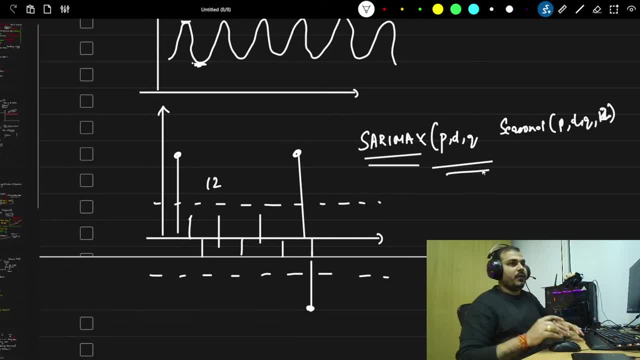 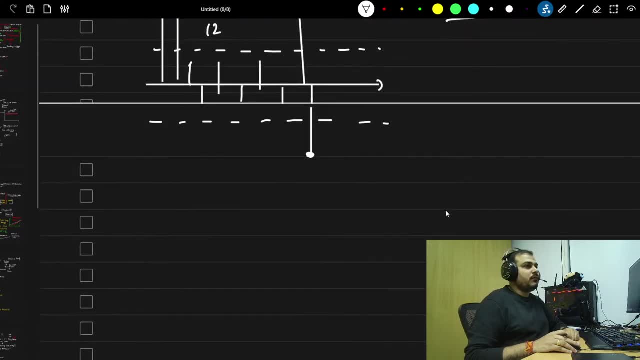 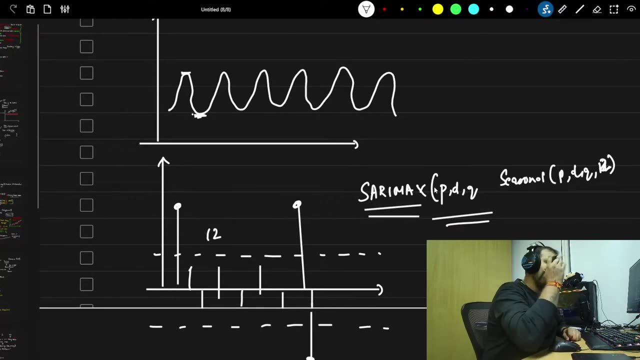 months. okay, I'll show you this when I am actually doing it practically, but I hope you have got an idea. with respect to Sarimax and Arim, okay, now the next thing is with respect to moving average. now, always, remember I'll. I'll give you an example of moving average also, but 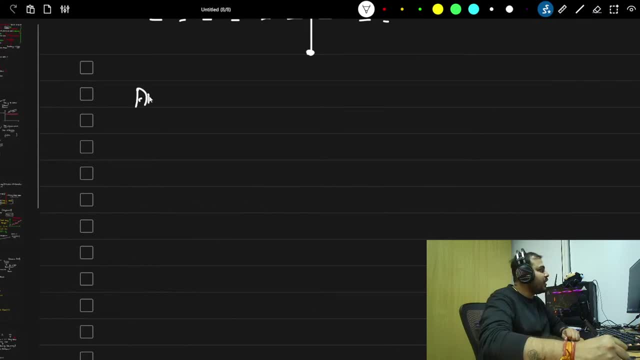 before that, let's understand- if you are probably solving an Arima problem statement- what all steps are basically there. the first step: check the data for stationery. check the data for stationery. usually when I talk about Arima or Sarimax model. this works absolutely good for seasonal data. 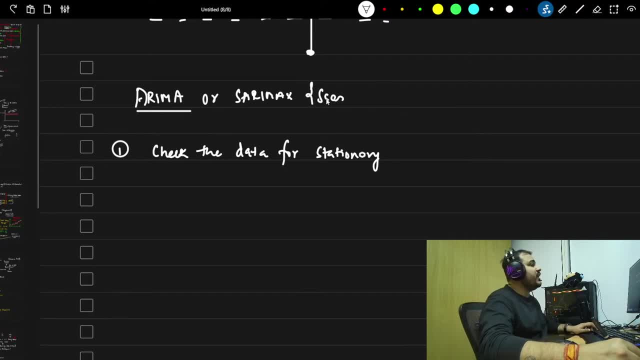 okay, but it works good for stationary data. I'll talk about what exactly- stationary data also okay. now, in order to basically check the data for the stationary, we follow some steps and that kind of hypothesis testing we do by using something called as Dickie Fuller test. now, in dickie Fuller test, what we do? we we initialize a null hypothesis and we 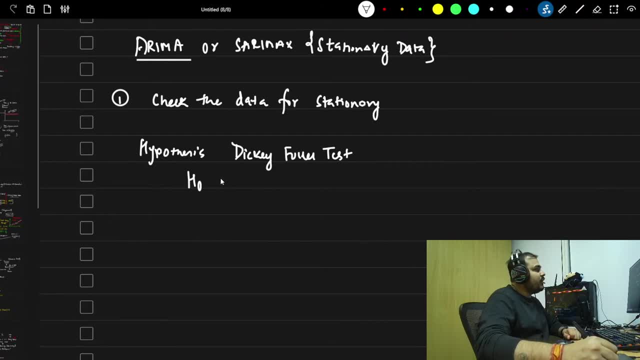 hypothesis. Now, inside the null hypothesis, what we do is that we basically say that my unit is equal to 1, unit root: I will specifically say this as unit root. Okay, Let's say I am going to write it in the words format. So here we specifically say that our unit root. 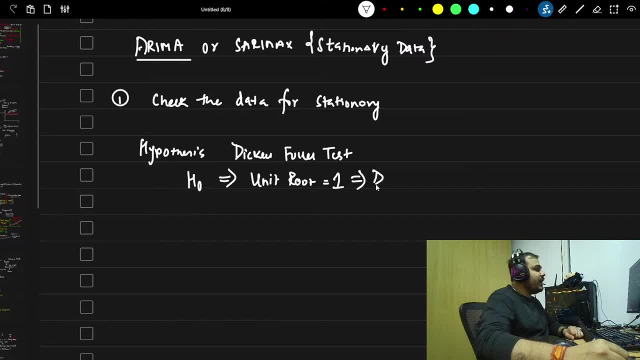 is equal to 1.. That basically means that data is not stationary. Similarly, with the case of alternate hypothesis, here I say that the unit root is less than 1.. So here we basically say that data is stationary. So this is our null and the alternate hypothesis that we 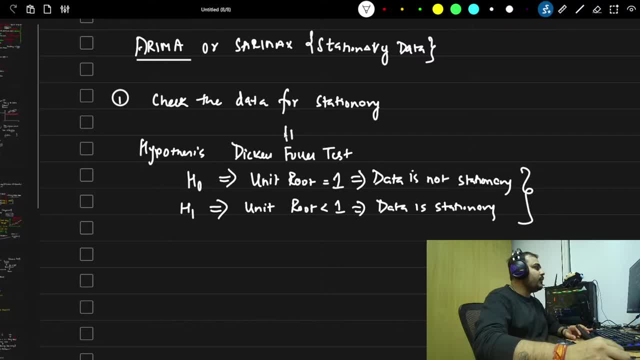 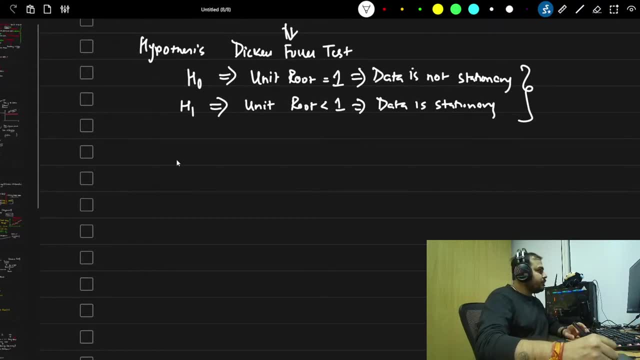 basically define. and this is basically. this test is basically done with the help of Dickey-Fuller test. Now, what does Dickey-Fuller test basically do? See this, Suppose I actually go and check, Suppose I have this seasonal data, let's say, Can anybody tell me, is this a stationary data? 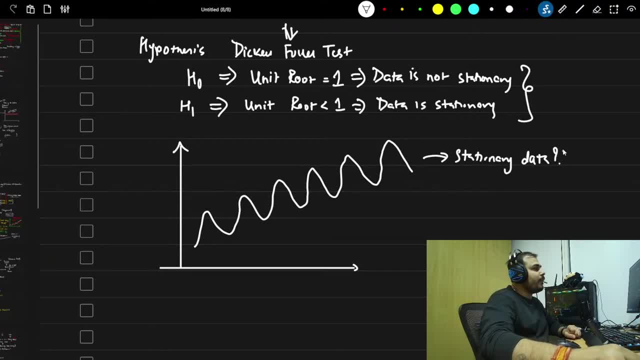 Is this a stationary data? Can anybody tell me Yes, guys, quickly, Without wasting any time, I will talk about it: unit root and all don't worry. Is this a stationary data? No, This is not a stationary data. Why? What are the condition? 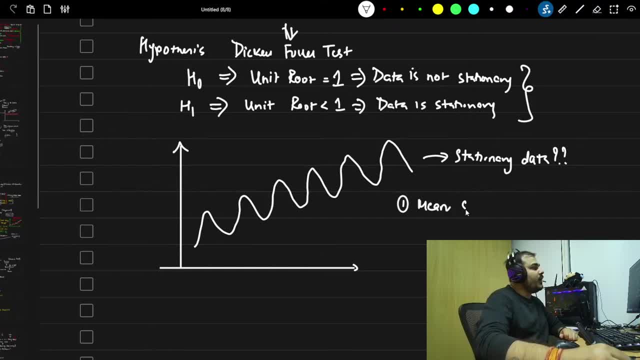 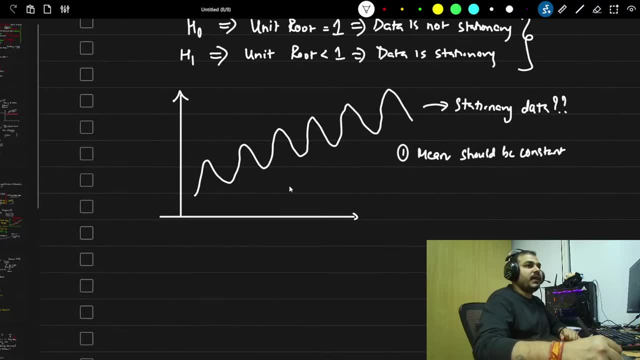 for the stationary data. First of all, your mean should be constant. The first step is this: Your mean should be constant. Second, you will be seeing that your standard deviation should also be a constant. Okay, So here you can see that, Obviously, your mean should. 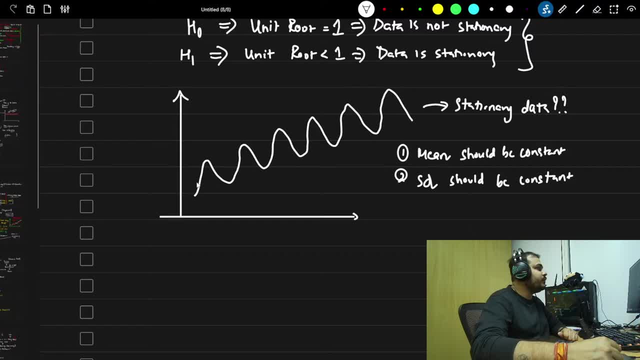 be constant. So you can see that here the original deviation is 0. If you have a standard, Obviously if I probably draw the mean and standard deviation, you will be seeing that it will be increasing. in this way, Standard deviation obviously should be constant, otherwise it will keep on increasing with. 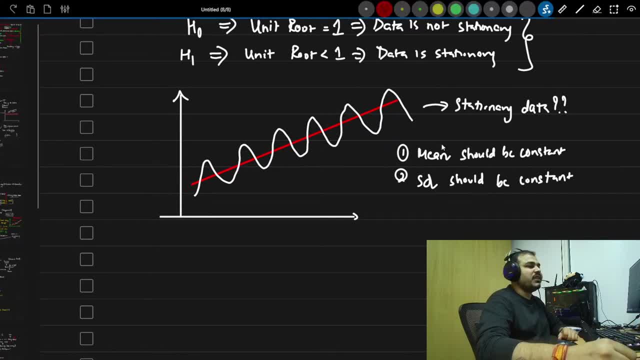 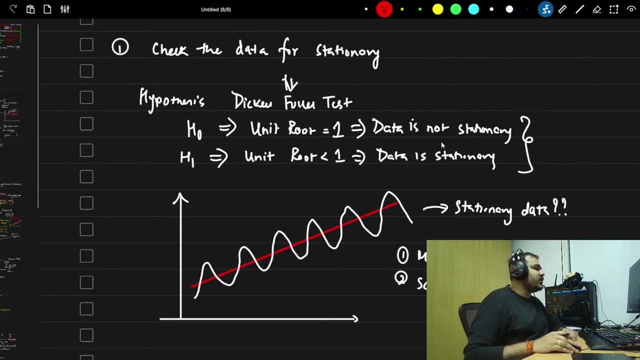 respect to the variance. okay, So definitely you can say that this is not a stationary data just by seeing visually. Now, the first step, as I said, in order to check whether the data is stationary or not, what we do is that we basically go and apply Dickey-Fuller test. 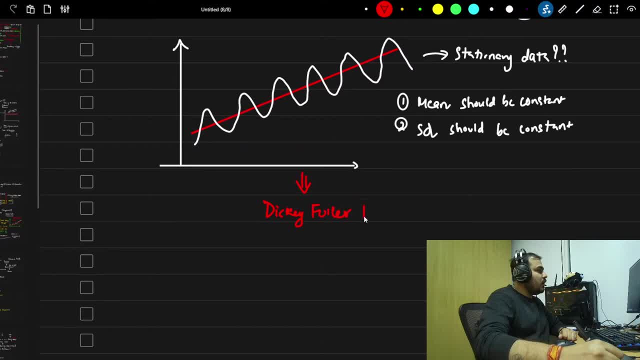 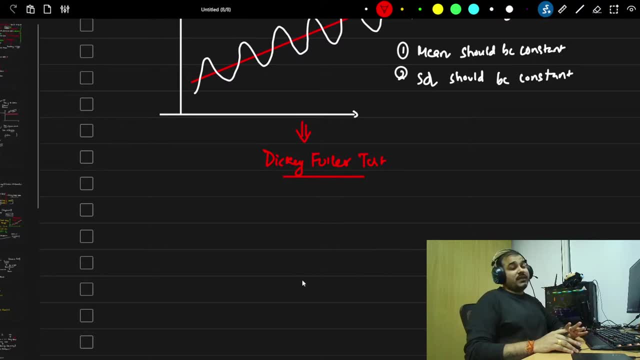 So Dickey-Fuller test. now this Dickey-Fuller test internally gives you two different values. One is the Z-statistic, sorry. one is the Dickey-Fuller statistics. we see mathematically. if I try to cover everything, it will take a lot of time. 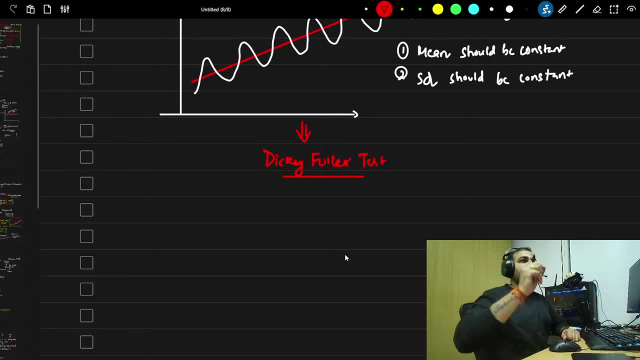 Don't worry, I will also be coming up with a time series playlist where each and every maths will be discussed Now internally here. what Dickey-Fuller test will do is that it will give you one p-value. If the p-value is less than 0.05, then what will happen is that if it is less than 0.05,. 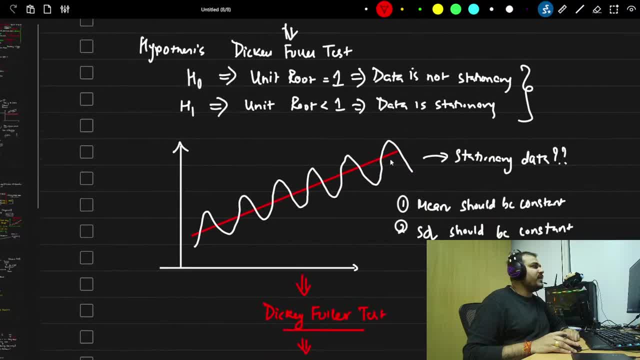 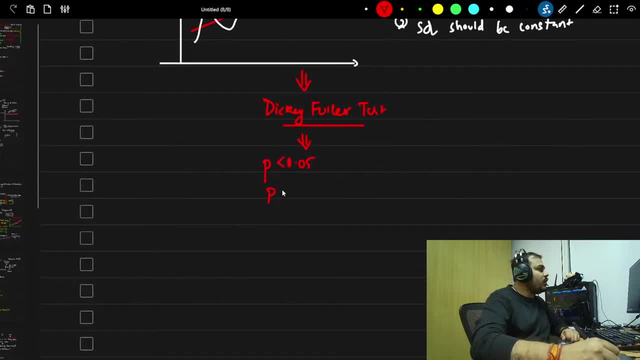 then your null hypothesis will get rejected okay. where, specifically, it is saying that data is not stationary, that will get rejected okay. Similarly, if I get p-value greater than or equal to 0.05, at that point of time, you will. 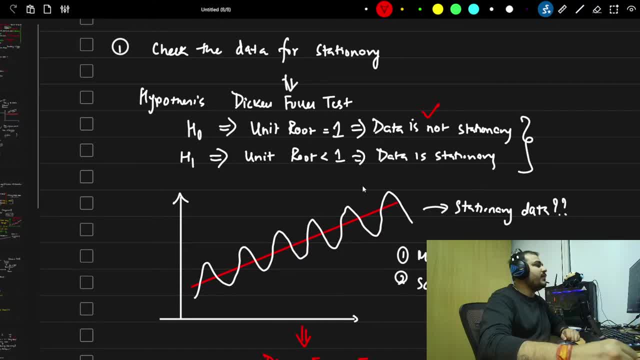 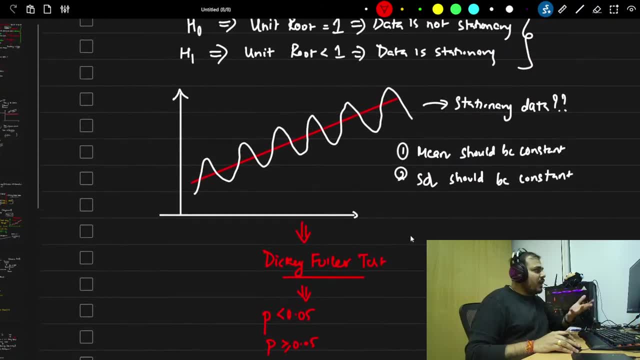 be seeing that your null hypothesis will be accepted, Where it is specifically saying that data is not stationary. okay, so this is what Dickey-Fuller test does. Now what if you find out that initially, I give this data set to my Dickey-Fuller test? 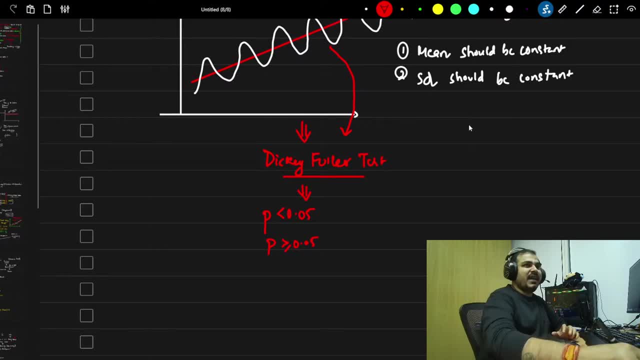 and it tries to find out. okay, with respect to this Dickey-Fuller test. and again, guys, there is a complex maths that gets applied, complex maths that gets applied. okay, If I talk about this complex maths and telling you it will take time, it will take one hour. 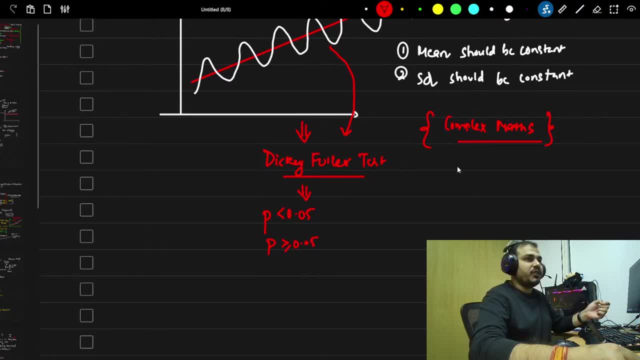 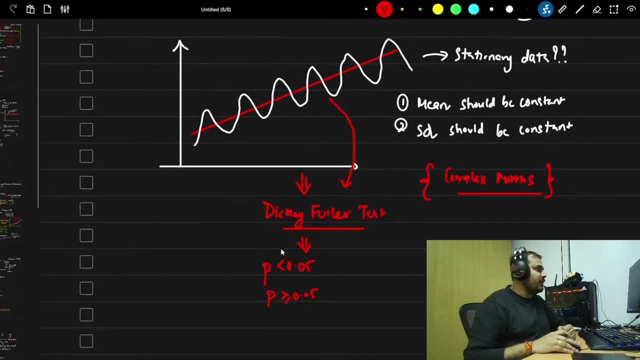 time, okay, So let me close up quickly over this. So let's go with respect to this explanation. okay, then, what I will do is that I will create a separate playlist on time series where I will discuss about each and every maths. okay? 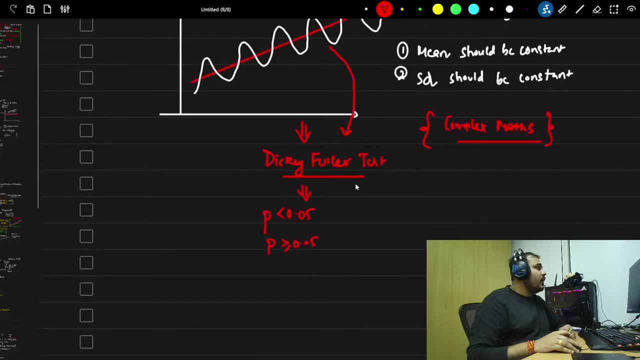 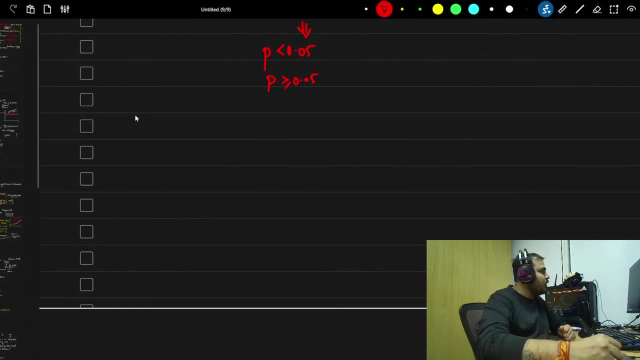 Now try to understand, because we need to implement this also. okay, Now what we do? suppose, if the data is not stationary in this particular case, then what is the next step? Let's say that I have this specific data. this is with respect to my date, this is my. 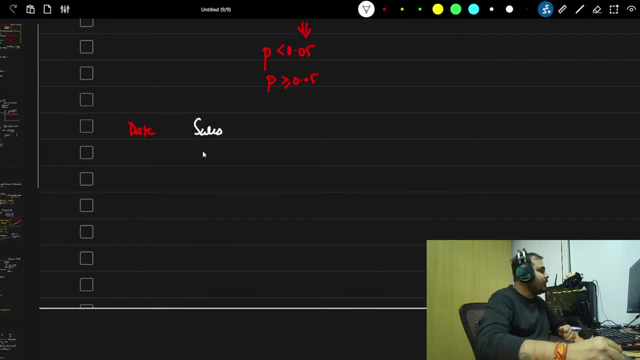 sales. sales data with respect to one year. Suppose, let's say 100, 120, 130.. Okay, 130, 140, 160, 170, 180,. suppose this data is not stationary, then what do you do? 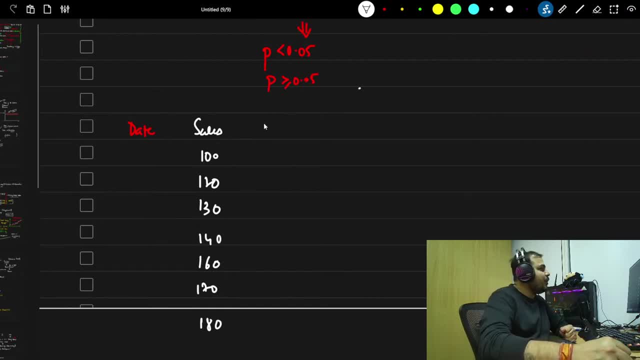 Now, in order to make this data stationary, so we basically apply something called a differencing. Now what is this step of differencing? I will show you What is this step of differencing. So we are going to do differencing. So this is with respect to T. then what I am actually going to do is that I am just 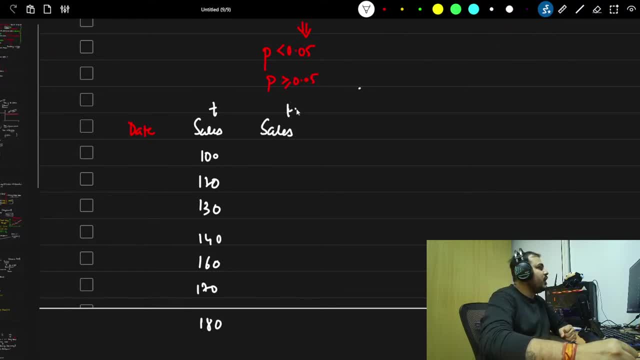 going to shift By one position, So this will be sales with T minus 1, where I am specifically shifting this data by one step. When I shift this data, so this will basically become 100,, then 20,, then 130,, then 140,, 160,. 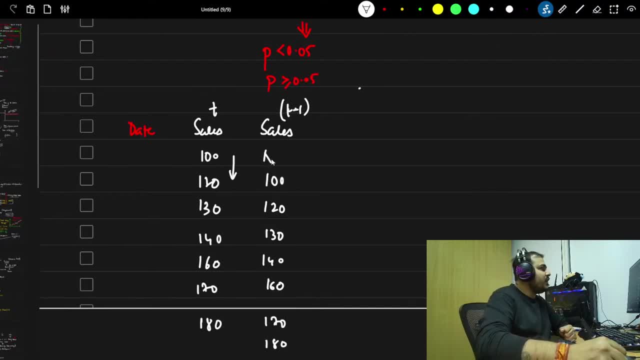 170 and then 180.. Now, what will happen in this particular case? this value will become NAN- okay, When we are shifting, I don't have anything over here- and this value will get deleted, okay, Now, differencing is basically saying that you just need to find out the difference value. 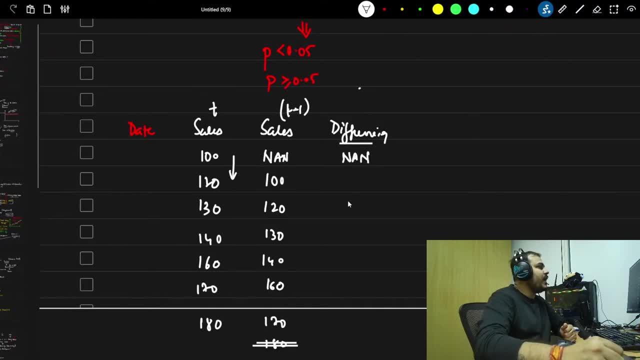 okay, What is the difference between them? So, in this particular case, 100 minus NAN will be a NAN value. then you have 20, then you have probably 10, 10,, then you have 10,, then you have 20,, then you have 10,, then you 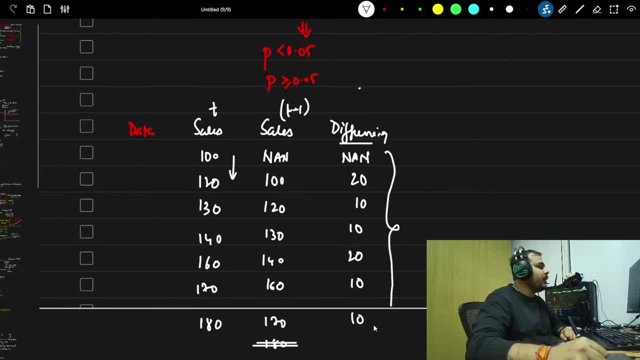 have 10.. Now, in this particular case, when you do this differencing- okay, suppose this is my first differencing- Now, in this particular differencing what we do, we provide this entire data. We provide this entire data later to our Dickey-Fuller test again. 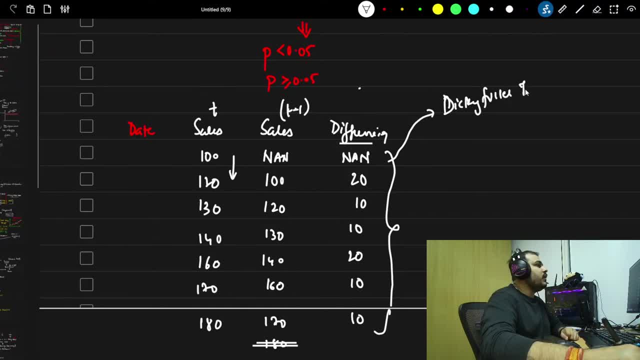 Dickey-Fuller test. Okay, Dickey-Fuller test. And then again Dickey-Fuller test will check, with respect to the p-value, whether it is less or greater than Okay. So if probably, this entire thing gives you a value less than or greater than 0.05, based. 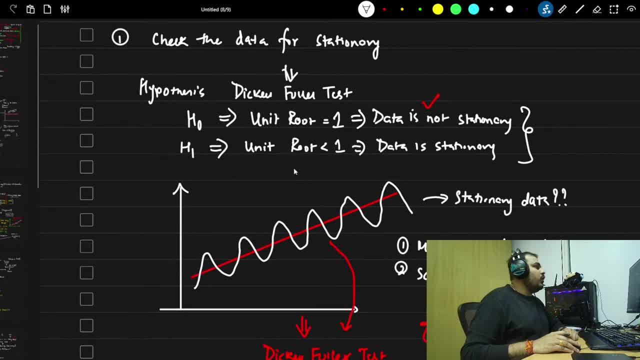 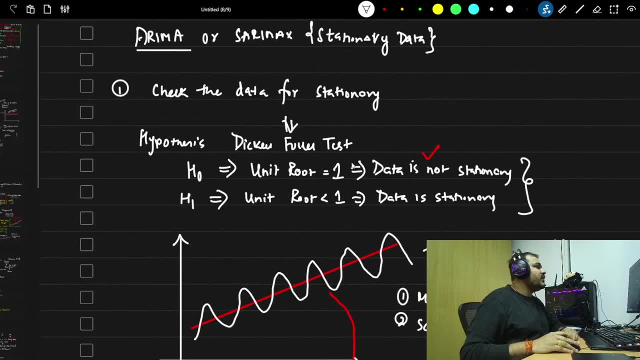 on that you can specifically take the decision. okay, So, unless and until, probably once, you get a probability greater than 0.05, so then what will happen? The null hypothesis will get rejected. sorry, p is less than or equal to 5.. 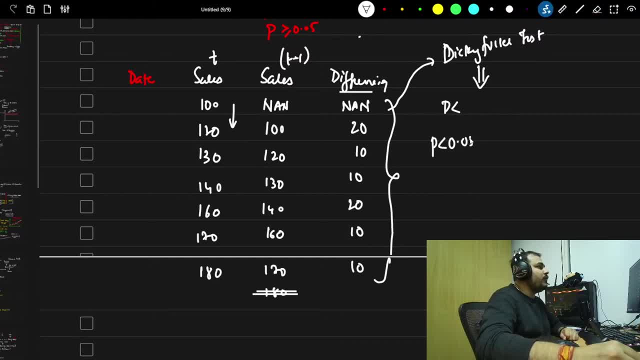 When you get p is less than or equal to 5, less than or equal to 5, at that time, what will happen? The h0 will get rejected and, based on that, it will say that, finally, you are actually being able to get a. okay, you are able to get a stationary data. 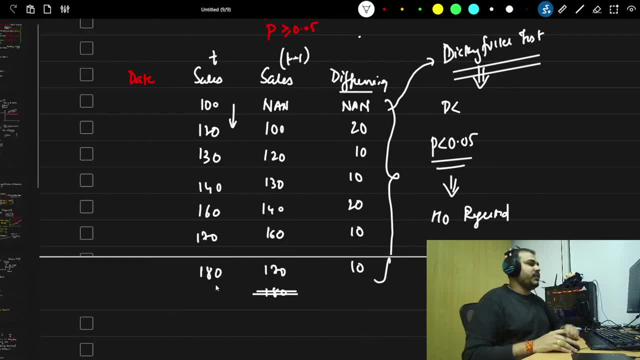 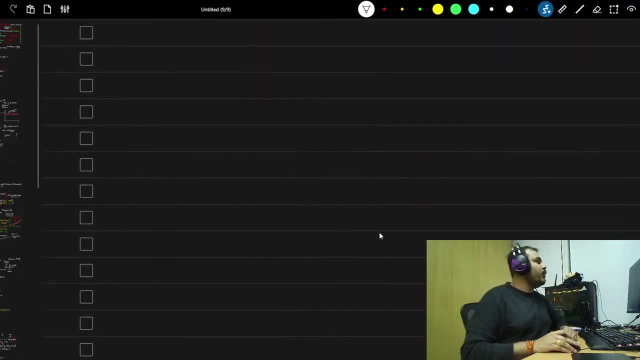 So this step we basically perform with Dickey-Fuller test. This is the first step. Now, once you get a stationary data based on this, based on this differencing how many number of times, you are doing the differencing. As I said, 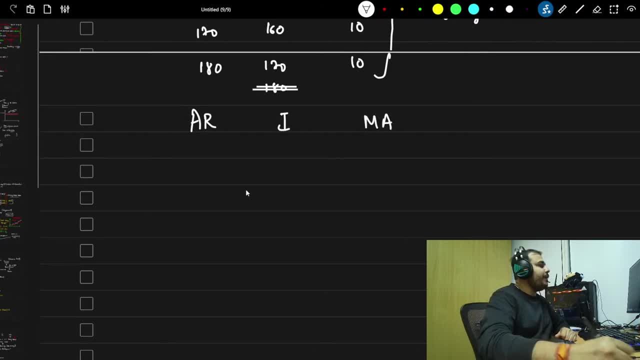 In ARIMA, A-R-I-M-A In ARIMA we find out this main three parameters: p, d, q. So the d value will basically specify the number of times you are basically differencing. okay, Suppose you did two times differencing, then you will probably write it over here. 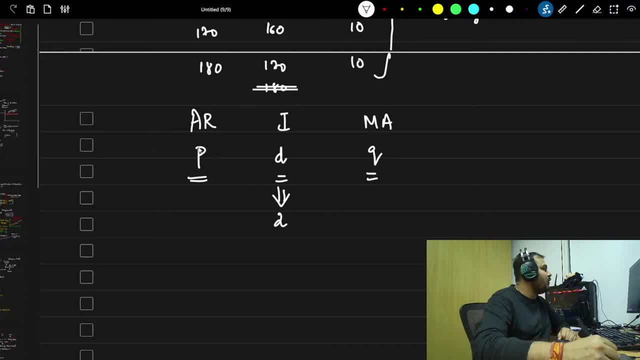 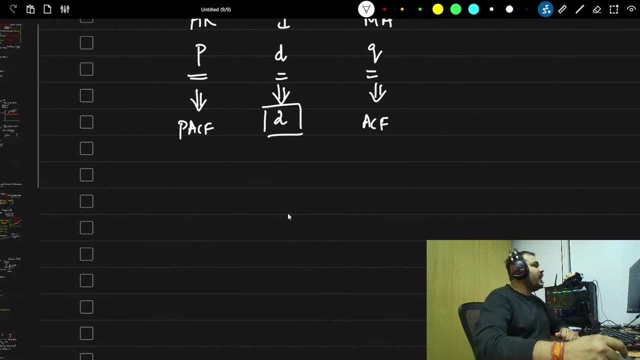 If you are probably doing A-R of this, this is basically calculated from the PACL And this is calculated from the ACF plot. okay, And this basically specifies that how many number of time differencing you are doing. okay, And then, based on that, the ARIMA model, where it will combine this autoregressive moving. 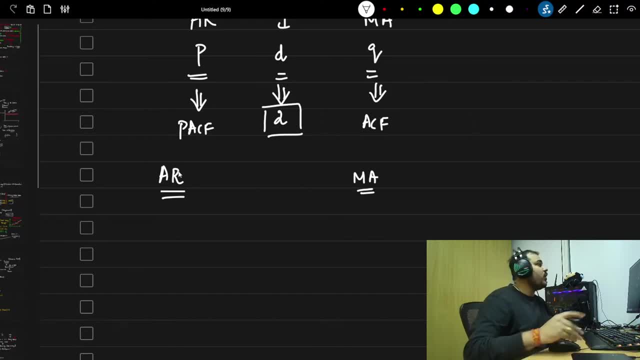 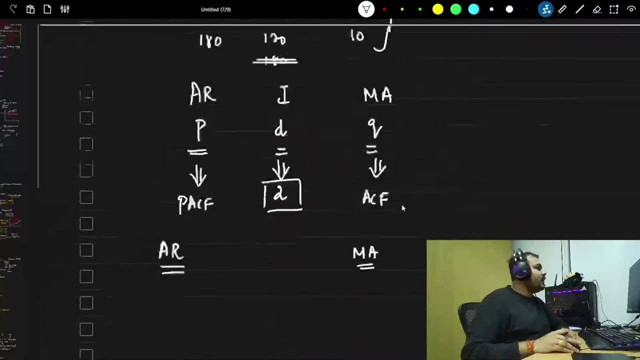 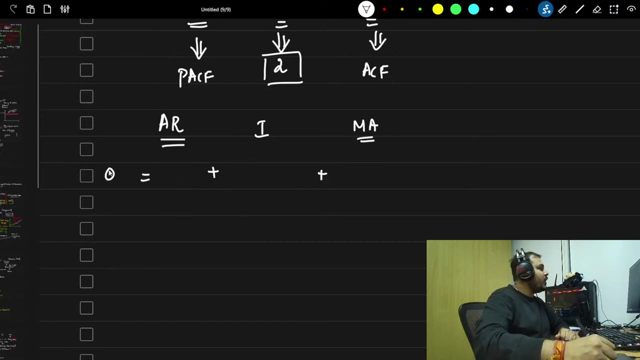 average formula, which I have actually shown you yesterday. autoregressive formula, which I have written right now. see this autoregressive formula, whatever I have defined it over here, and the integrated value Combined everything. It is just going to do the addition and finally you will be getting your output with respect. 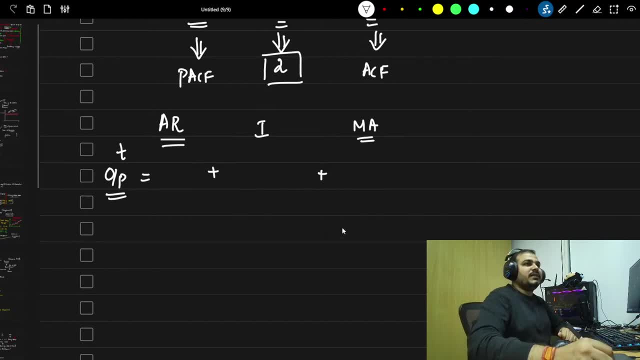 to the current time step. Okay, Guys, why 0.05? Just understand. no, this value can also change, right? We discussed in statistics. usually we use this 5% confidence interval right Now. if you have not attended statistics, that is not my concern, okay. 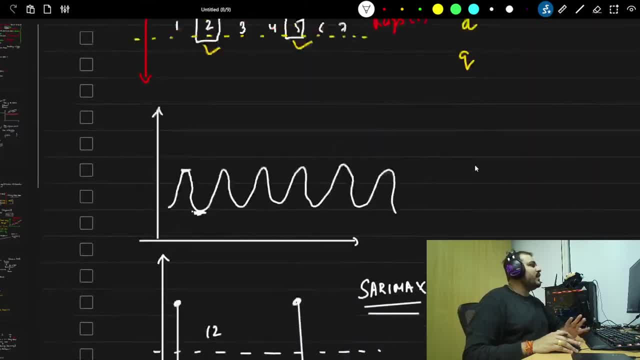 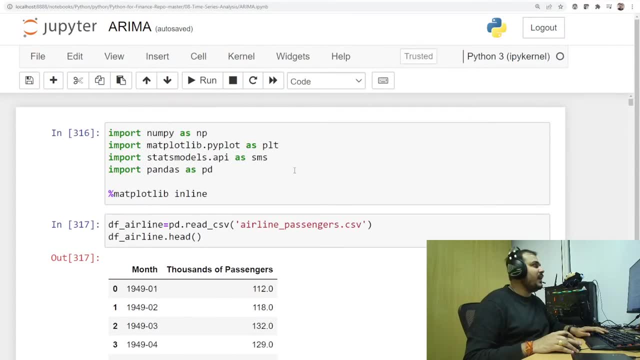 Because I have already taken that. Now let's go ahead and try to implement this entire ARIMA model in a quick way. Okay, So let's see. So, first of all, we will try to do this and we will try to see what all things we can. 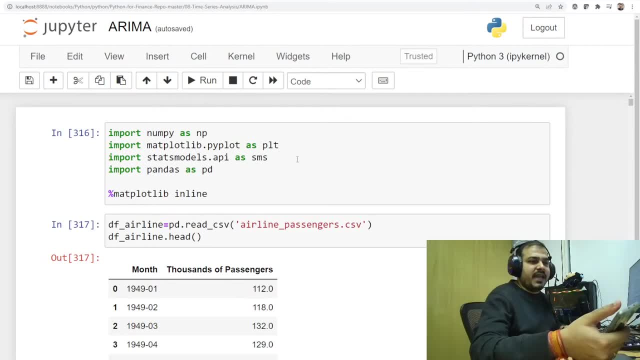 actually what is the data? see, data set can be anything. You can use any kind of data set. but whatever data set I wanted to look for, I don't want it to do that much feature engineering. Okay, Upper bound and lower bound again for that. just imagine, see, how do you find out an? 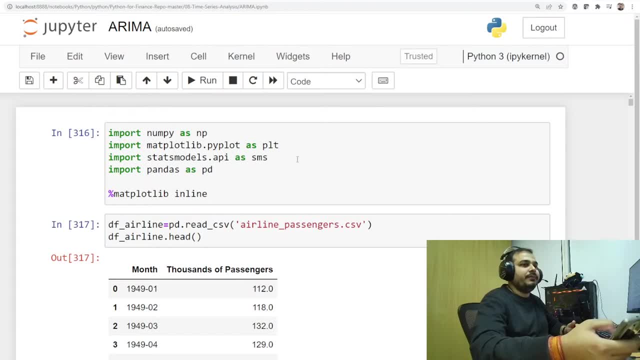 upper bound and lower bound in an outlier. Tell me, We have discussed right Upper and lower bound in outliers. how do we find out? So similar kind of formulas we can apply and we can get the upper and lower bound okay. 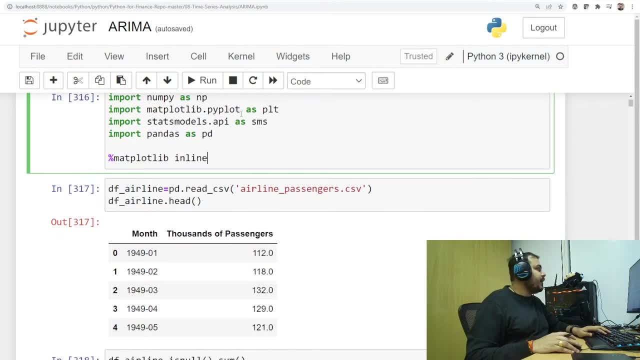 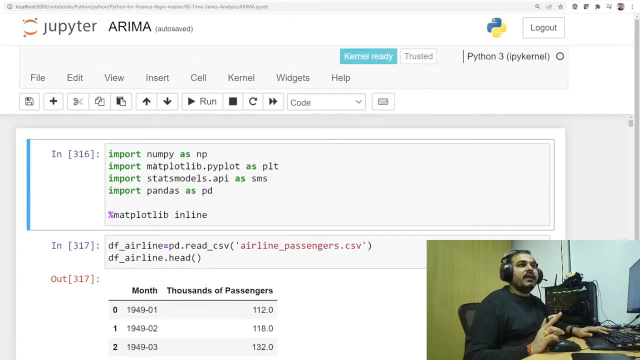 So let's go ahead and execute this. So I'm just going to restart the kernel, okay. So initially I am. I've already given you the entire repository, okay, Based on that, you will be able to see that okay. 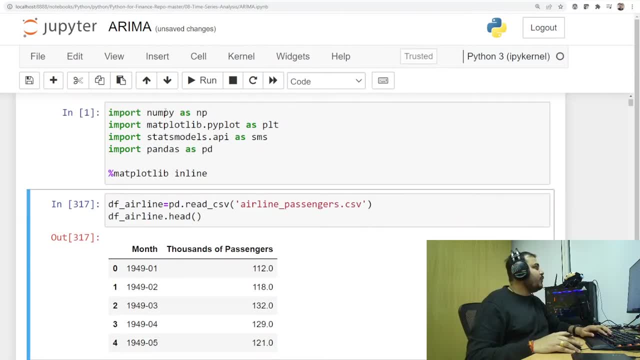 Now let's execute this Initially. I have already given you the entire repository. okay, Based on that, you will be able to see that. okay, Initially, I am importing numpy, matplotlib, statsmodelapi. This will probably have all the necessary things, okay. 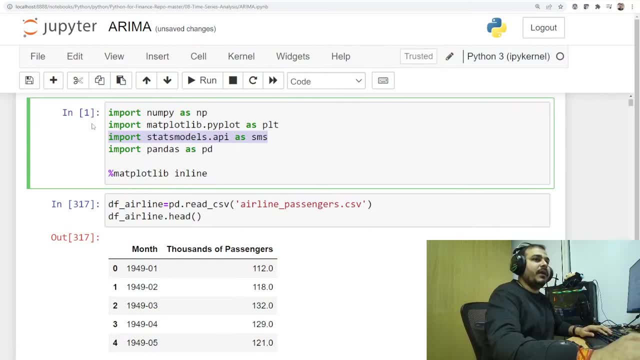 All the necessary libraries that you require in order to implement it. okay, So please check your internet connection. if you are not able to get video quality, good, That is not my problem, because here in my system I am able to get amazing video quality. 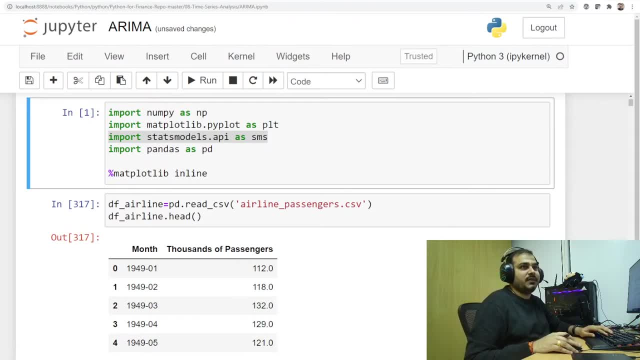 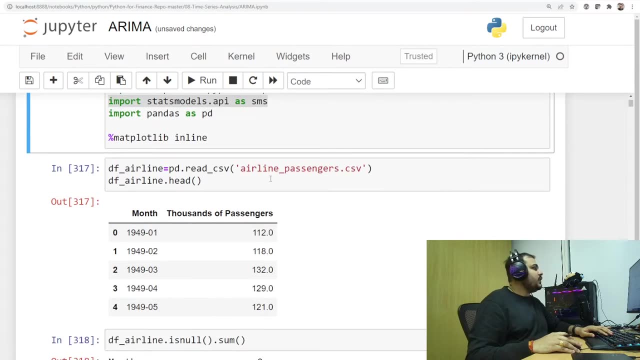 Okay, Please check your internet. Otherwise, use Jio 5G. Okay, Jio is the boon given to the Indians, So utilize that. okay, Now the first thing. first we will try to read the airline passengercsv. So here you can see that I am actually being able to see the data. 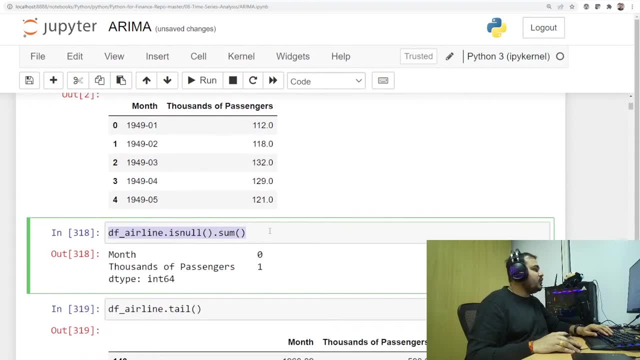 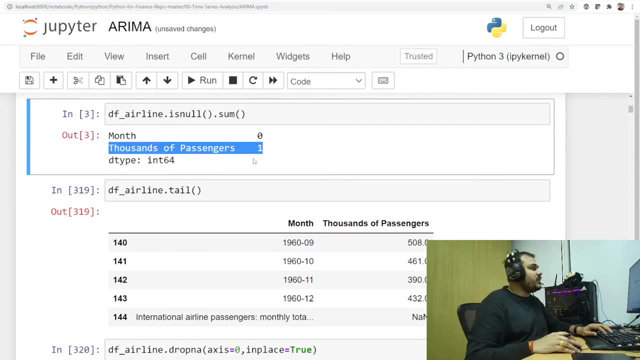 Now, first thing, after this, we are going to check whether there is any null values or not. So I am just going to execute over here with respect to the null values. It shows that, fine, we have one null value, which is which is saying that this, this 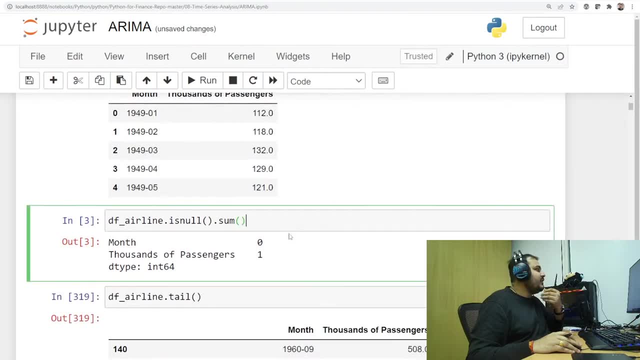 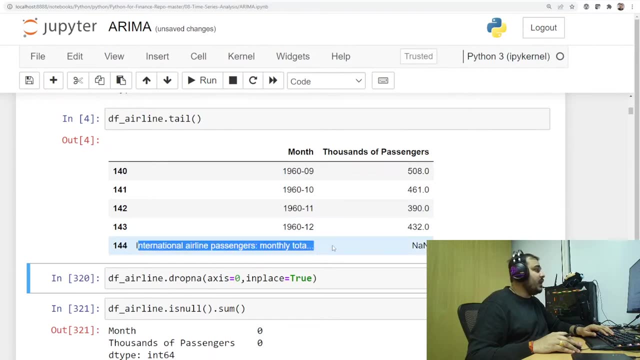 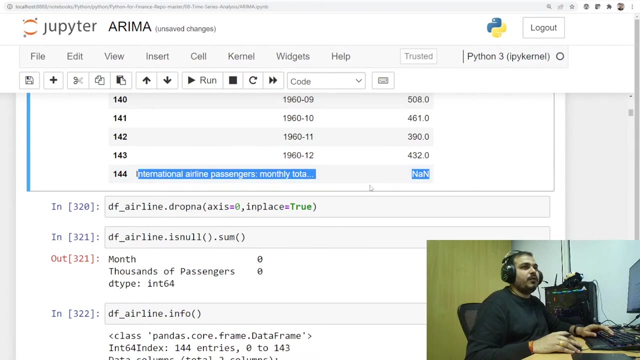 this column has one null values. then what i did is that we, if you go and probably check the tail here, you will be able to see one value which is called as internal international airline passenger, and that value is null. so, just since there is only one row, just try to drop that, because we don't. 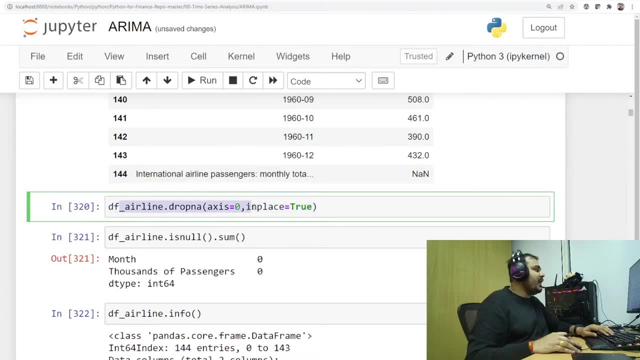 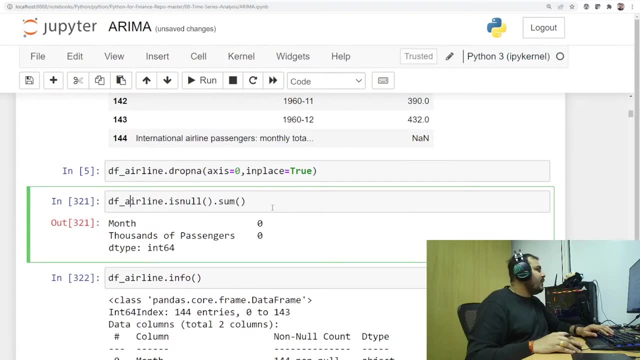 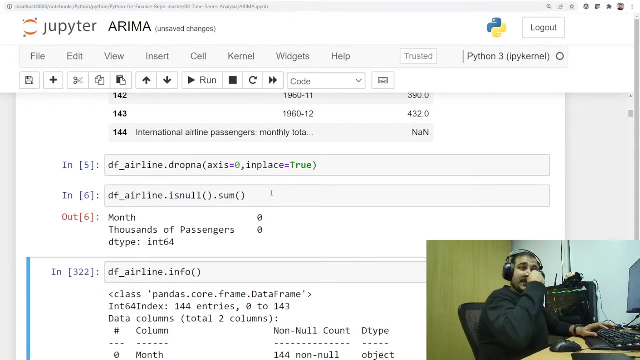 want to replace it. so: df underscore: airline dot. drop na axis is equal to zero in place is equal to true. if we do it, we will be able to see it. okay, then again, i will go and check it out whether we are able to see any kind of some one. everybody clear with respect to this. yes, can i get a quick yes? 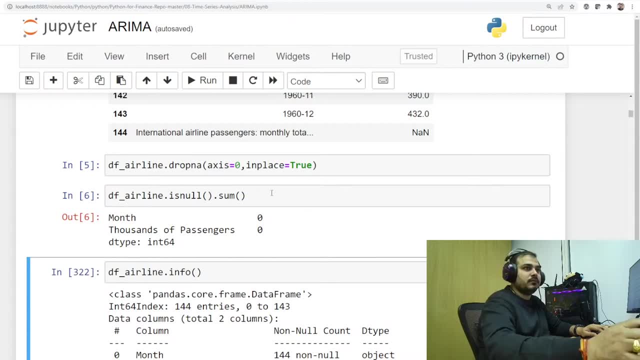 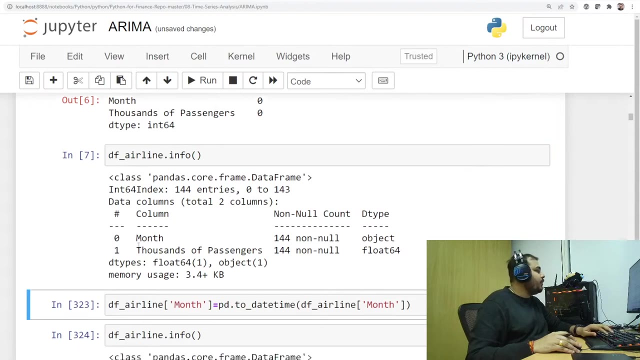 yeah, yes, guys, okay, perfect. so now the next step is that i will just go and check the info here. it says that month is a. okay, perfect. so now the next step is that i will just go and check the info here. it says that month is a. 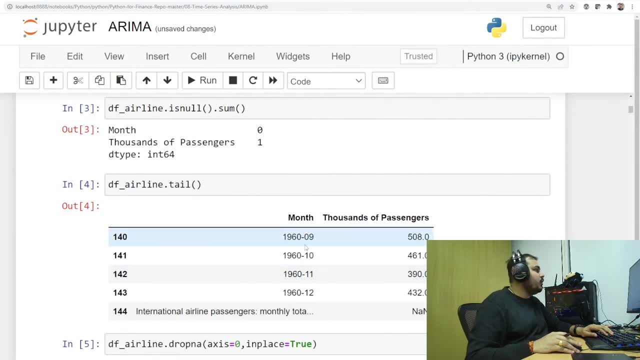 object type. so this is wrong because our month should be a date time type. right because this is what is basically there. our input is basically going to take this and probably calculate the model or try to do the prediction right now. the next step: what we are actually going to do over. 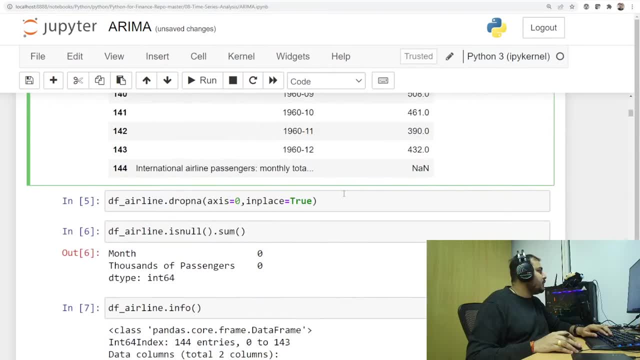 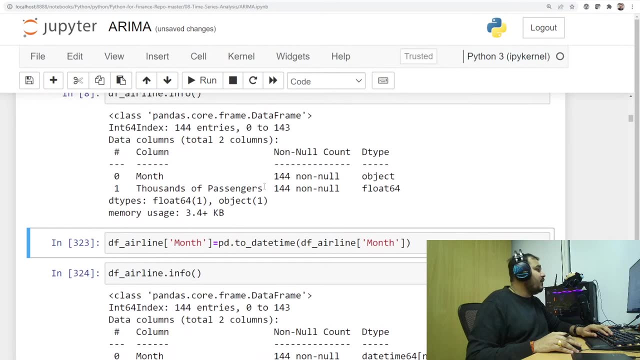 here is that i'm just going to basically say: uh okay, i've dropped it. uh okay, this right now is object okay, object okay. now i'm just going to convert this entire month into date time. how do we do it? pd.2- underscore date time, df- underscore airline of month. now, once we do this, i'm just going to 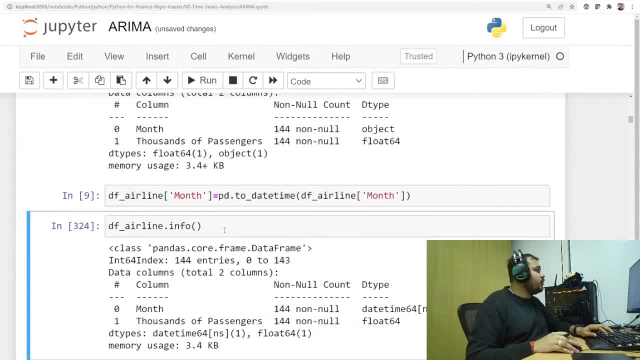 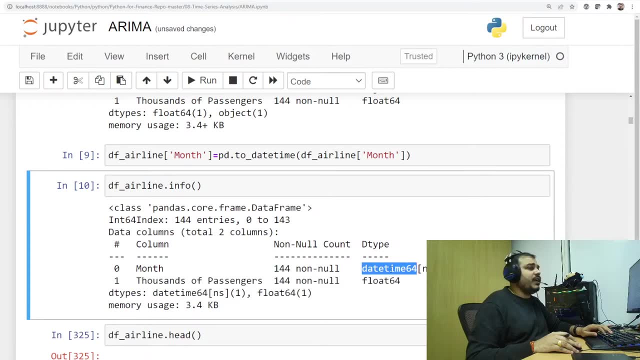 push it in the df underscore airline month column and i'm actually going to get it. similarly, if i go and probably see df underscore airline dot info, i'm actually able to see. now it has got converted into date time. okay, let me do one thing. let me do one thing. 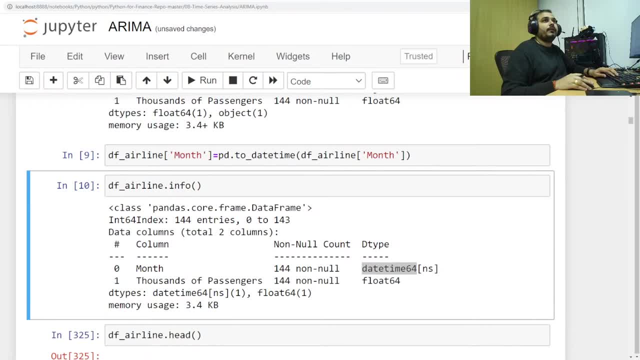 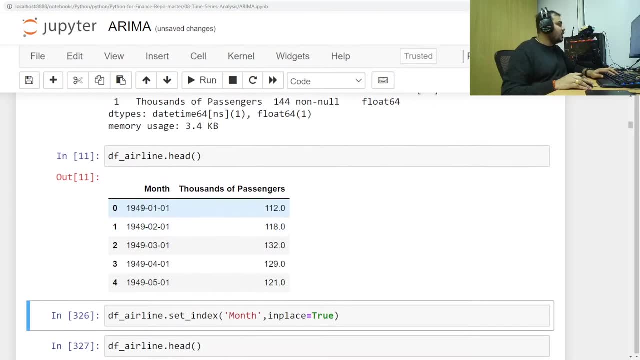 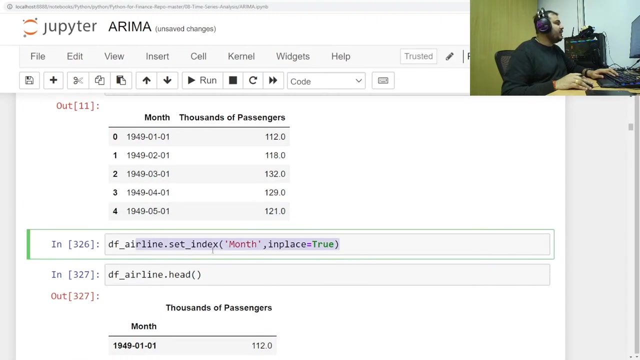 okay, perfect, okay, now i will go and see the head part. now this is now got converted into months and days. you can see over here with respect to the month and then, finally, what we are going to do. we are going to set this month column as an index. okay, this is going to get set as an index, so df. 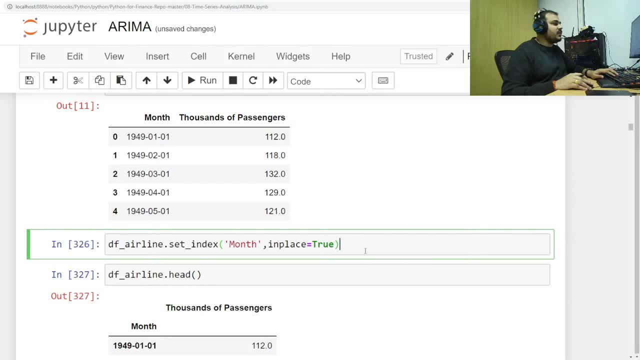 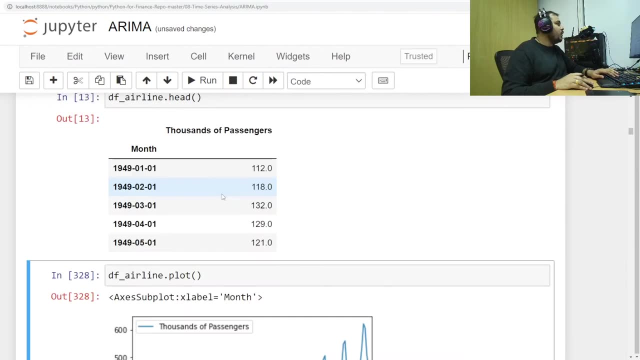 underscore: airline dot set index. month is equal to in place is equal to true. so once we are doing it, this, you will be able to see this. this month column will become an index. so once i go and now see the head part here, you will be able to see that i'm actually able to get the month as my 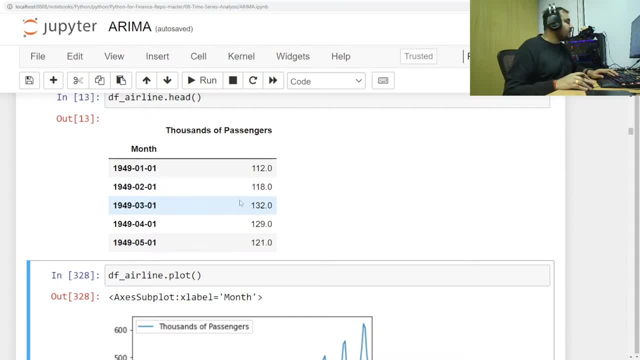 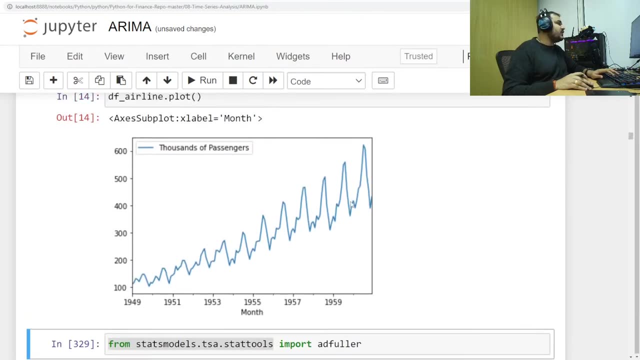 index. so basic, simple things. basic, simple pre-processing that we have focused on. then i'm actually going to just go ahead and plot it now. what does what kind of graph this looks like? is this looks like a seasonal graph or not? so i'm going to plot it now. what does what kind of graph this looks like? is this looks like a seasonal graph or not? 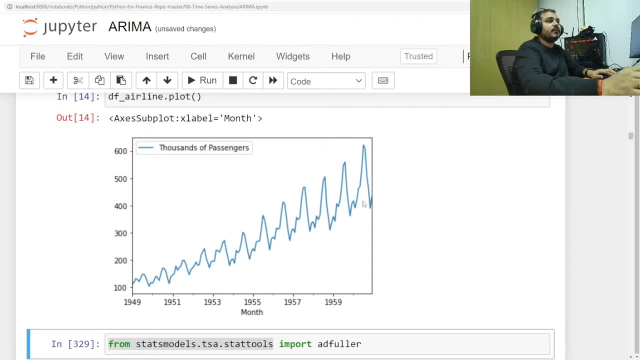 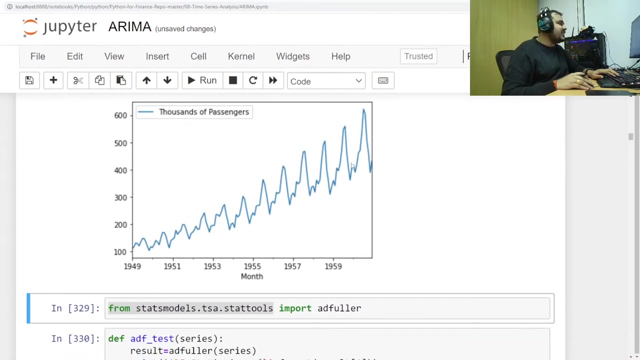 yes, is this a seasonal data or not? yes or no, guys, come on, tell me. is this a seasonal data? yes, obviously it is a seasonal data. here you can basically see that the graphs are moving up and down and, based on that, you can basically find out some kind of trend. okay now, since this is a seasonal data, now see what will happen, okay. 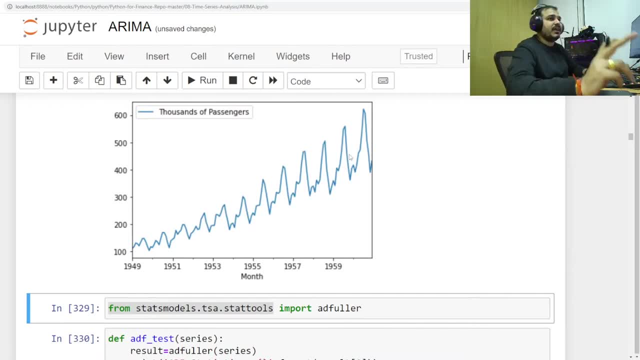 if this is a seasonal data, it cannot be a stationary data. understand that our data set should not be seasonal because, see over here, everything is increasing. it is not stationary, okay, so what we are going to do is that we are going to basically use dickey fuller test, which is imported. 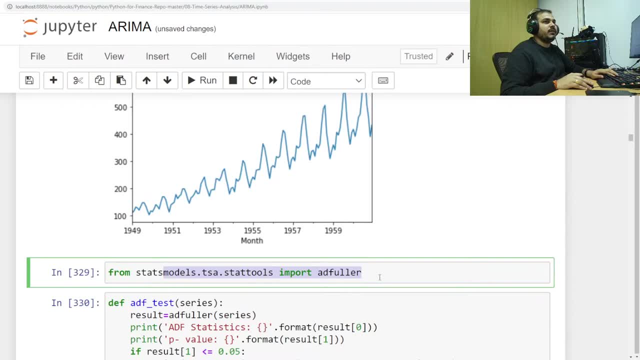 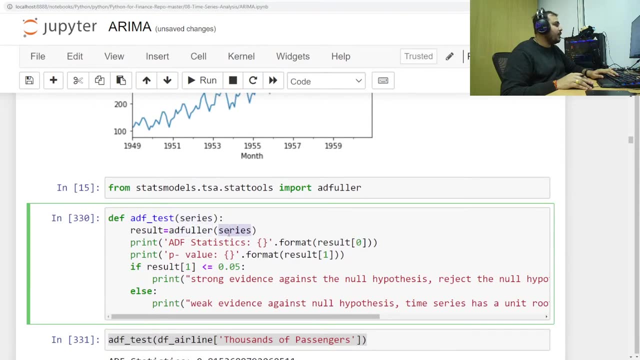 from this library, which is called a stat models, dot, tsa dot, stats tool. okay, import, add fuller. now inside this what i am actually going. i'm using this ad fuller whatever data set is coming over. here i am getting two values. one is adf statistics and 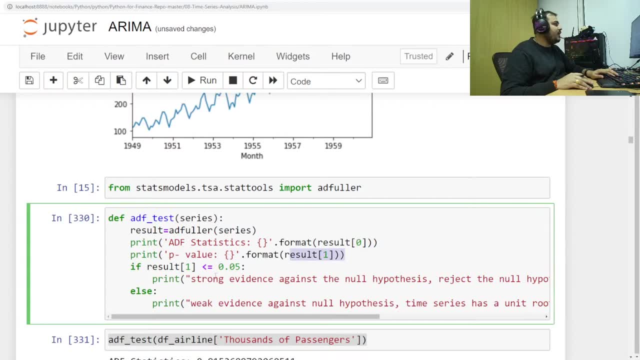 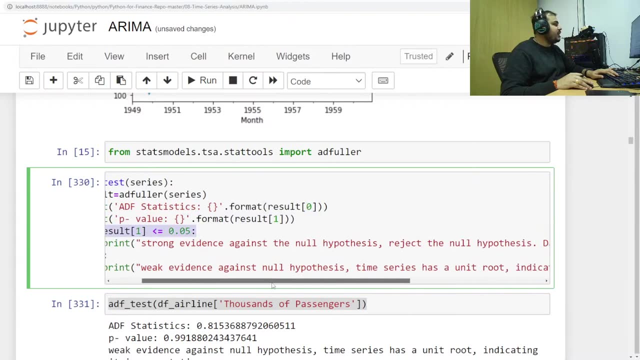 one is p-value And this p-value from result of one. I will be able to see it. I am just saying that if the p-value is less than or equal to 0.05, I am actually saying that strong evidence against the null hypothesis rejects the null hypothesis. The data has no unit. 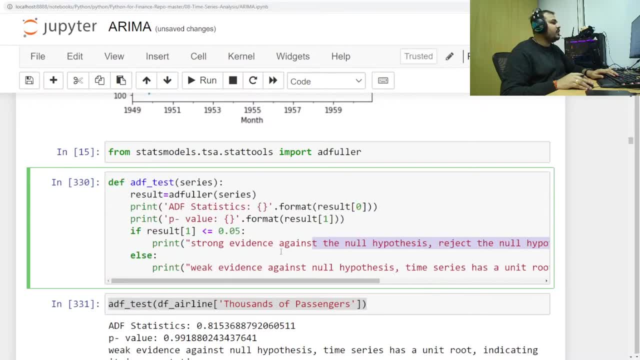 root and is stationary. So, in short, we are just rejecting the null hypothesis And we are saying that: okay. we are saying that: okay, fine, the data is stationary If this value is greater than 0.05, then we are basically saying weak evidence against null hypothesis. 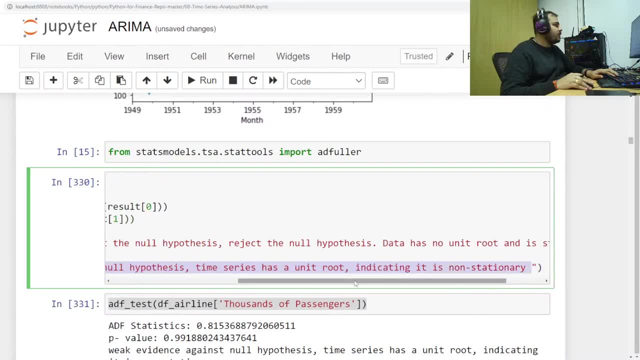 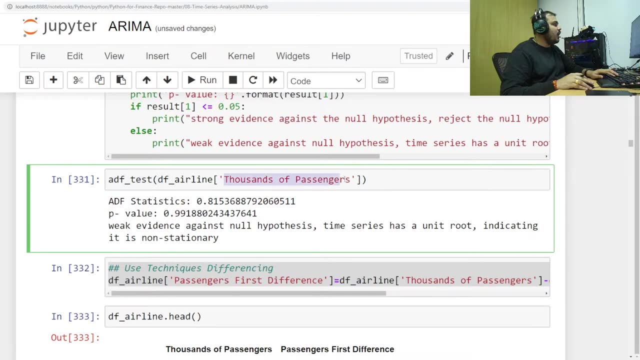 indicating it is non-stationary. Okay, So these two things. I am creating a function with respect to this. Now, what we are going to do, add underscore test. I am just going to give my column, that is, thousand of passengers, which is the current column over here, And 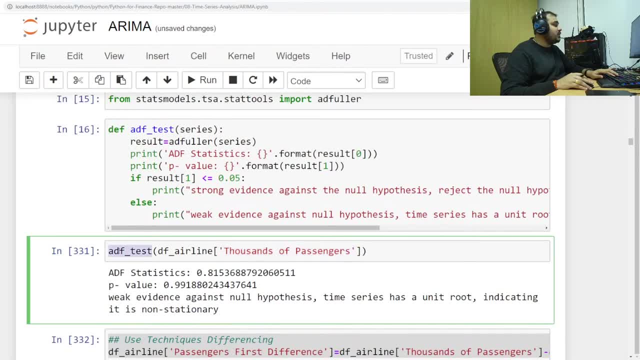 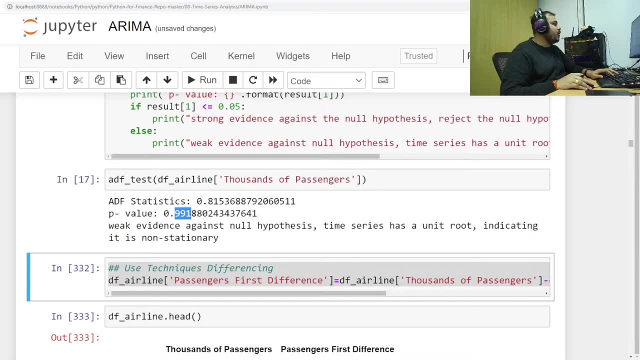 we are just passing it to this df underscore airline, I mean to this function which is called as adf underscore test. Now, once I calculate it, you can see that my p-value is coming as 0.05.. So definitely the else block will get executed And it is indicating that the data is not stationary. 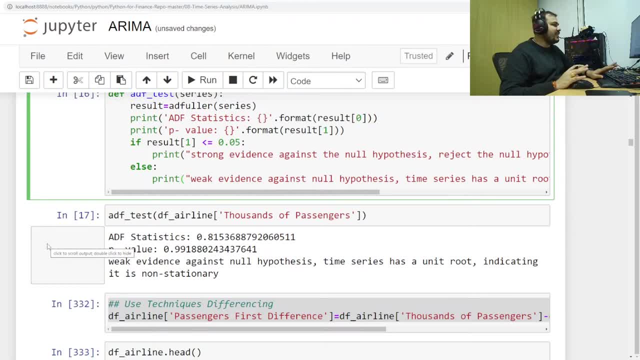 And obviously the data is not stationary. So you can basically think over it that, yes, the data is not stationary at all. Okay, This is done. Perfect, Till here, you are absolutely fine. You have executed this Now in order to make it stationary. we will start doing. 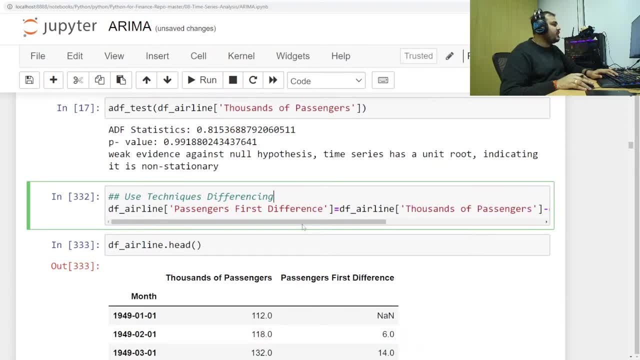 differences differencing. Now, in differencing, what we do is that we are just saying that passenger first, difference. Okay, So we will just use dot shift of one. One position will be shifting because we are just doing differencing by one day. Okay, So df of airline of thousand passengers minus. 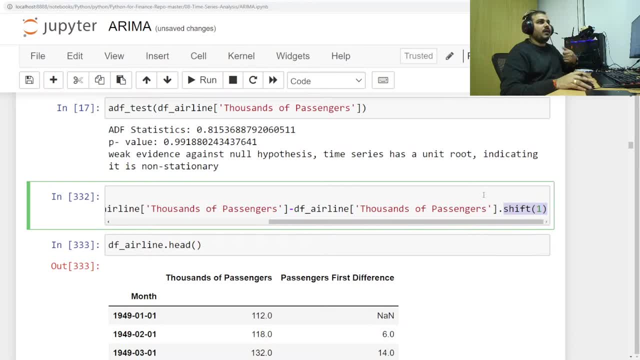 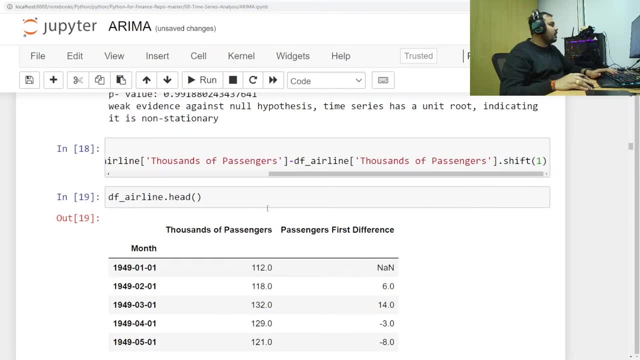 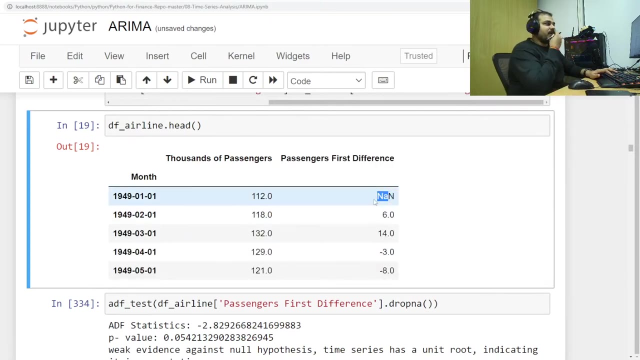 df of airline thousand passengers dot shift of one Then it will get just shifted by one position. Okay. So if I try to execute this and see now df of airline dot head, you will be able to see passenger first difference: The first value is NAN. Okay, The first value. 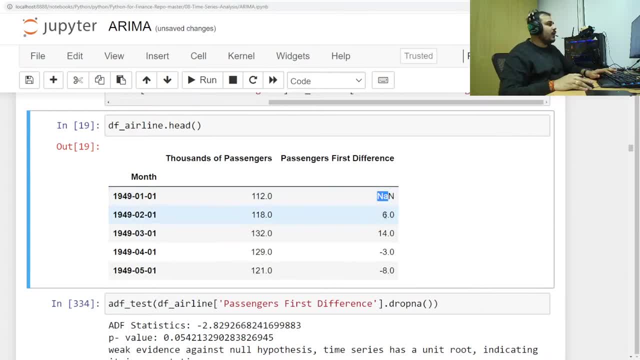 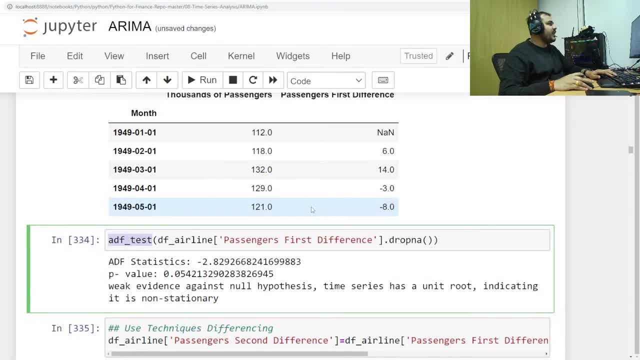 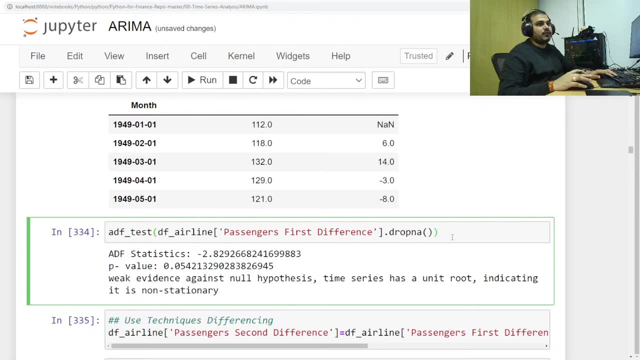 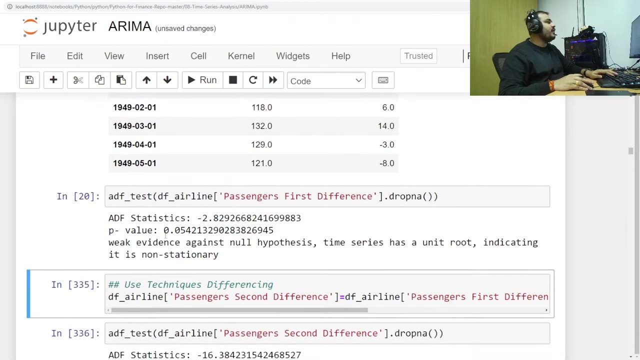 going to do over here is that I'm again going to give this ADF test and I'm going to pass now my first difference column and try to check whether I'm actually getting any kind of values or not. Okay, So over here, if I'm executing it here, you can see my p-value is 0.054.. Again. 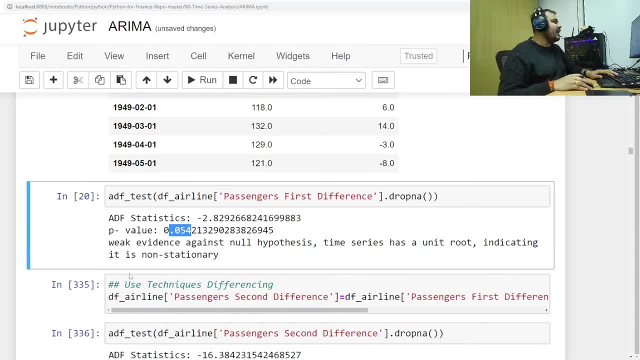 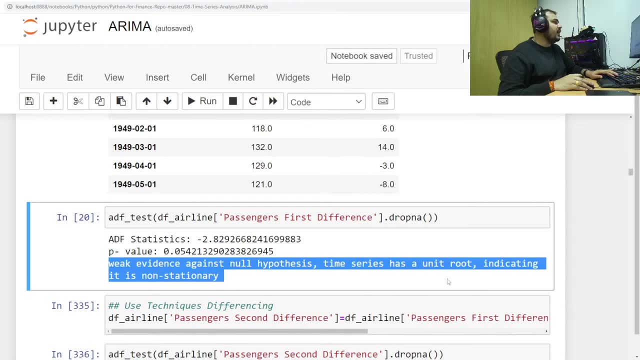 the null hypothesis will get rejected and it will indicate that it is not stationary. Okay, So weak evidence against null hypothesis: time series as a unit root, indicating it is non-stationary. Okay, We have to make it stationary because the p-value is 0.054.. 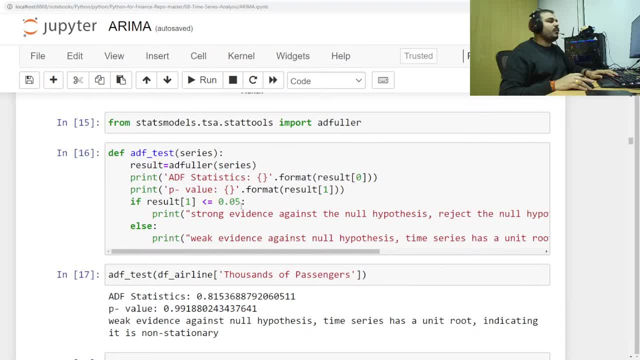 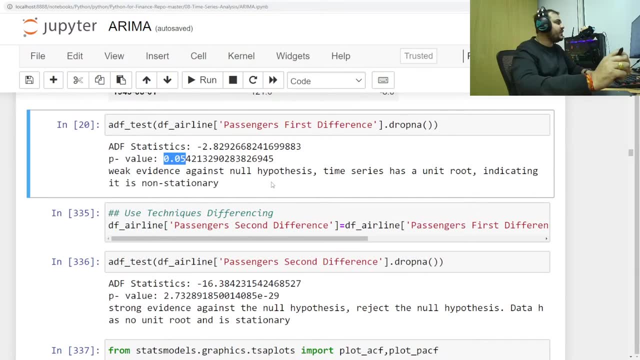 But here the condition that I've actually written it is less than or equal to 0.05.. Okay, So this part is done, Right. Everybody clear till here. With respect to differencing, the first differencing Now currently, if I'm not able to get it right now, so what I'm actually going to do Again. 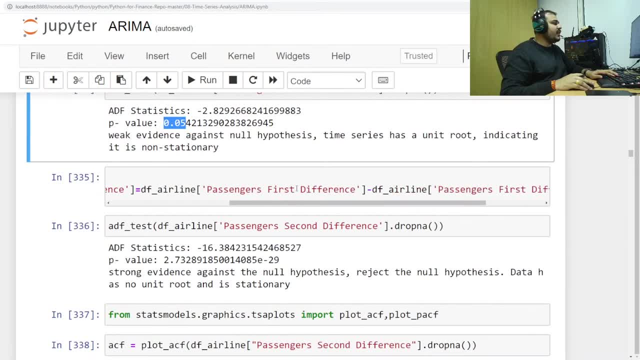 I'm going to do the second differencing. Now, second differencing, I'm going to take this column, that is first difference, Okay, And then I'm actually going to do first difference: dot shift of 1.. Okay, Now, this will basically give me my second differencing, And if I probably try, 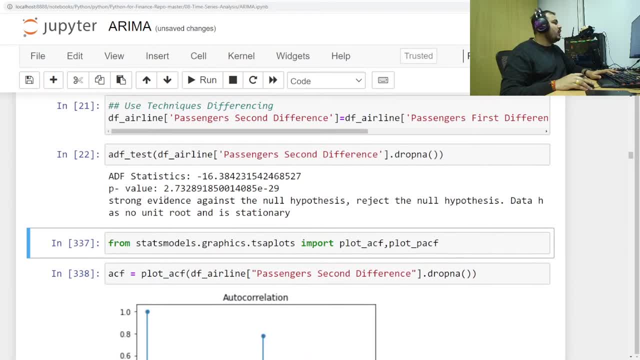 to execute this and pass it to my ADF test. it is now giving 2.73 multiplied by 10, raised to minus 29.. So that basically gives me 2.73 multiplied by 10 raised to minus 29.. So that: 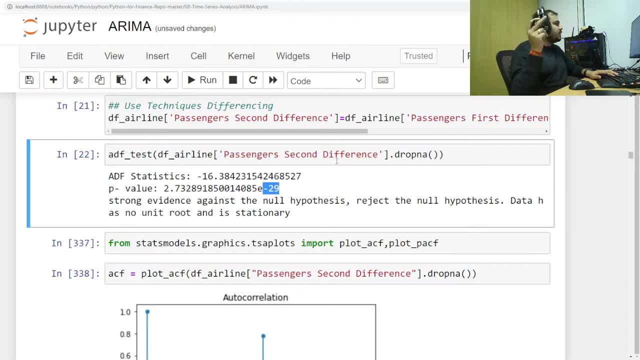 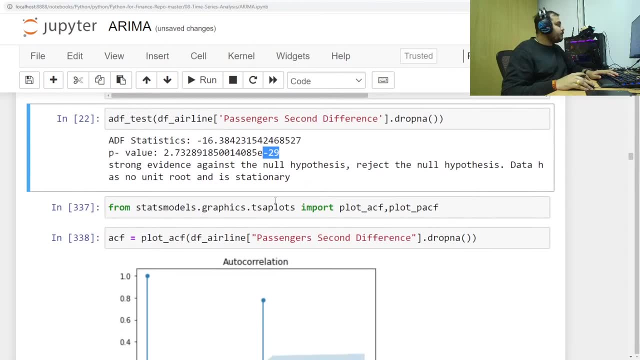 basically is 0.0000000000273, like 29 times 273.. Okay, Now, with respect to this, now you can see that we are rejecting the null hypothesis and we are saying that data has no unit root and is stationary. Okay, This is fine. That basically means we have now got off my d-value as 2.. 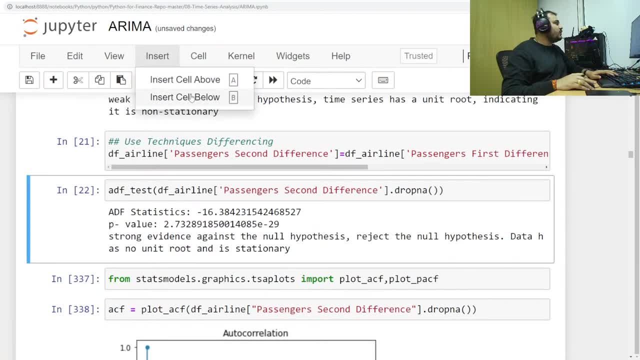 But I can understand one more thing, guys, If you probably want to. you know that this is a season. You know that this is a season. You know that this is a season. You know that this is a seasonal data. Right, Everybody knows that this is a seasonal data. Now, in seasonal data, we should. 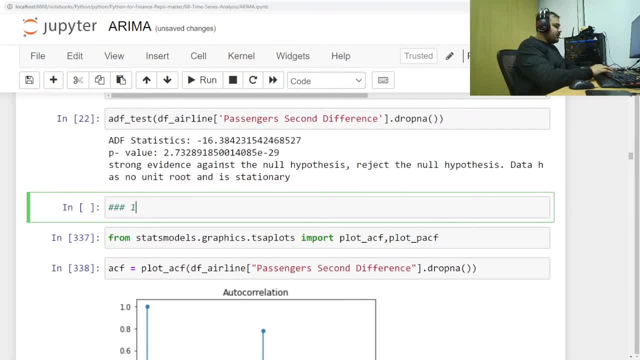 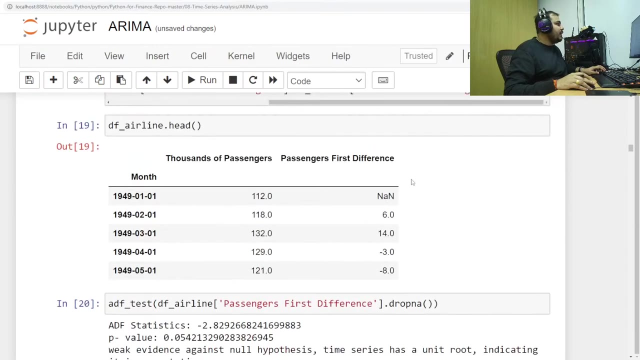 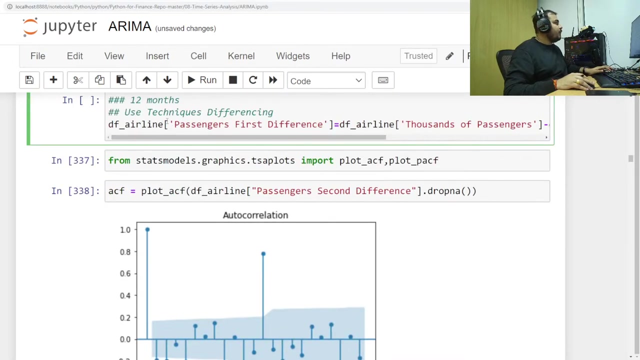 also be making sure that we do 12 months Because in seasonal data, since it is for the year where you have got up and down, Okay, With respect to that, what we are going to do, we are also going to do it for 12 times Okay. So, if I probably take this up, that is 1000 passenger. Okay, I'm. 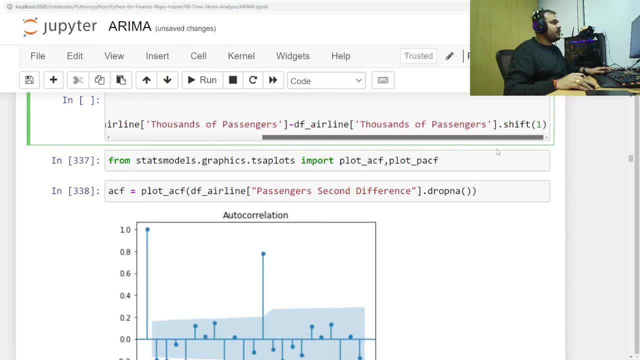 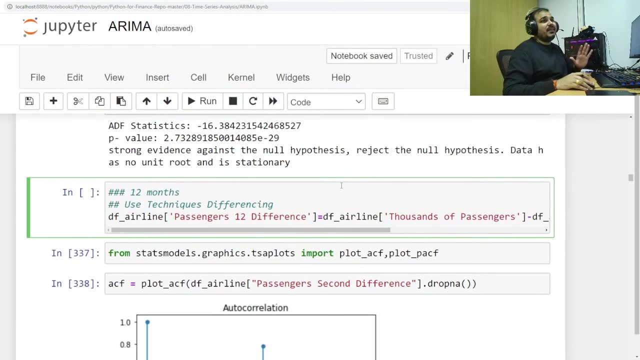 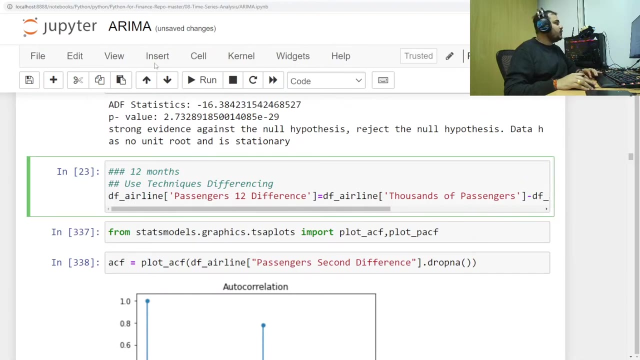 going to basically say passenger 12 difference, This is for seasonal Right And then, if I do, shift of 12. That basically means we are doing it for the entire year, Because seasonal data will also have that kind of examples to see whether the data is stationary or not. So here I have. 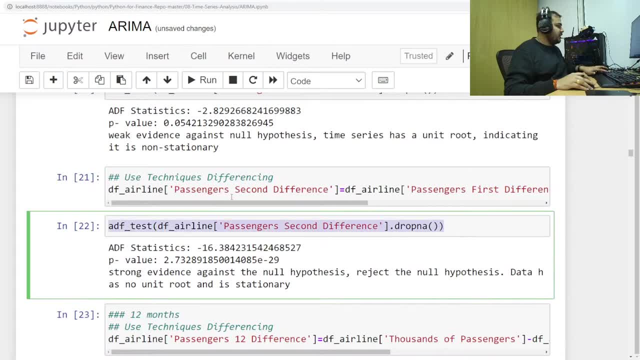 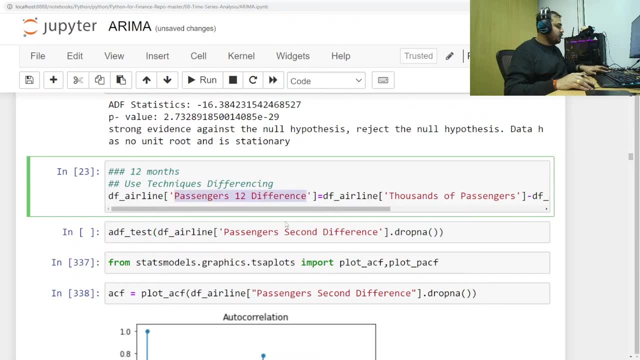 executed it. So what I am actually going to do now, I am going to just pass it towards this ADF And I am going to basically say that this column that I have passenger 12 difference, I am going to pass it over here. So if I execute it here, you will be able to see that strong. 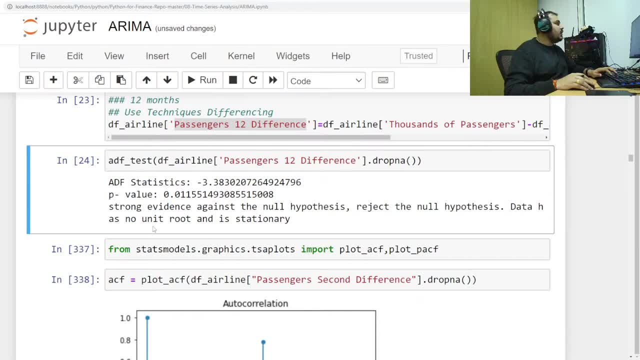 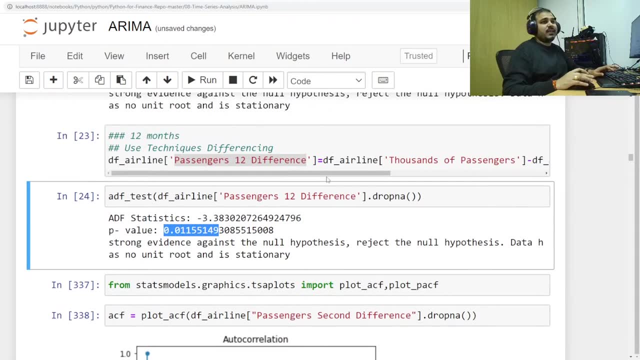 evidence against the null hypothesis: reject the null hypothesis. data has a no unit root and is stationary. Now, since I have got 0.01, that basically means yes, seasonal difference, that is, also. we can basically apply within one difference only. we are able to see that. 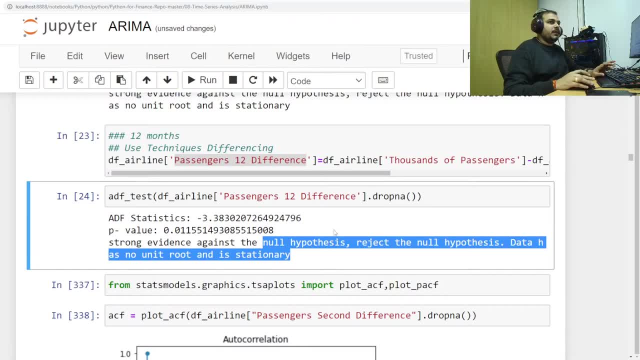 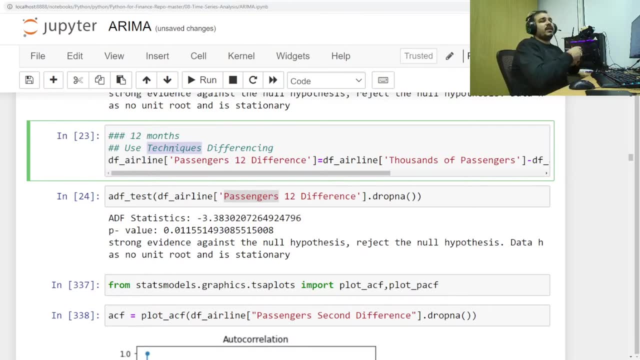 we are able to get it stationary right. So I hope you have understood why we have done this seasonal difference. also because for seasonal, you know, sometime ARIMA will not work well, SARIMAX may work well, okay. So that is the reason. Then now let's go and select our 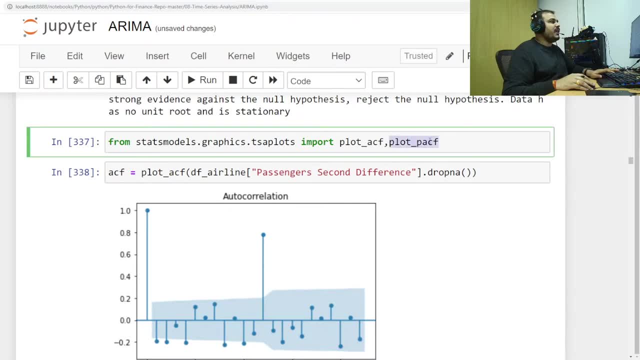 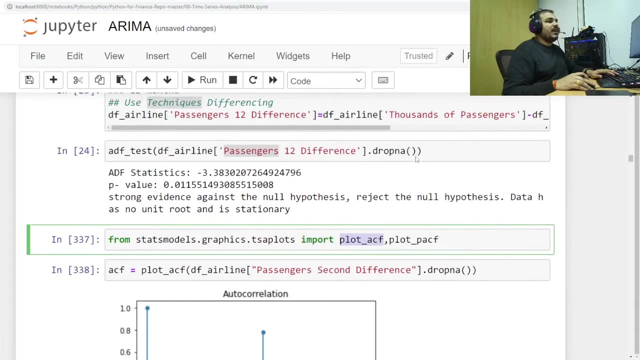 P and Q value. P value is basically determined by PACF. We have to plot a PACF and ACF is nothing but autocorrelation plot, okay, It is not. which is better. guys understand Commonly. we have to plot a PACF and ACF is nothing but autocorrelation plot, okay. 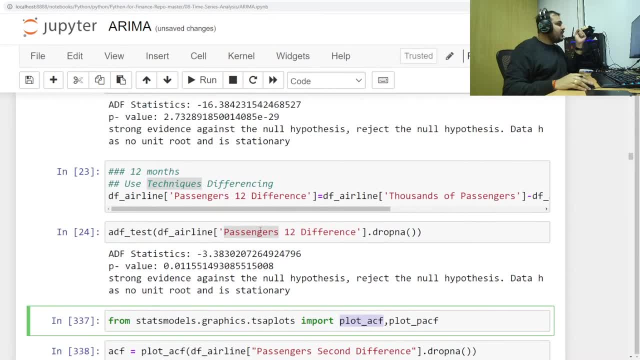 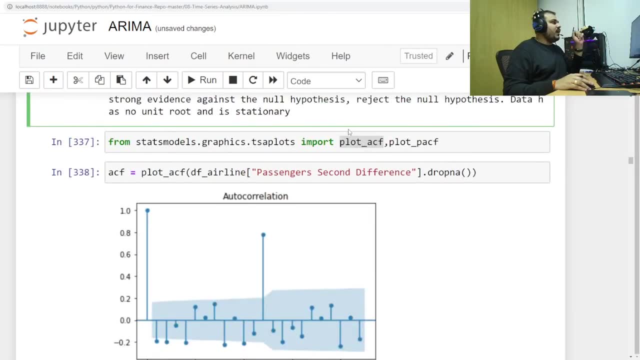 If you have a seasonal data, you should definitely go with this kind of 12 months difference. okay, Here you will be able to understand. see what will happen if I probably give plot underscore ACF. okay, Suppose if I try to plot it with respect to: 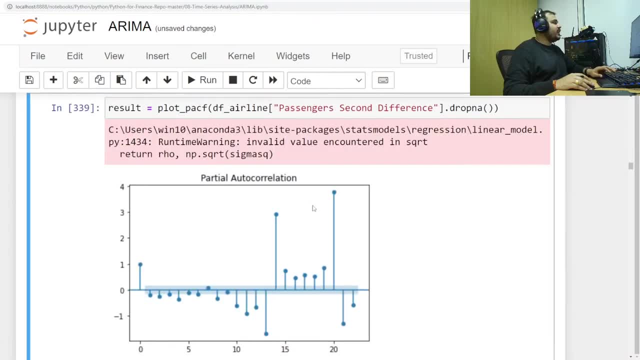 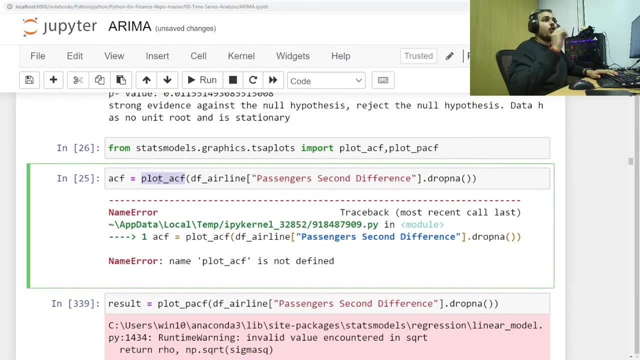 second difference: okay, Second difference, So I am just going to execute it. So, okay, I have not executed this. okay, fine, So now see if I am plotting an autocorrelation plot with the help of this particular column, that is, passenger. second difference: because we have 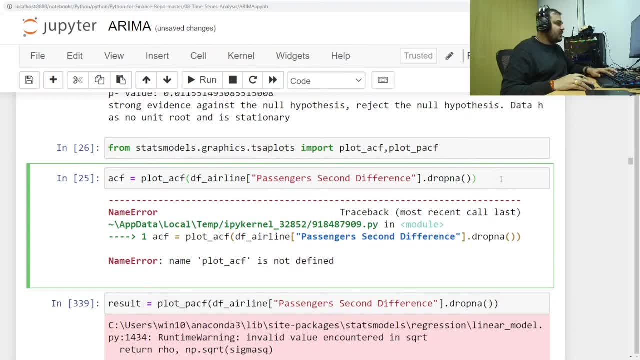 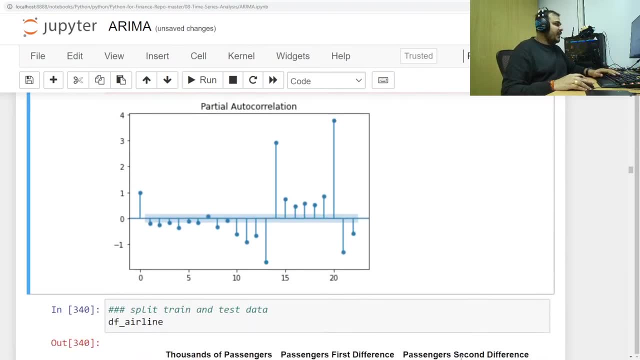 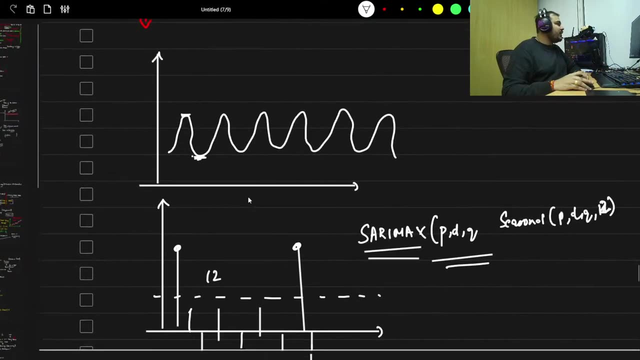 to provide our stationary data dot drop NA. then you can see that I am getting this kind of graph. Now this graph. what does this graph basically say? Tell me guys, Here you can see that. right, I have drawn this graph. I have drawn this graph. okay, with respect to ACF. 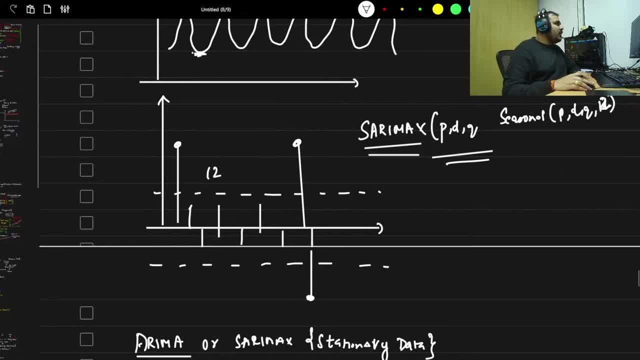 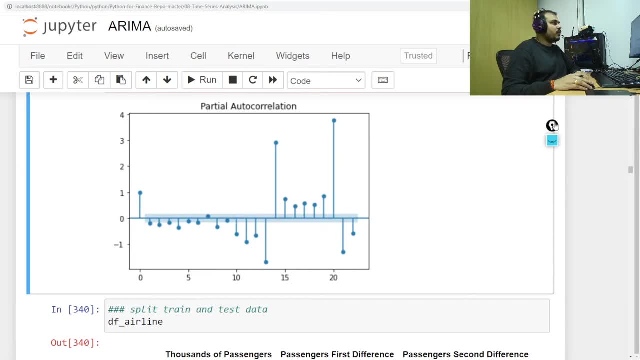 something like this. It is similar like this: only right, You can see over here, here is my borderline. Everybody, focus over here. See this, everybody. I will show you. I will show you over here Now which I was actually talking about. 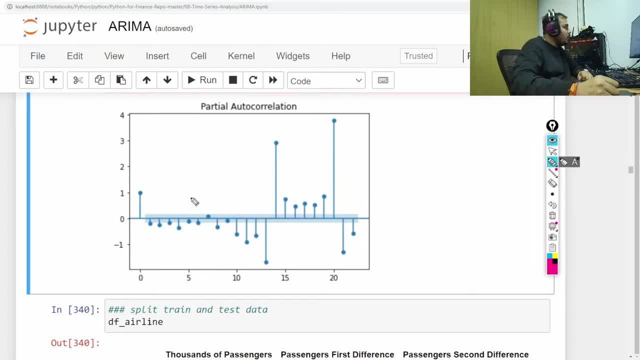 what is this line? Can anybody tell me What is this line? What is this line? What is this line? Come on, tell me. That is nothing but your upper bound and lower bound. okay, Upper bound and lower bound, I told. 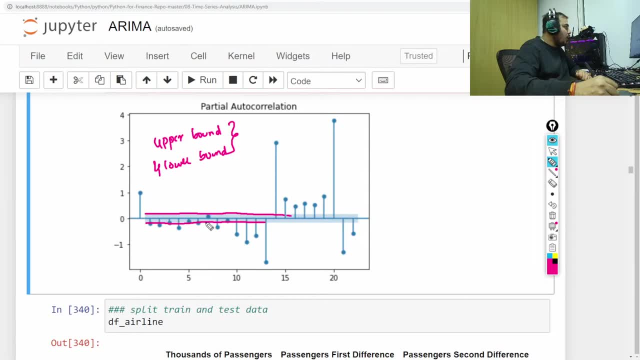 you right Any lines that is going above this upper bound or above this lower bound, then what happens? It says that it is having a direct impact, That from here it is basically starting from t0.. Then we have t1, t2, t3, t4, t5, t6, t7, t8, t9, like this. So usually in seasonal 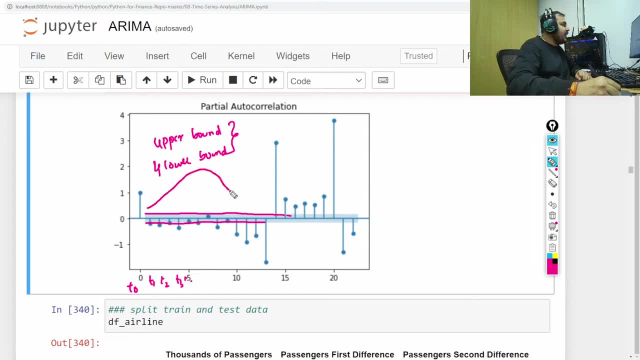 data. you will be seeing that. suppose my graph looks like this, right With respect to seasonal data, Let's say it is looking like this. it is looking like this right Now, in this particular case. you can see that over here, hardly any correlation you will be able to find out, But 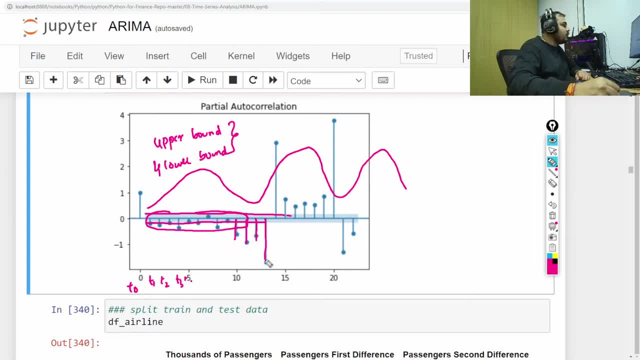 from here you will be able to see the lines are going up, And here also you can see the lines are going up. So for this we can definitely use seasonal type also. okay, Now, if probably you are saying me: okay, Krish, try to find out my p-value by using this diagram, then how do you? 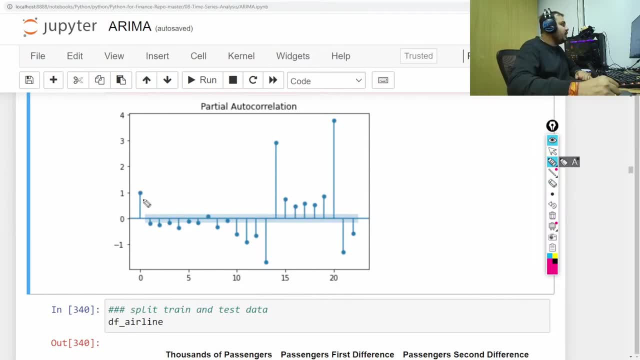 find out your p-value. You just try to calculate. okay, From here to here, I can probably see the first line that is going below this itself. right, This is a partial autocorrelation, right? So let me just show you once again. okay, Now see, here we are plotting. 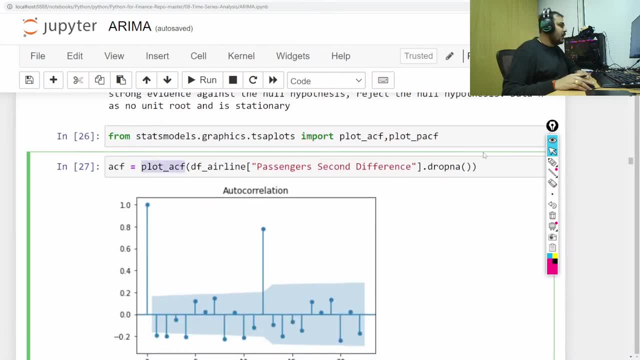 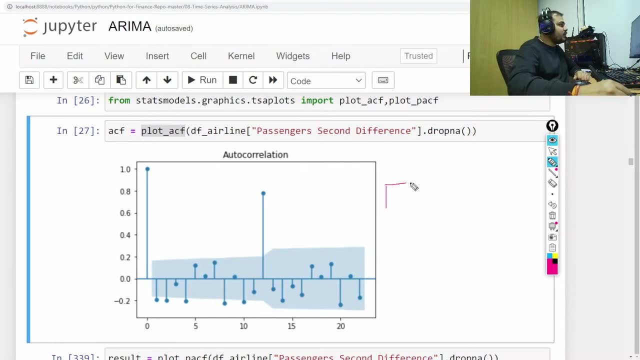 first, let's start with autocorrelation plot. okay, Now in autocorrelation plot, let's see this. What did I say with respect to autocorrelation plot? I told you that suppose this is January, suppose this is March, and there is also February In autocorrelation plot. they will suppose this is. 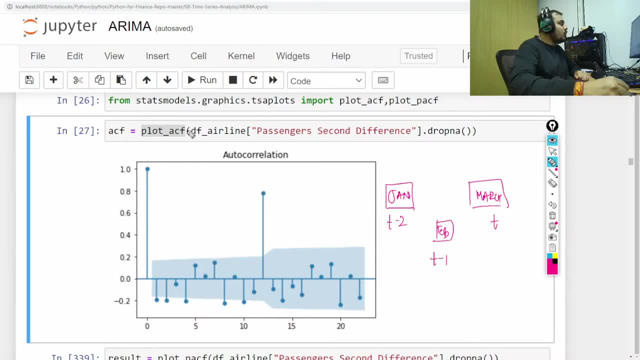 time. this is t minus one. this is t minus two In autocorrelation plot. that is ACF, right. There are two things. First of all, we try to see how January is correlated with February, how February is correlated with January, and one more indirect, how January correlated with 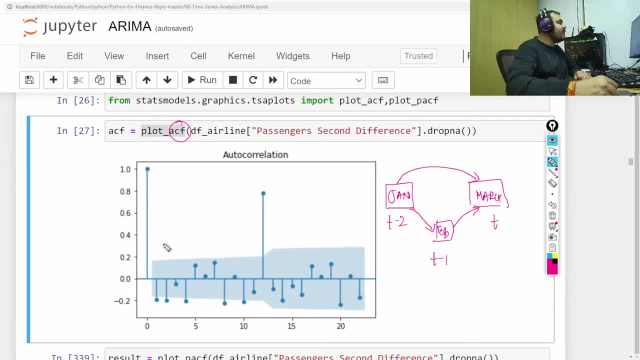 February. So all this information will basically get combined, and here also you use Pearson correlation. Pearson correlation, okay, Pearson correlation. We basically combine, combine this. let's say: this is my x, this is my y, this is my z. okay, Now what we are basically. 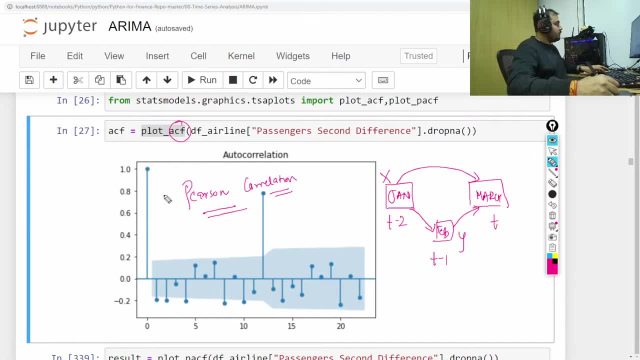 going to do. We may have data, see, we may have data with respect to x, y, z, like this, and this data will be basically present. So probably I may say that, something like this: okay, This, this data is with respect to January, February, okay. 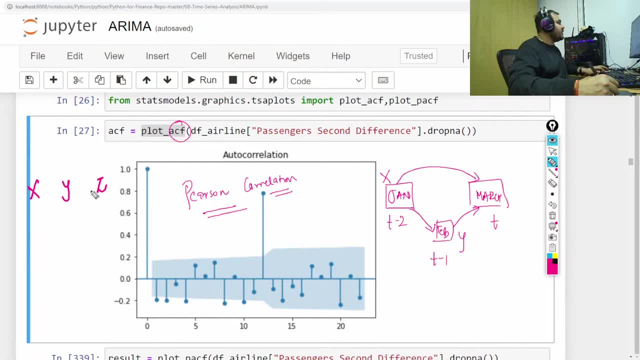 Or let me make like this: okay, Let me say that: okay, this is my x y z. I know what is my x month. My x month is Jan, my z month is March and this month is Feb. 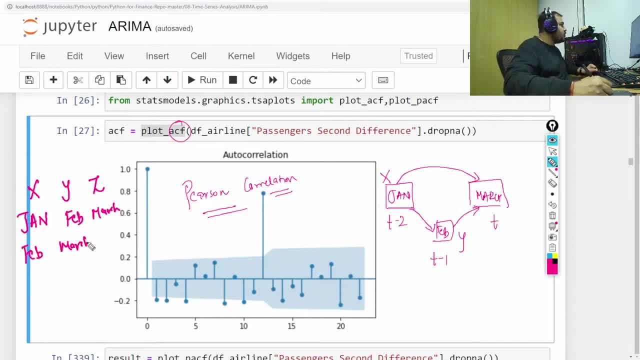 Then next what I'll do. I will make this as Feb, March, April, So I'll have this specific data, March, April, May. I'll take all this data and try to find out the correlation between x to y, y to z and x to z And overall. 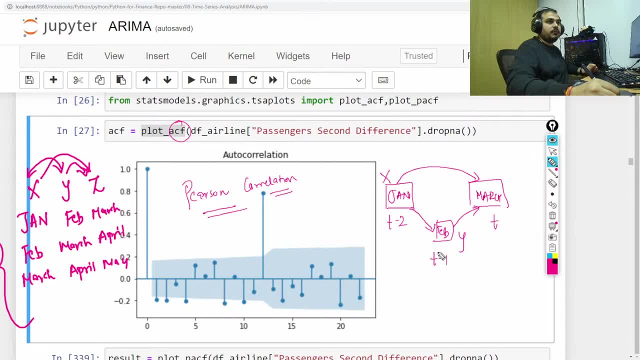 we'll try to combine and we'll try to create something like this. okay, so, in short, acf, we are going to see whether there is a direct impact, whether there is an indirect impact, and everything will get plotted in this specific way. okay, one property. you can see that as we are. 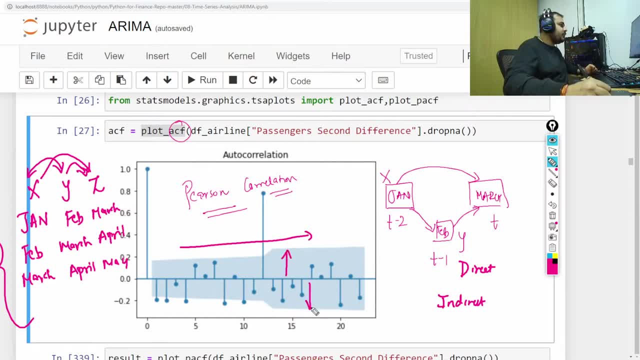 going like this. right, you can see that this band is increasing. right, this band is also increasing. that basically means this error part is also increasing. okay, now, how do i find out what should be my see, with the help of acf, we find out a parameter that is q. okay now, with the help of, 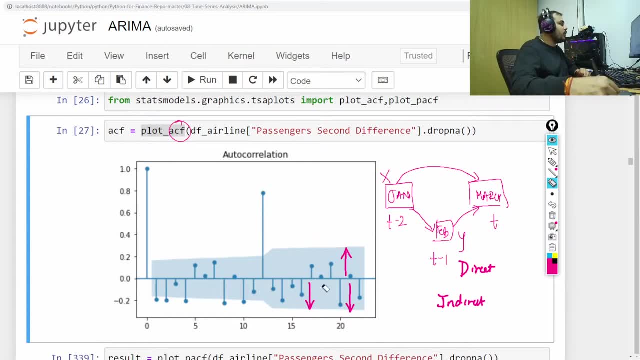 this: how do i find out what is the parameter q? what is the parameter q? so i will just go and calculate with respect to the data points that i see. the first data point over here, this is for 0. 1 is also passing this lower bound. 2 is also passing this lower bound. this has no impact. 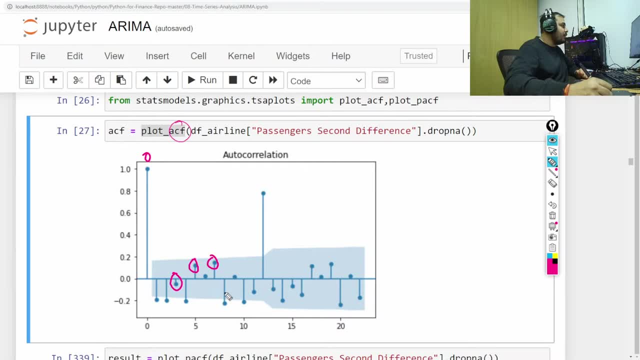 this is passing through the lower bound. this has no impact. this has no impact. this is passing towards the lower bound Over here. you can see that the maximum it is passing from here. So I will just go and count: 1,, 2,, 3,, 4,, 5,, 6,, 7,, 8,, 9,, 10,, 11,, 12,, 13.. 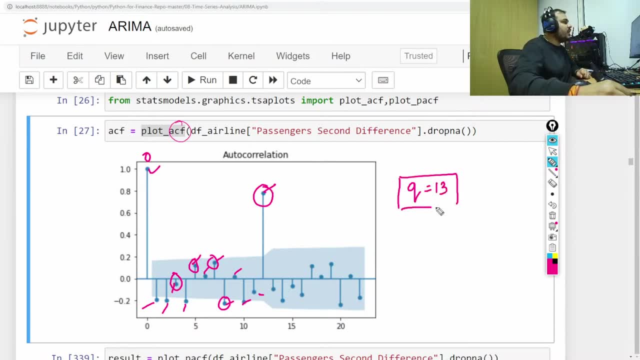 So I may say that my Q value will be 13, because I really want to see this impact. that is there, Okay, But since this is from 1 to 13,, you can see that there is some kind of seasonality. So what I will do is that now I will try to plot this. 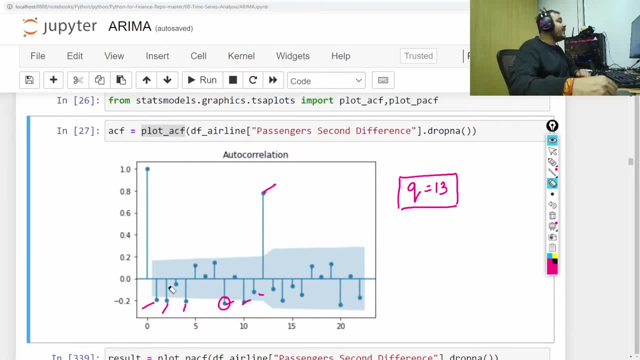 plot underscore ACF with respect to the 12 differencing that we have done, So that we'll see that, whether there is anything with respect to that also. So what I am actually going to do, I am just going to plot this, I am just going to basically. 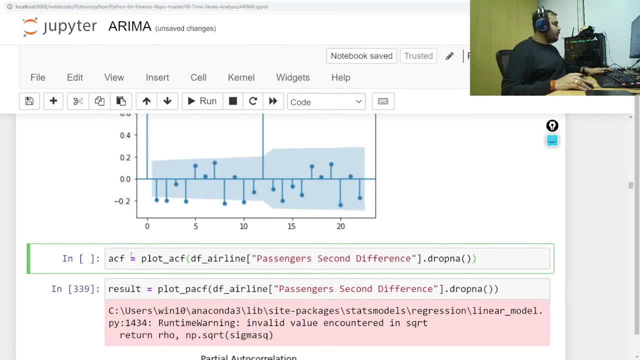 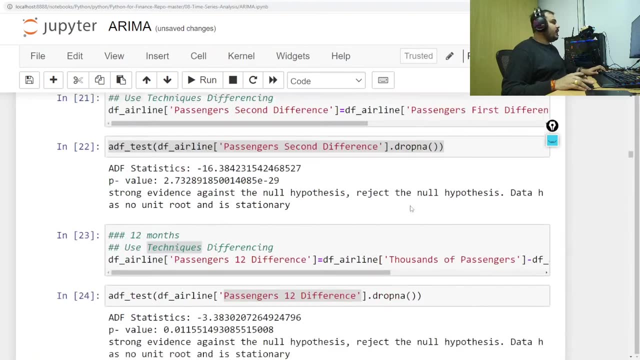 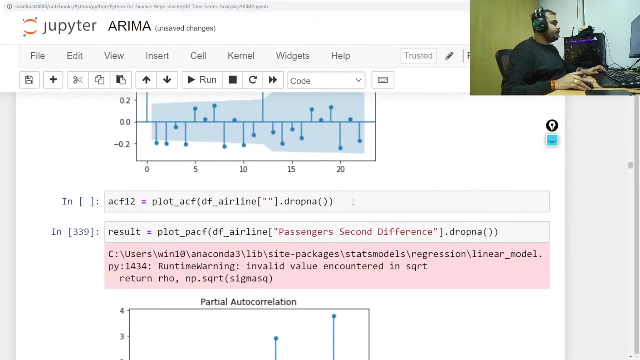 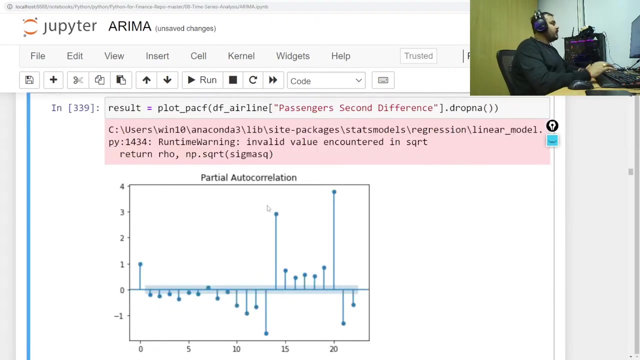 insert cell below I am going to say ACF 12.. ACF 12. and here I am going to basically say what is the column name that I created: Passenger 12 difference. Passenger 12 difference. Now, if I try to plot this and if I try to see, are you? 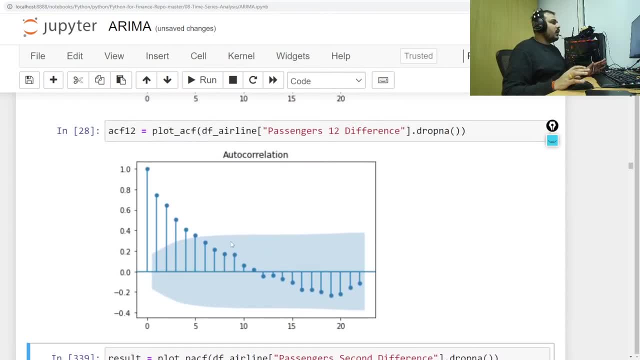 able to see some amazing thing over here. Now, what is happening over here? Just see this, guys. What is basically happening with respect to passenger 12 difference? Okay, No, it is not necessary. you have to use Arima model For seasonal data. we should use SEA remax only. But I am just 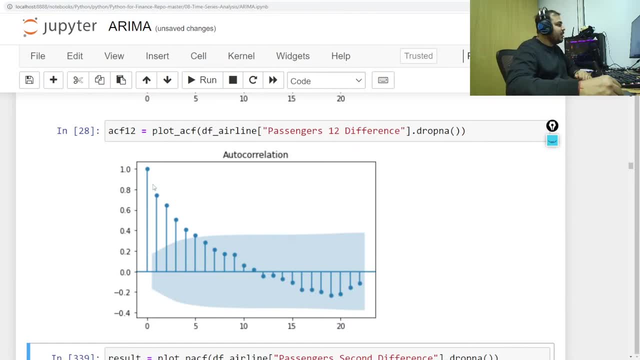 trying to show you how to implement Arima model. Now, in this particular case, you can see that it is going down, down, down and it is going there. So here, if I want to select my queue value, what? what would I select? Can embed: tell me. 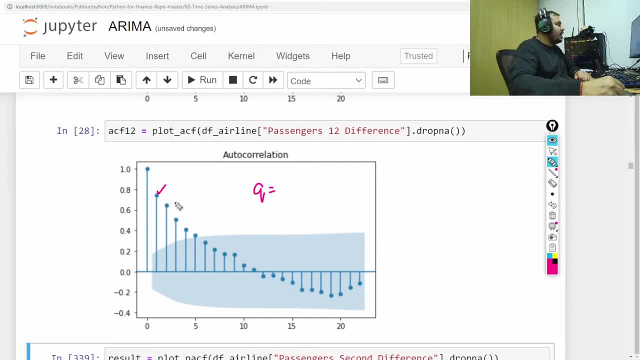 now What should I select? my queue value 1, 2, 3, 4, 5.. I can select 5 and remaining all Here. you can basically say: from here to here, there is no much impact on the correlation. That basically means I may consider considering the five previous seasonal data and try to see this with respect. 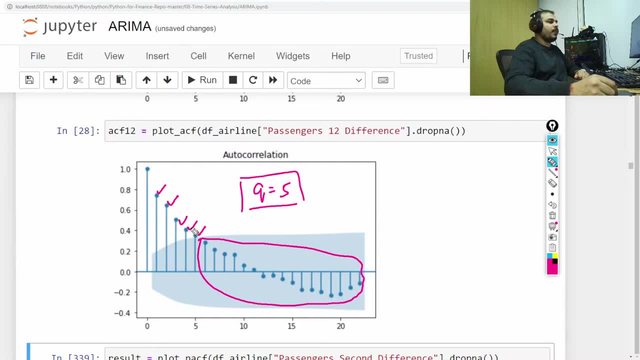 I hope everybody is able to understand. Yes, Yes or no, Amazing First is for zero. no, You don't count that First is for zero. So from here you count. So here also you can see that as you go ahead, your probably as we go future like this, it will be increasing. 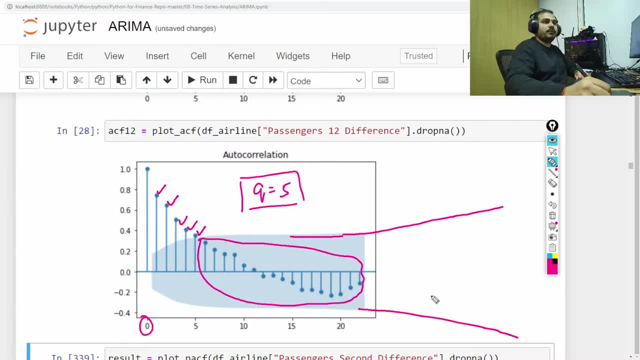 Okay, it will be increasing. The error will be increasing with respect to the bound Right: Perfect. So I have actually showed you this Now. similarly, let's go ahead and select with respect to our, with respect to our PSEF. 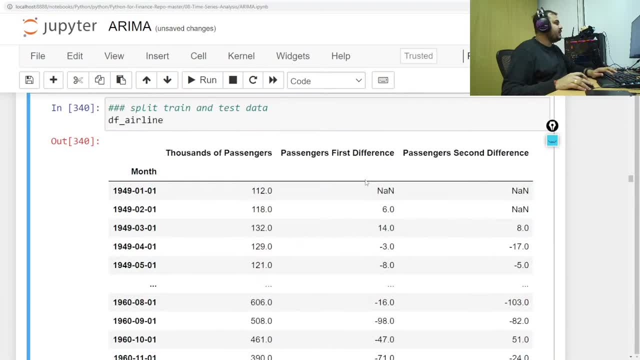 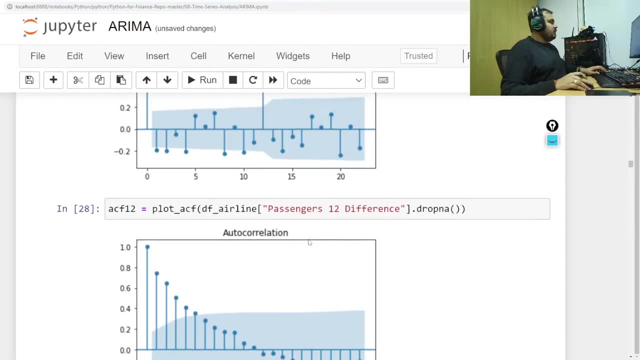 Now PSEF plot I can see over here. This is how PSEF plot is done. Okay, Here also you can see some kind of seasonality. So what I'm actually going to do? I'm just going to copy this. 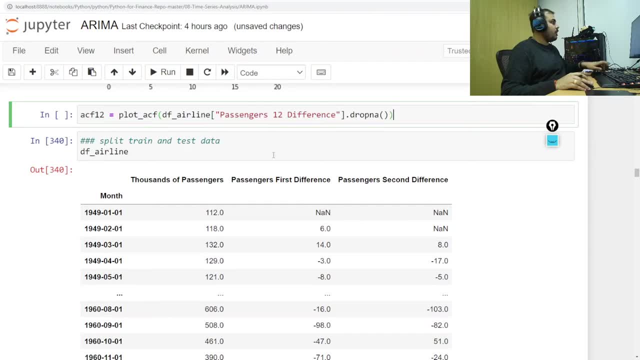 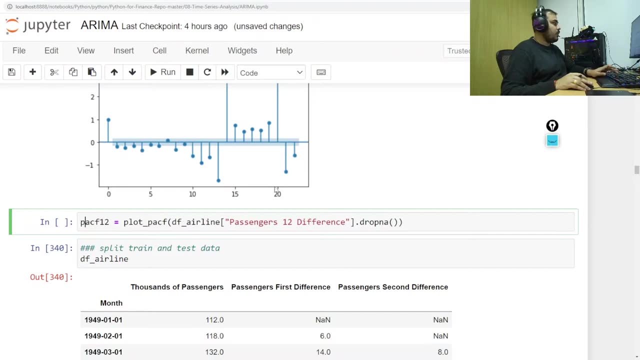 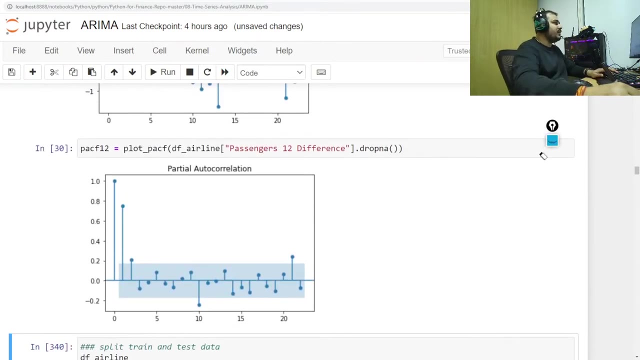 I'm going to plot it over here. So here you can see, plot underscore PSEF. Okay, If I execute it, Here you can see. You can now see that. yes, definitely my P value I can think up to. I can first of all try and create my model up to: P is equal to two. or next value that I can say: 1,, 2,, 3,, 4,, 5,, 6,, 7,, 8,, 9,, 10, P is equal to 10.. 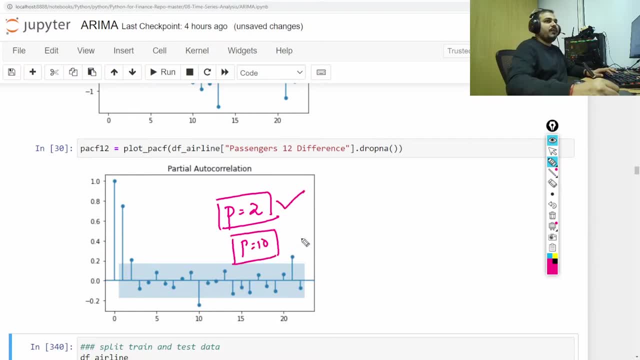 So first I'll try to go and see with respect to P is equal to two. If it works, fine, Okay. If it works fine, then it is fine. If it does not work fine, I'll go with. P is equal to 10, because here you can see that one line is going above the upper one. 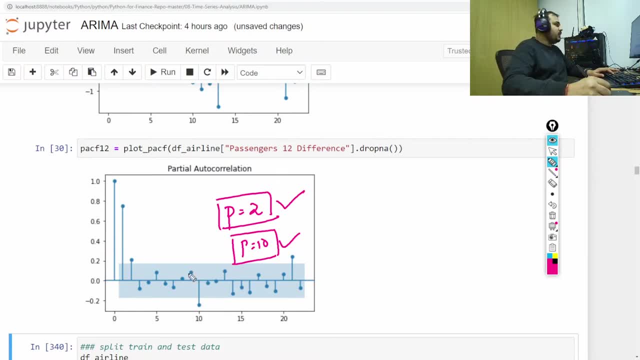 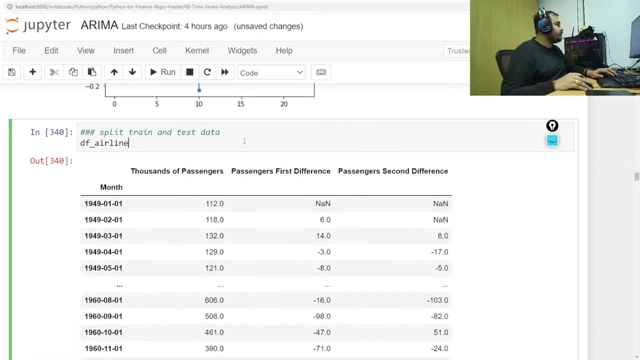 Should we count the line? if it touches the bound, Yes, Unless until it's above this or it is in that border, you can definitely try it out. Clear, everybody, Amazing. So now if I go and see my DFN square inline, you can see thousand passenger first difference. second difference: passenger 12 difference. 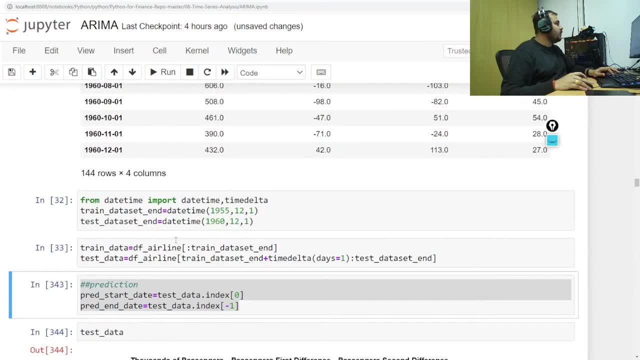 Now let's create my train and test data. Now let's create my train and test data. So here you can see: from this date to this date, I've actually created my end date for training data and date for test data. Okay, And then I'm executing this. 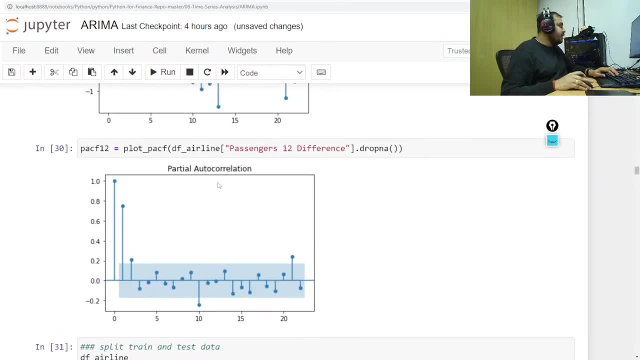 This will basically have my train data, With the help of PACF. you are basically performing. You are basically performing what you are performing with respect to this. You are basically performing auto regression With the help of ACF. you are performing. 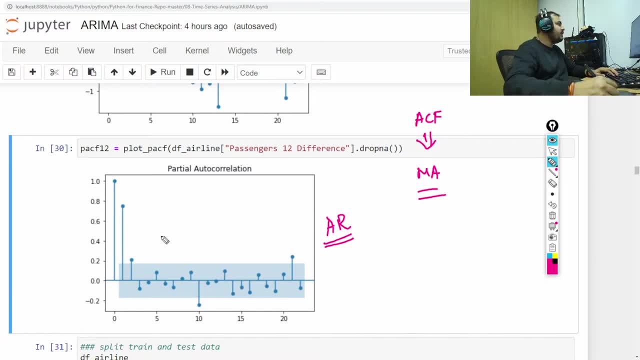 Moving, Moving average, which I discussed yesterday. With the help of this PACF, you find out the P value. this Q value And D value is nothing but differencing value, which you can also say it as integrated, Okay, Dynamic pricing. it may come to ARIMA. 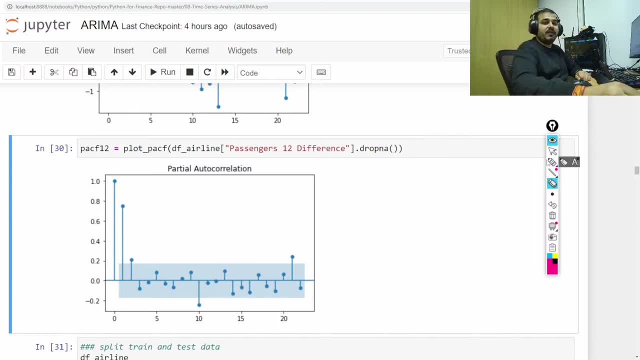 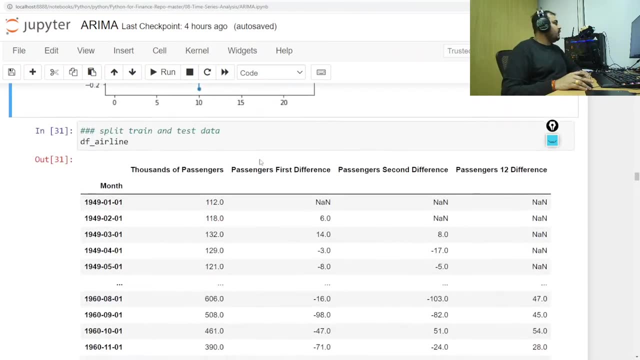 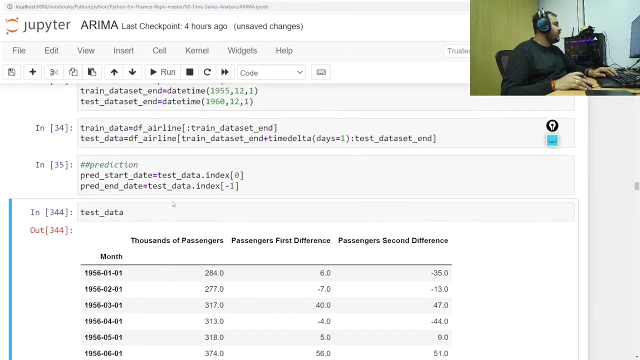 Yes, But it depends on the type of data that you have. If you have a seasonal data, then I would suggest yes, you can actually use. Okay, Now, done, done, done. This is done. So this is my training data and test data. with respect to my prediction on the test data: 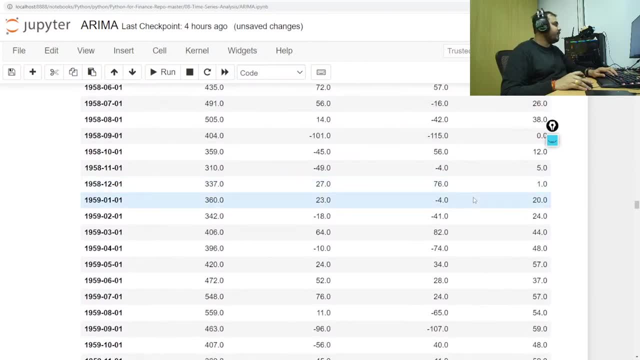 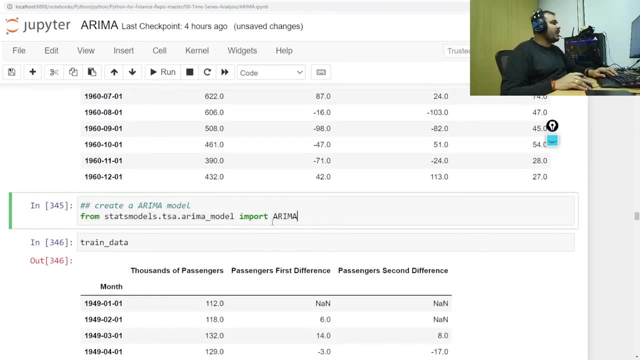 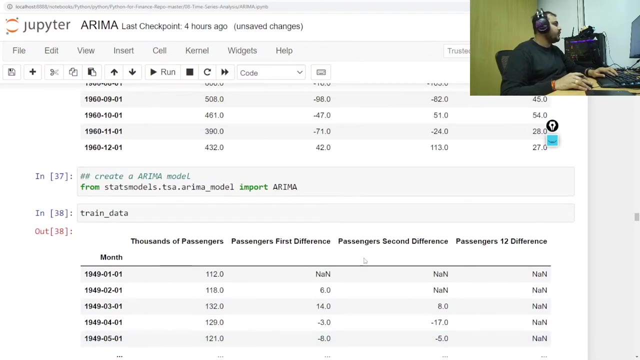 I can see this. This is my test data. here You can probably see everything. Just keep on executing till here, guys. I think everybody will be able to execute it. Now let's try to do ARIMA. Okay, So ARIMA, I will just import ARIMA and then I'll probably see this train data. 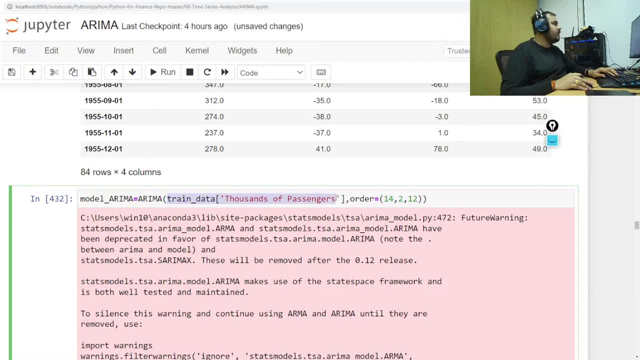 Now in ARIMA, what all features will go. First of all, my training data will be going as thousands. I will be able to see thousands of passengers. Okay, Yes, Q is the number of impacts. No, no, Not, not like that. 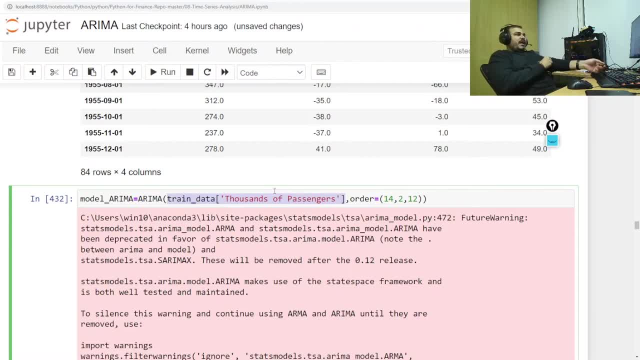 Q. you can consider that it will try to give you a coefficient. See, Anyhow, when we are applying ARIMA model, you know, with respect to every timestamp there will be a coefficient that is getting applied. So if you see that, okay, from one point of time, you can see from that it is crossing the upper bound. 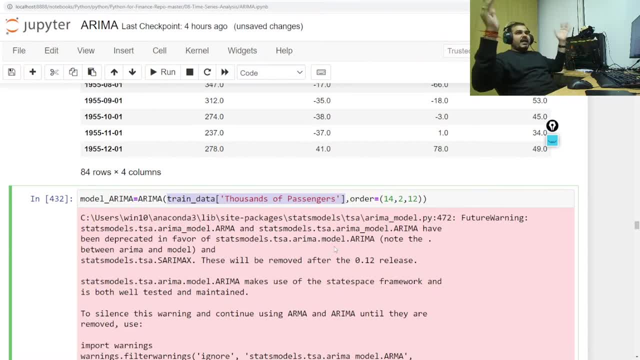 Let's say, after five to six timestamps, one more is crossing the upper bound, upper bound. You can experiment that with respect to 6.. That basically means you are going to combine all those features, that is, t minus 1, t minus 2, t minus 3, t minus 4, t minus 5, t minus 6. 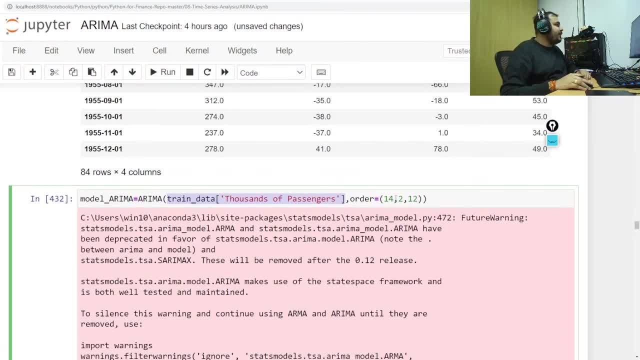 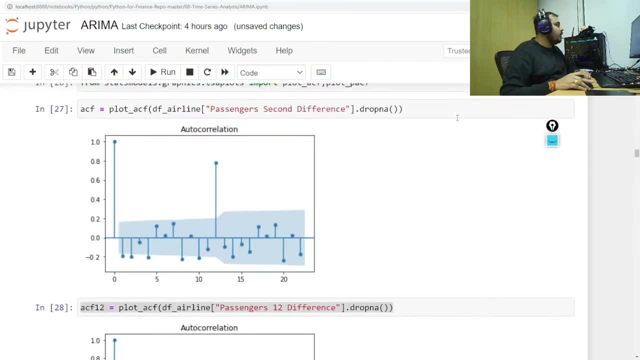 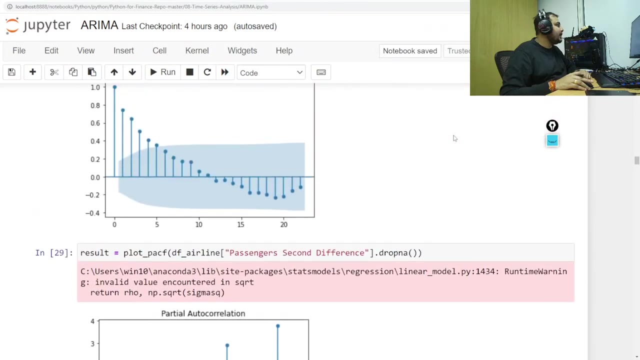 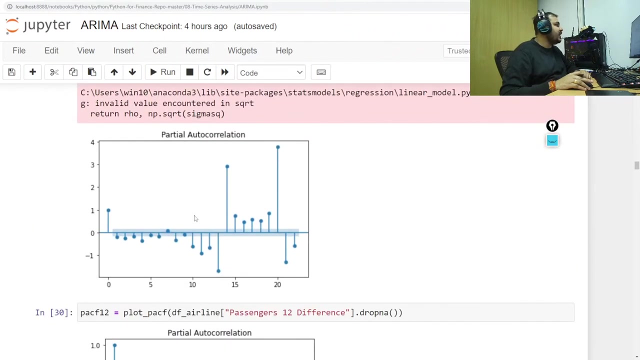 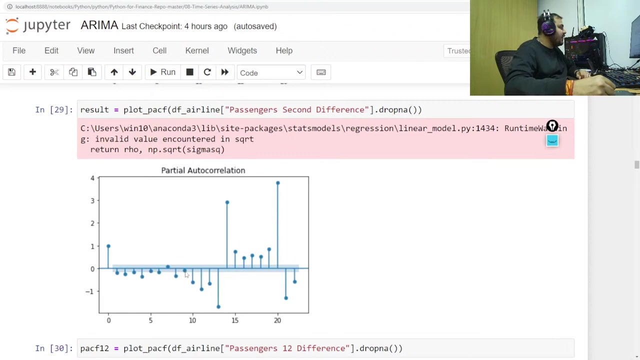 like that. Okay, Now let's say: why did I probably take for Arima as 14?? Can anybody think: See, go and see the graph. Go and see this graph, Passenger, second difference. Go and see, with respect to this graph, Why p value is taken as 14? See, let's count 1,, 2,, 3,, 4,, 5,, 6,, 7,, 8,, 9,, 10.. I can. 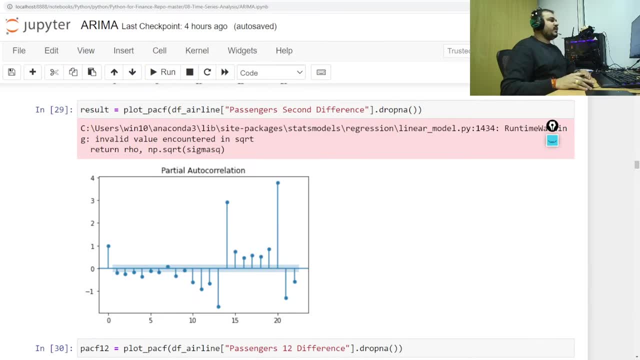 start from 10.. Okay, I can start from 10.. So let's first of all start with 10.. So here we have a graph. We have a graph of a passenger. We have a passenger, We have a passenger. So here I am, setting my p-value to 10.. 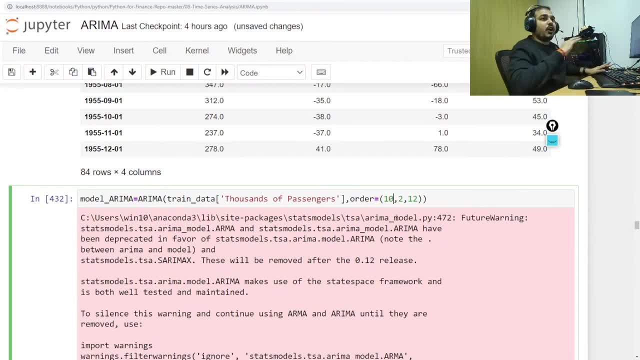 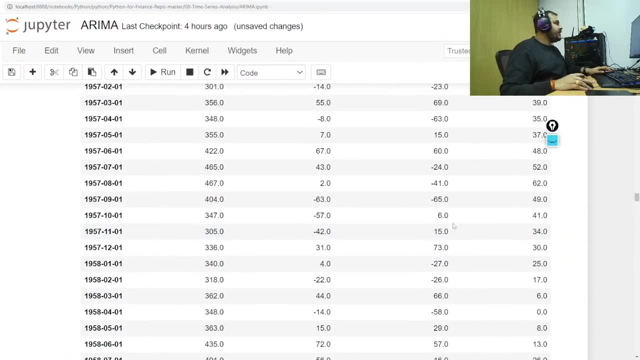 How many number of times we did differencings initially- This is not for seasonal, okay. How many times we did differencing? Probably 2 times, So I have kept 2 times value over here. Now let's go to the ACF and see what was the, what was the line that we could see over here. 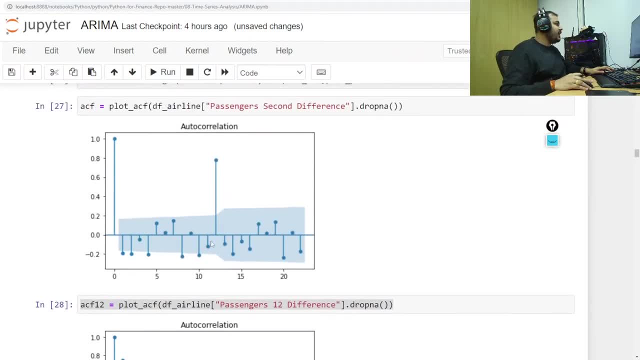 This is after 1,, 2,, 3,, 4,, 5,, 6,, 7,, 8,, 9,, 10,, 11, 12.. So 12th data is basically having a high impact, right. 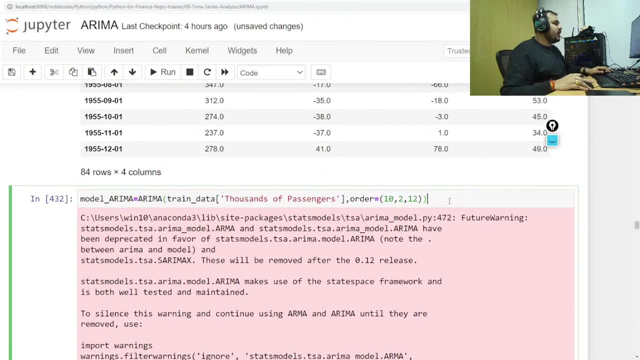 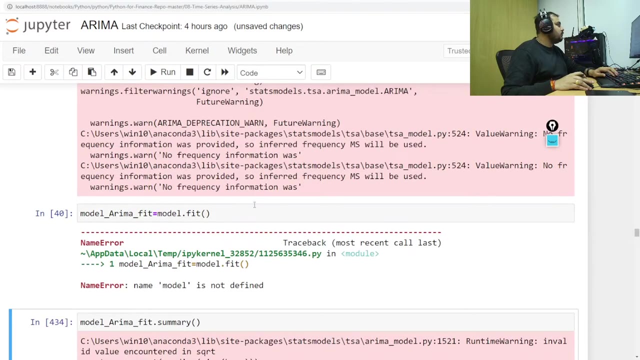 So I am basically going to set it as 12.. So here it is set as at 12.. So order: this specifies my p-value, p-value and q-value. So once I execute it and then once I do modelfit model, why model is not okay? model underscore. 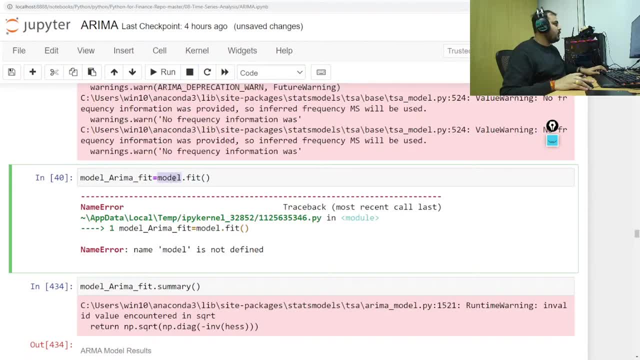 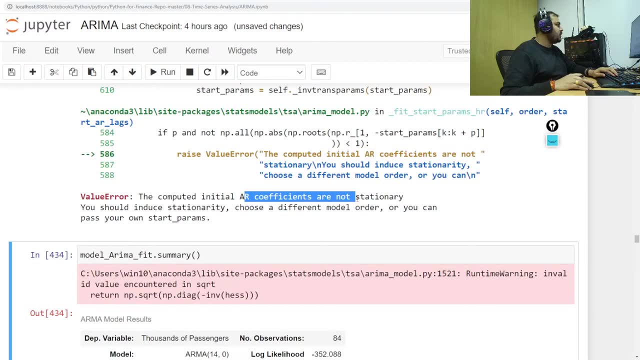 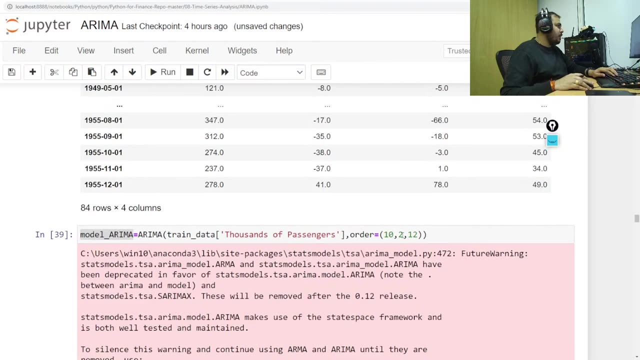 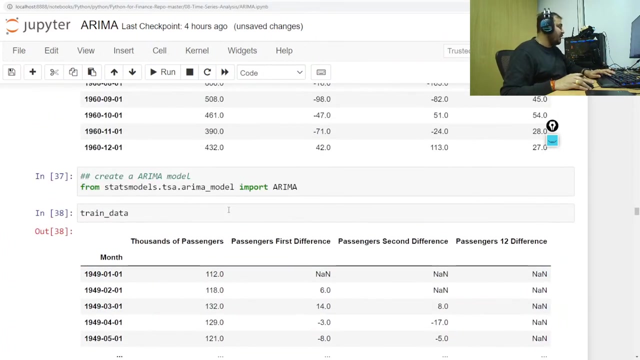 arema model- underscore. arema model underscore. arema dot fit. okay, I am getting an L. The computer not stationary, you should. okay, but why? let's make this to 0 for right now? okay, I will make this value as 0, moving average. I will just check it why the error is coming. 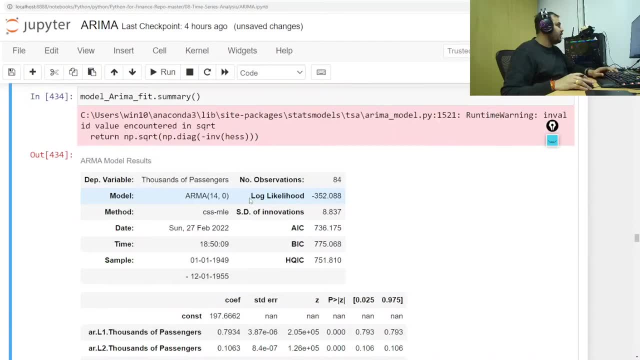 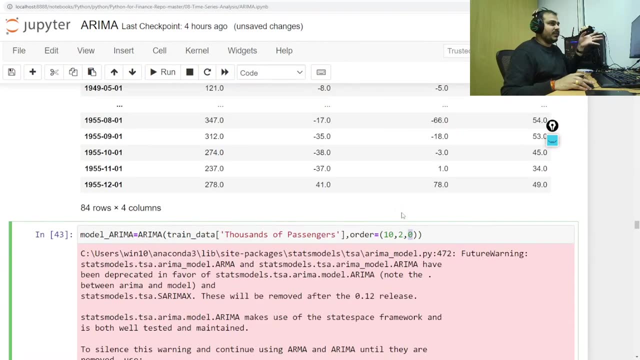 okay, So this has got executed. if I do fit, make this value to 0 guys for right now moving average, we will just try to focus on auto regressive. okay, We will just try to focus on auto regressive. that is the p-value. 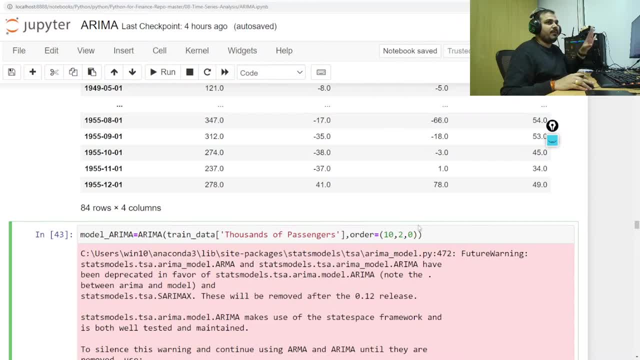 Differencing is 2, let's keep q-value for some time, Because q-value if I am doing 12, then I have to move it to seasonal arema- okay, Because seasonal arema will give you the 12th value, right. 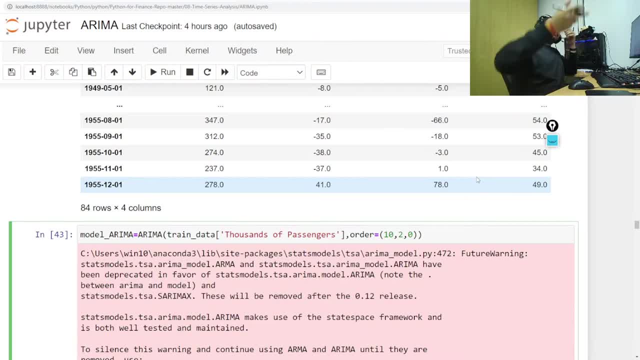 12th, if you are considering 12, with respect to the data set, that becomes yearly data. So I am just going to execute this. this, this summary, is done. Now see, let's focus on the summary. Let's focus on the summary. 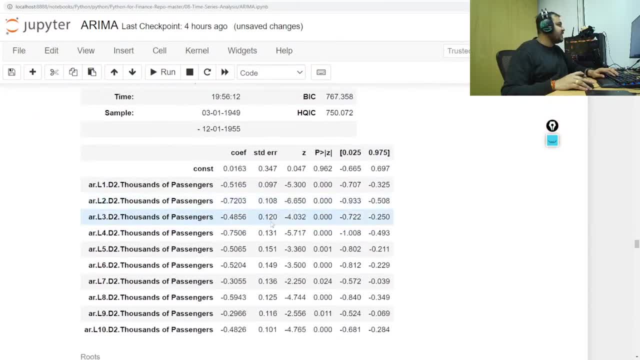 Let's focus on the summary. Okay, Let's focus on the summary Now. summary basically says this all thing. see, What does summary say? This is my constant, that beta 0. I told you These all features are less than 0.005.. 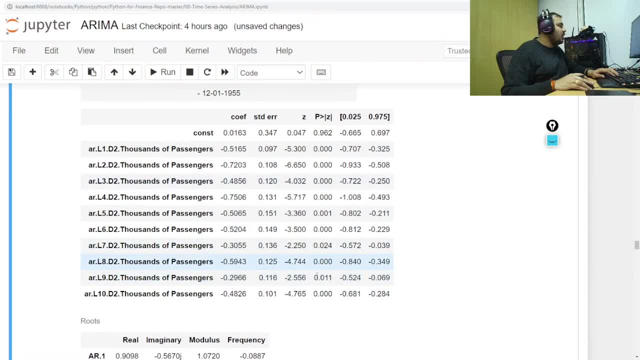 So that basically means all these features has a good impact. All these features till now, whatever 10 lags that I have actually taken- okay, 10 lags that I have actually taken- all the p-value is less than 0.005, okay, 0.005.. 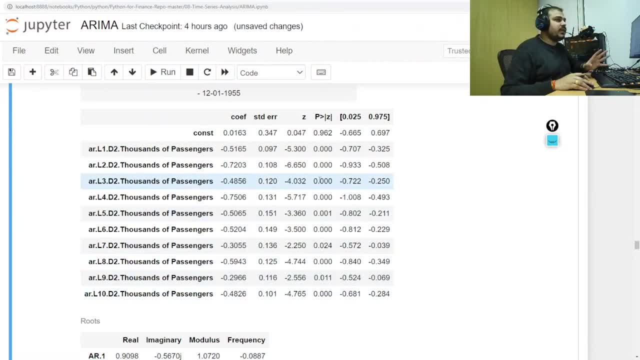 That basically means it has a positive value. It has a positive impact on the current timestamp data that we are trying to predict. okay, So here you can see: all are less than 0.005,. see, Is it? No, no, 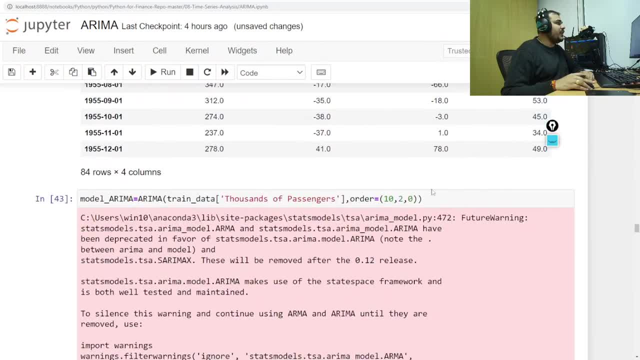 Can you see it, guys? All are less than 0.005.. Please don't make sure that you keep this value as 0, otherwise you will get an error. okay, with respect to this one, with respect to arema, when you are trying to find out. 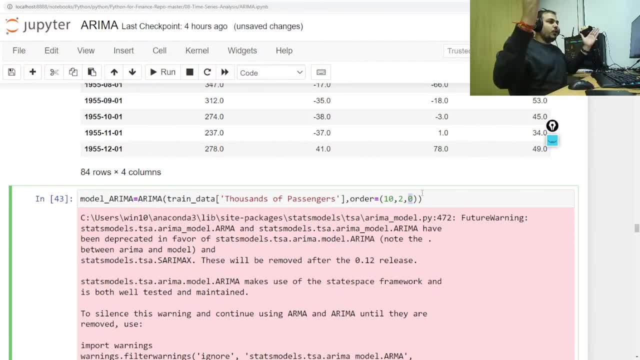 arema, Because for seasonal data, you cannot take 12 months. If you want to, if you are probably taking 12 months, you cannot take 12 months. You cannot take 12 months. You cannot take 12 months. That is your Q value. 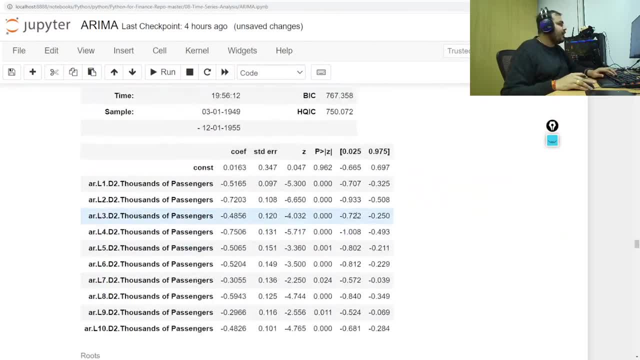 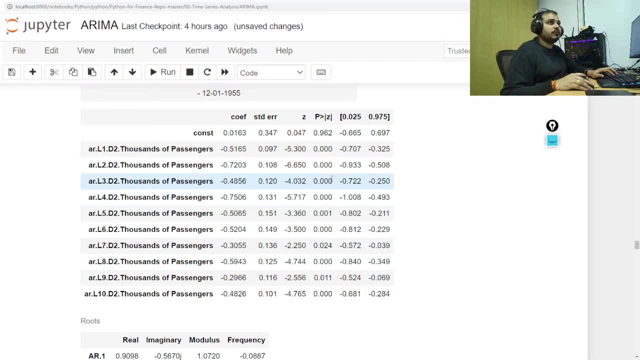 You can better go with seasonal arema. okay, Everybody clear over here. Everybody clear, Yes, Yes, yes or no. Oh Krish, it is very difficult. I know Nothing is so easy, So you are getting paid so high, right? 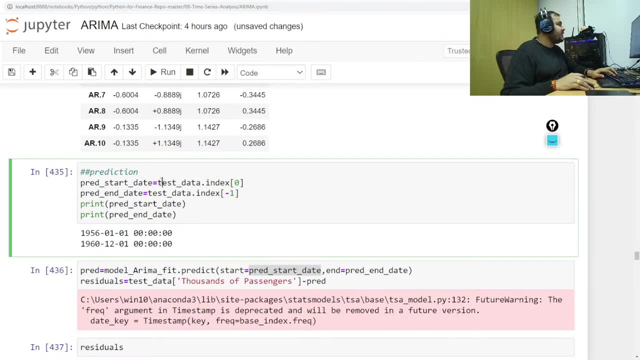 Okay, Now let's go to the next step. Next step: I will start doing the predictions, But for the predictions I need the start date and the end date from where I want to do the prediction. Currently, my prediction will be for the test data that I have. 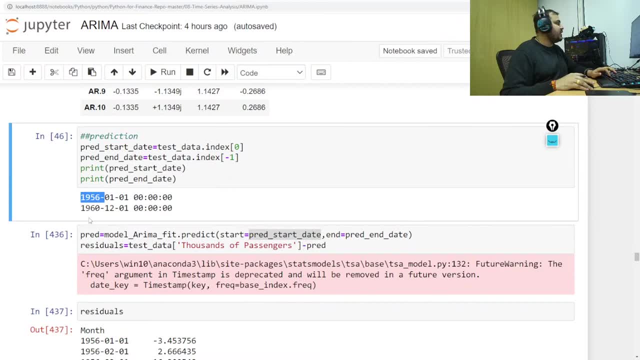 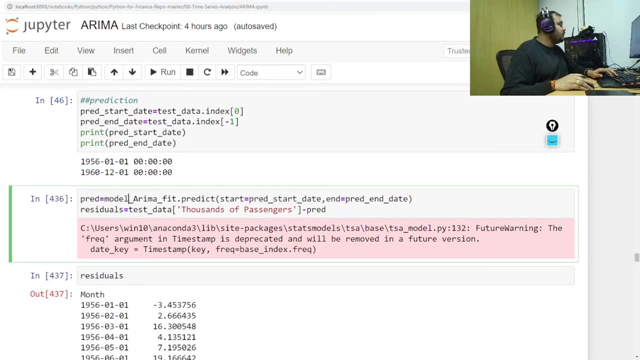 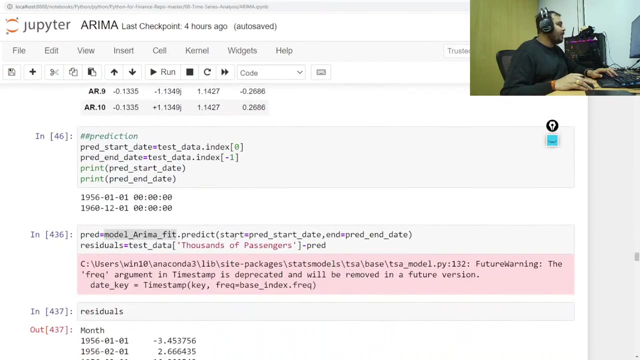 So this will be my time from 1956 till 1960.. I am just going to do the predictions, okay. So here what I am actually going to do. again, I will write model underscore arema, underscore fit- See. here you can see model underscore arema, underscore fit- dot predict. 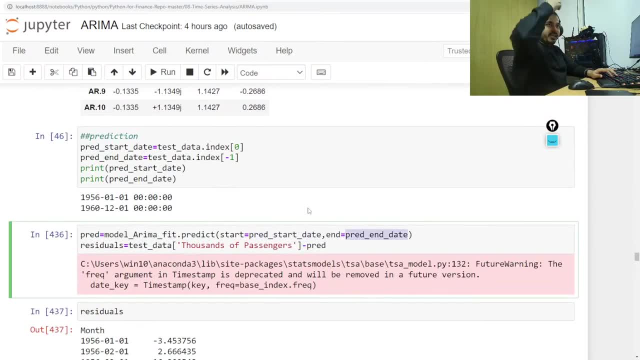 The start date will be prediction start date. End date will be prediction end date. So once I execute this here, you will be able to see. I will get pred and this pred I will put it inside. I will just try to find out the test data difference and try to find out the residuals. 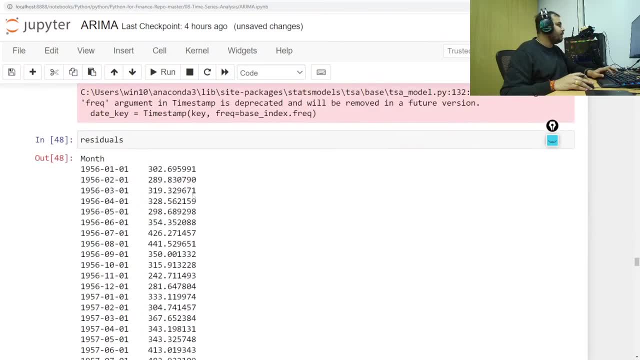 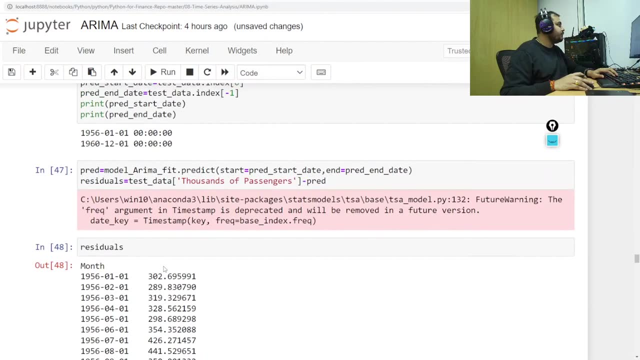 okay, So here I have executed. This is my residual. This is my residual. You can see this. These are my residuals over here. These are my residuals. okay, Now let's go and plot with respect to all the residuals. So here you can see. 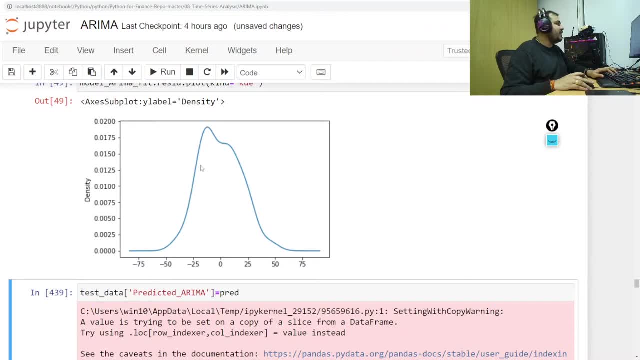 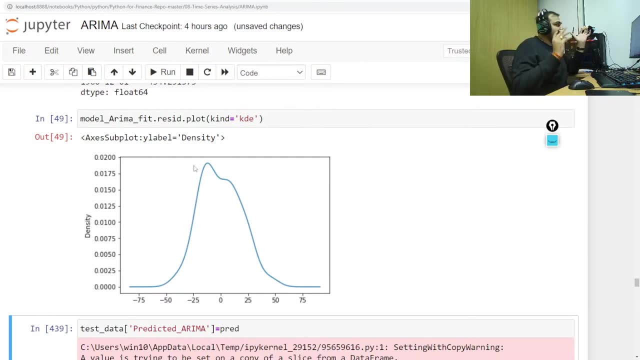 This looks like an amazing centered graph, Don't you see? This looks like a good graph, like normal distributed graph, right, Which is very good. okay, That basically means we are going in the right track. probably because there I have not specifically 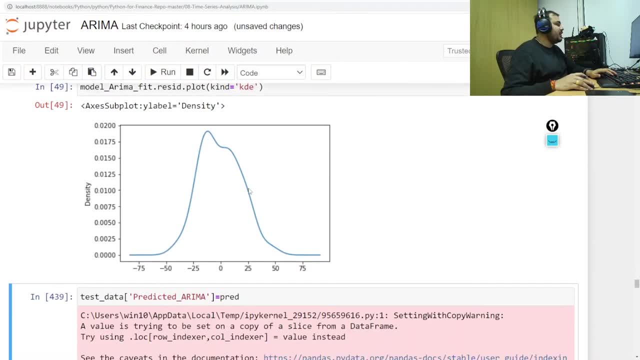 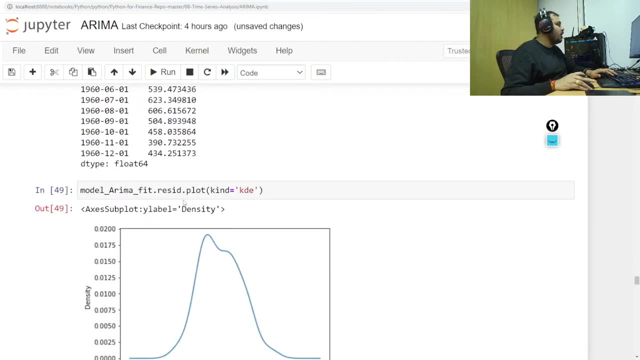 taken the Q value. okay, Yes, little bit is there, but it's okay. Now, all this predicted value, what I am actually going to do, all this predicted value, I am just going to put it inside another column, okay, And that column I am naming it as predicted underscore arema. 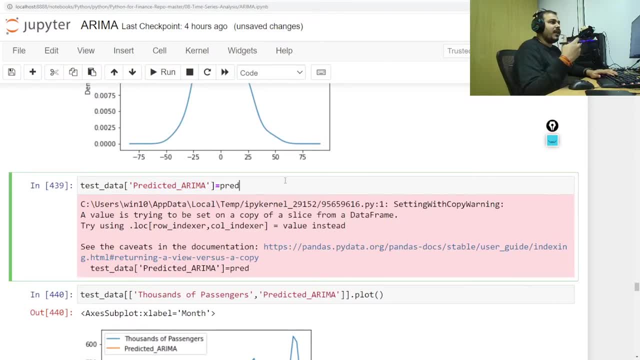 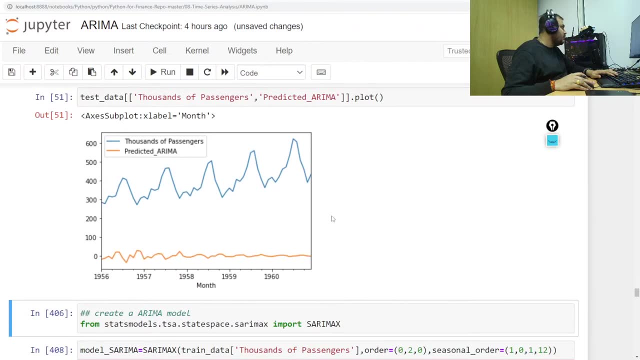 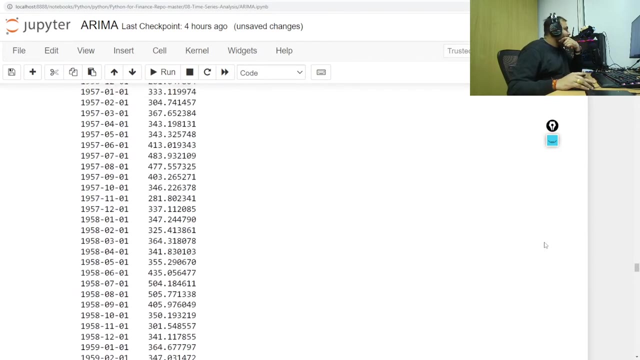 That basically indicates that, with the help of predicted underscore arema, I have done this prediction. So here now, if I try to plot it, oops, this is a huge difference. What is the problem? Something, some mistakes have happened. Let's see. 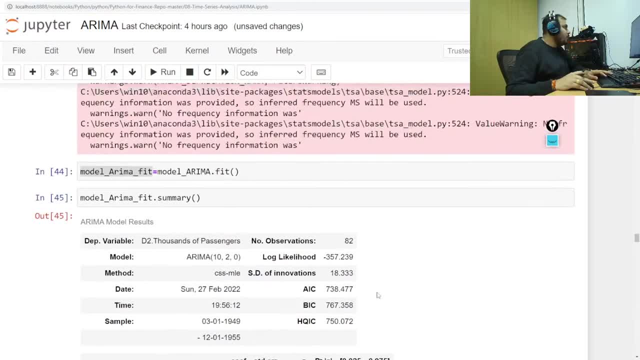 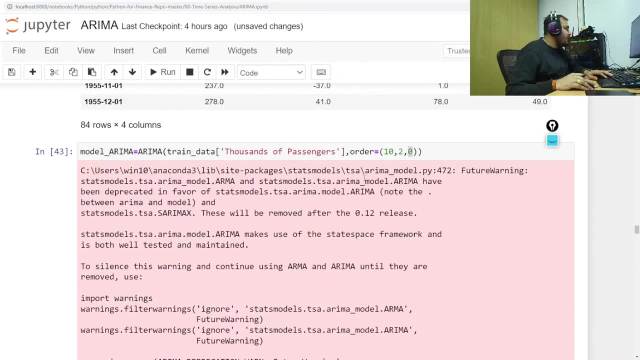 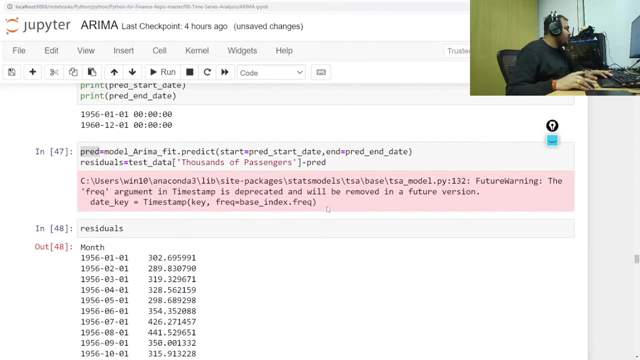 Some mistake has happened, guys. Let's see What was the error Order. this is this. is there? Thousands of passengers? fine, differencing 2, arema fit arema. summary: One mistake that I have actually done. let's see. 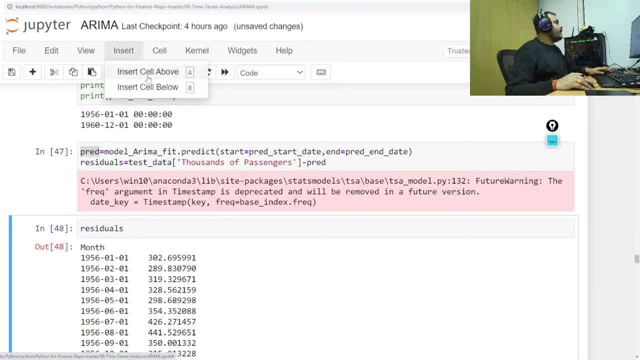 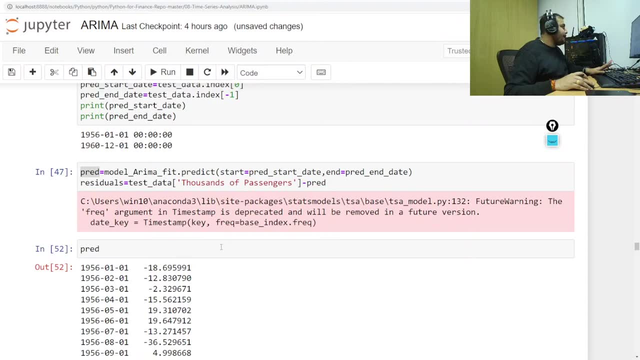 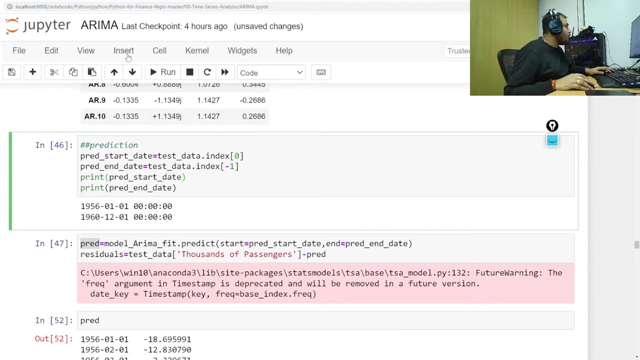 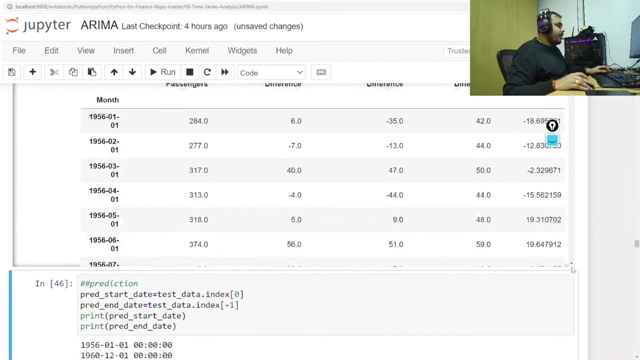 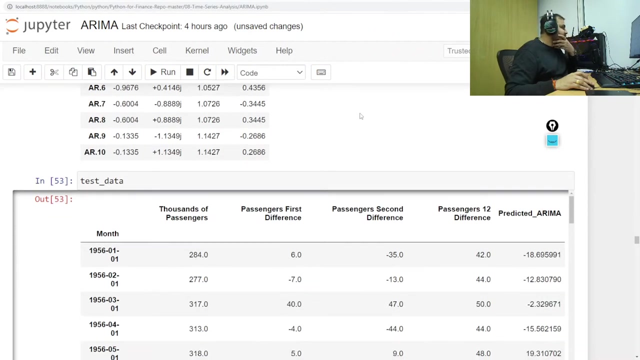 Pred what is pred. So I am just going to compute pred. The prediction value is very small. Why Start date, end date? right? Let me just check out my test data. This some some mistakes have happened Somewhere. I think I have missed something. 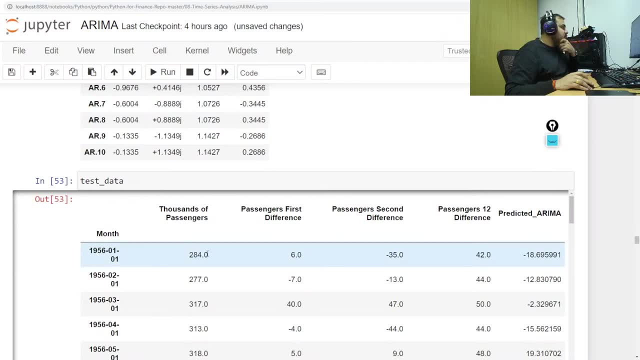 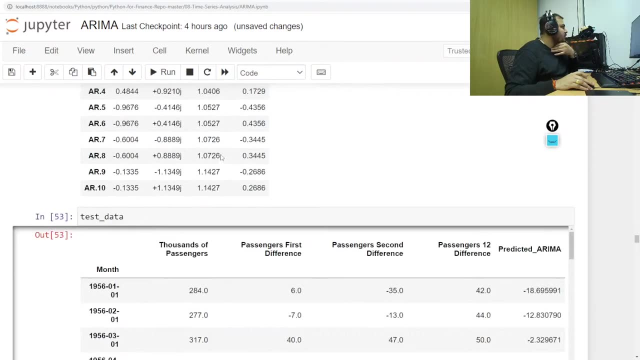 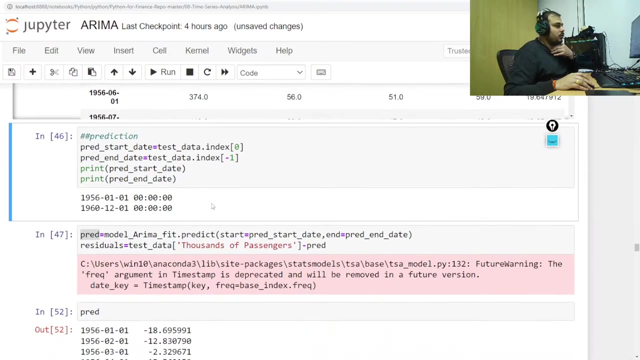 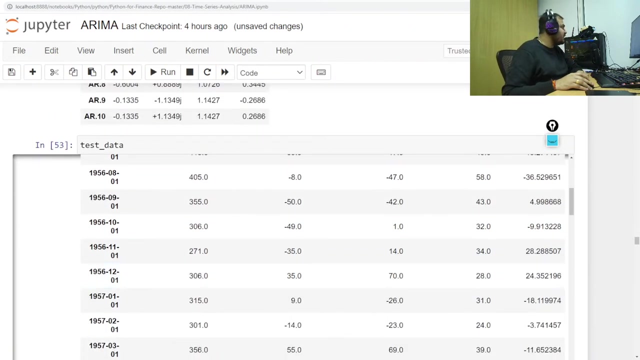 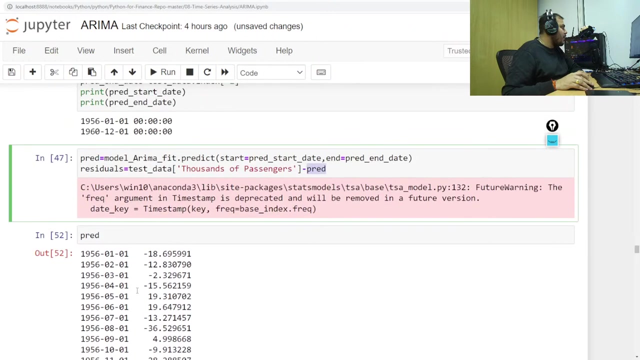 First difference: thousands of passengers. Second, I am predicted, arema, I have taken zero. Where I have taken zero. Where I have taken zero, It should not be zero, But where which line? Ex-cumulative Prediction: pred value minus residuals. 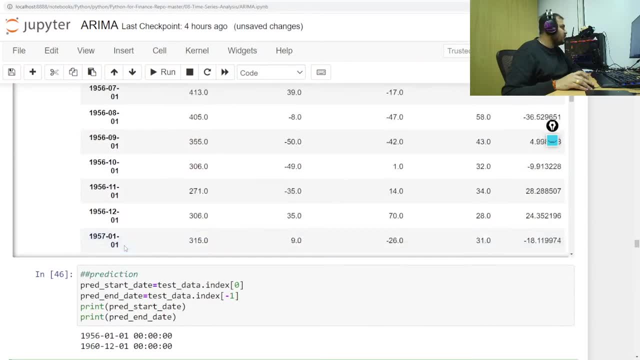 No, no, no, no, no, Q-val, it's fine If you take it as zero, also, not a problem. I think it should not be a problem, but let's see, I will just keep for testing. I will keep it for 2.. 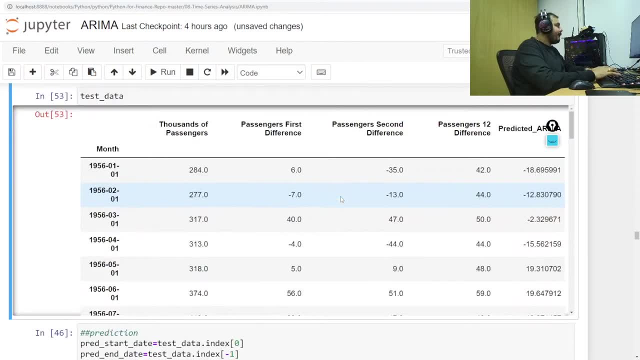 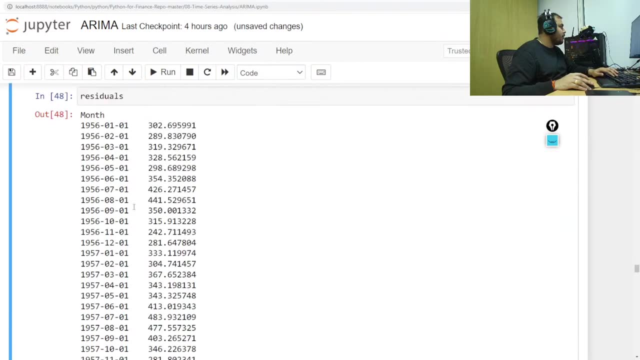 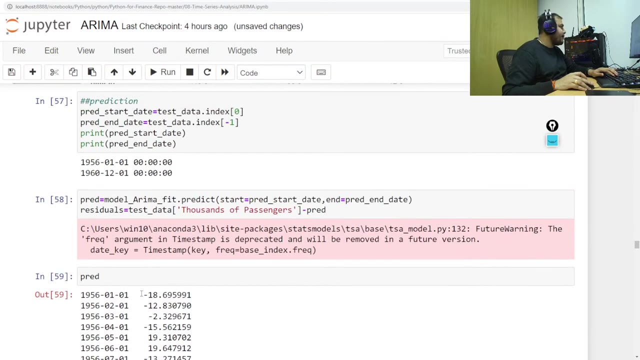 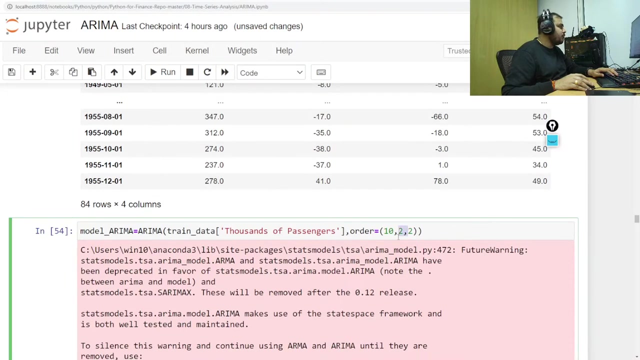 Let's see, Let's see. No, it is coming as same. T-value is not zero at all, It is 2. Thousands of passengers. order, Just a second. I made one alternate copy of the file that I was working with. 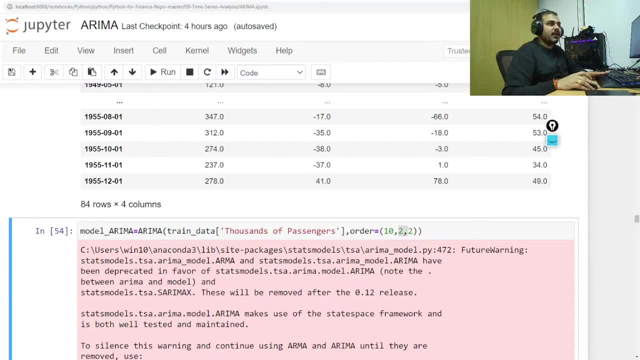 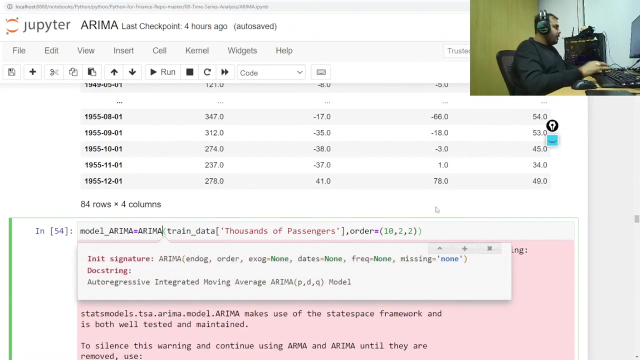 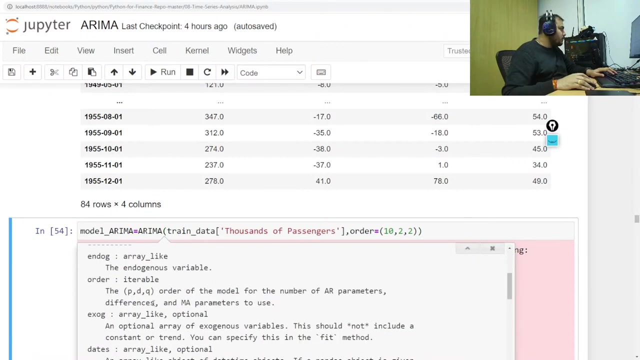 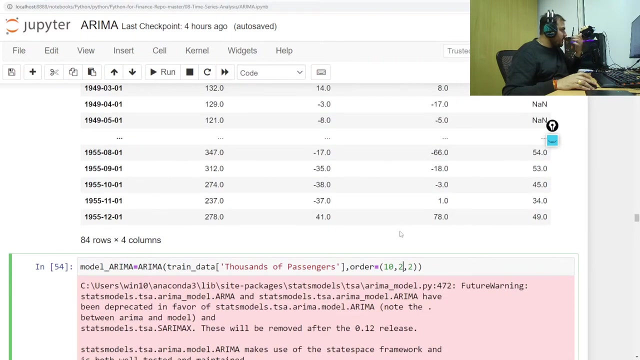 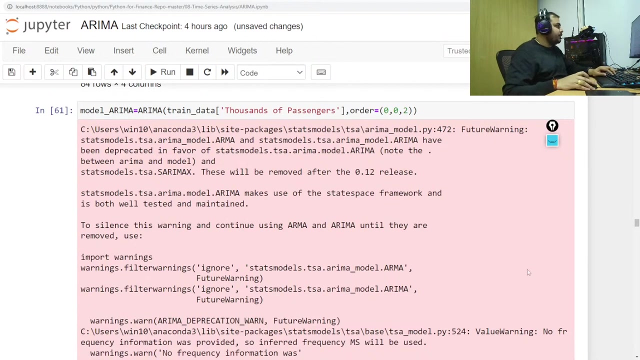 Just a second. Give me a second, It will get fixed. I am just checking what mistake I made. If I go and see ARIMA Press shift tab, The order is going to be Two time differencing, I think. since this is a seasonal data, it may not work. 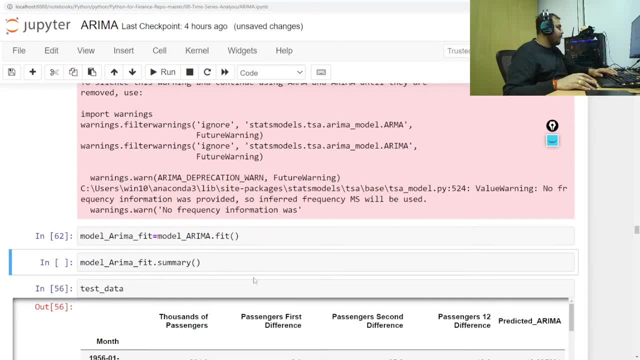 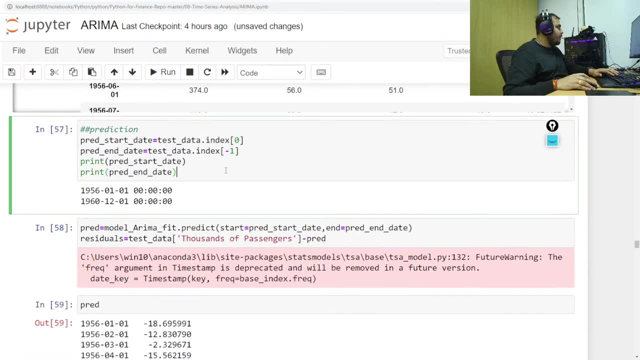 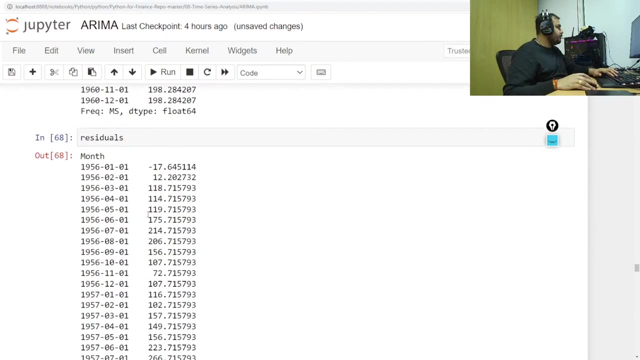 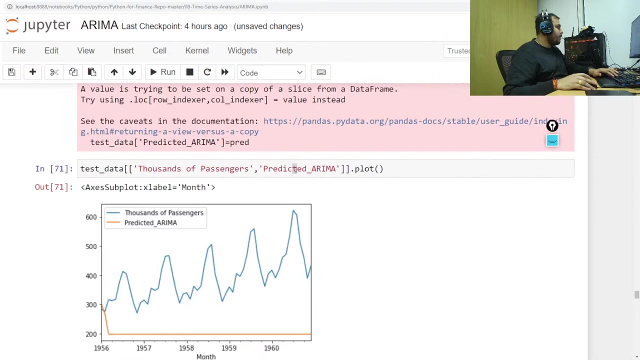 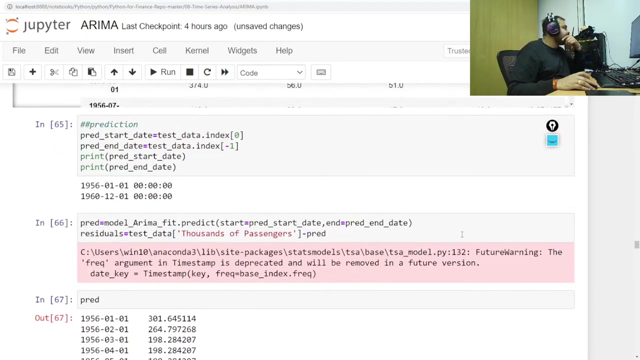 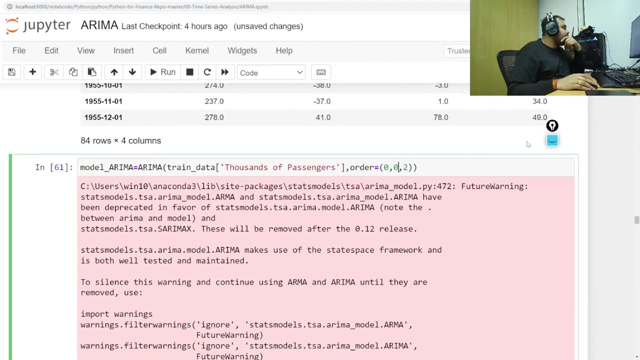 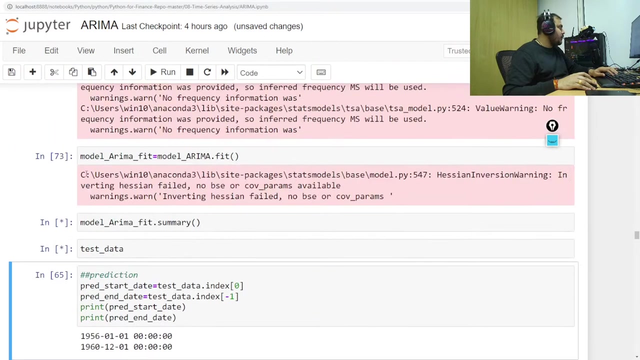 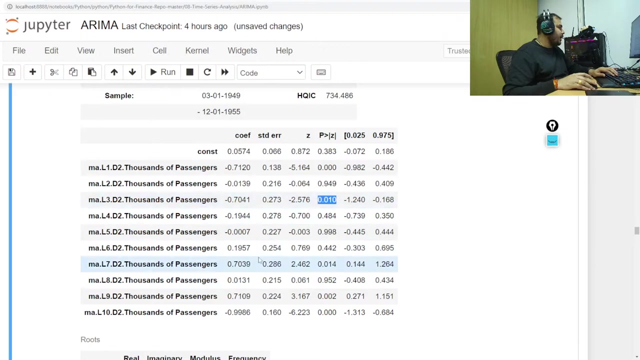 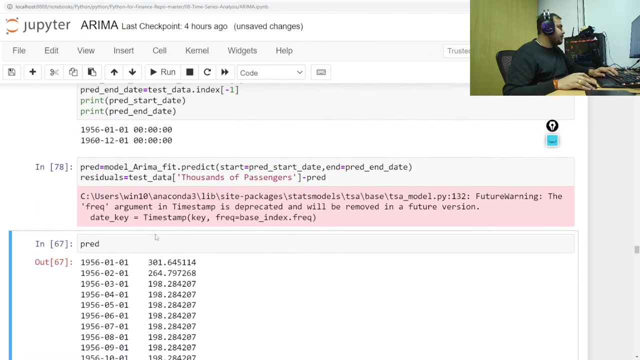 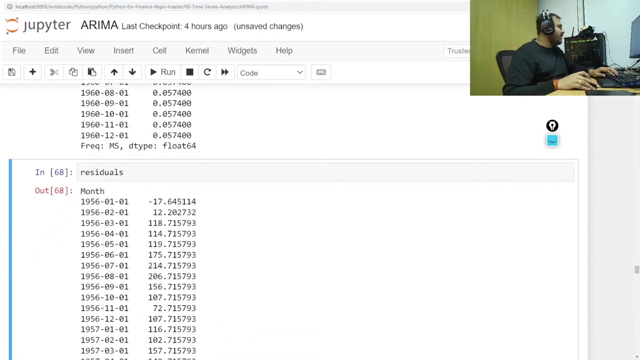 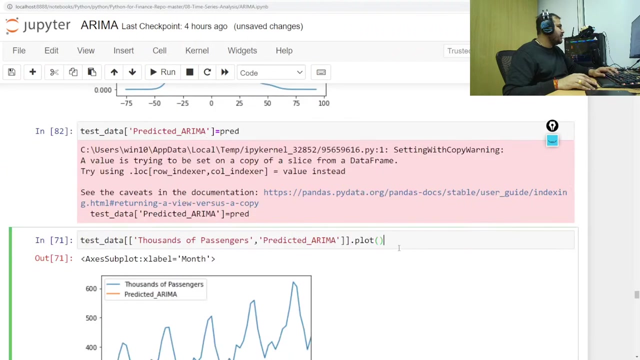 Just because of a seasonal data. Let's see Just a second. Just a second Probably. take ARIMApetsata. You can see there is a lot of unnecessary impacts. Okay, The value is getting reduced. Why There is some problem? 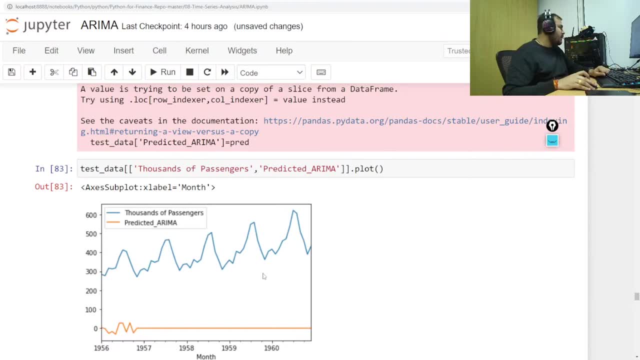 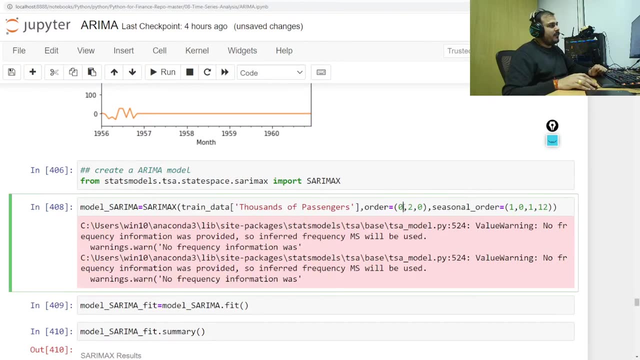 See this. The graph prediction does not look good. Let me try once with ARIMAX model. guys, Just a second: 0, 2, 0.. 1, 0, 1.. Because one time I did not. 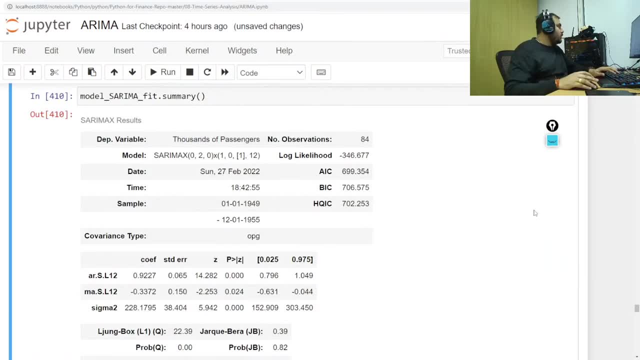 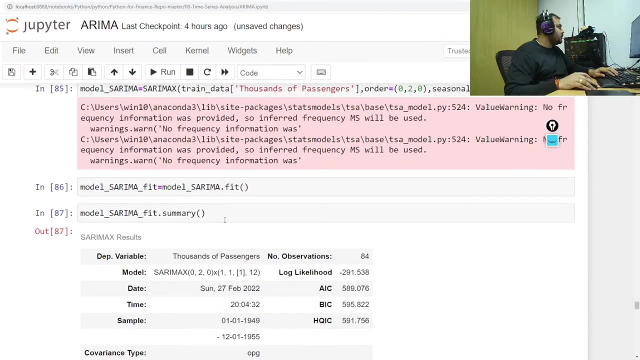 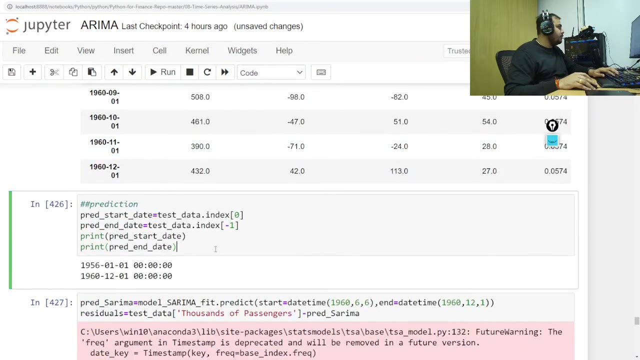 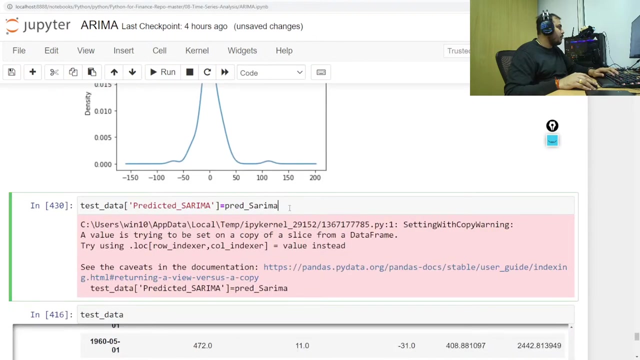 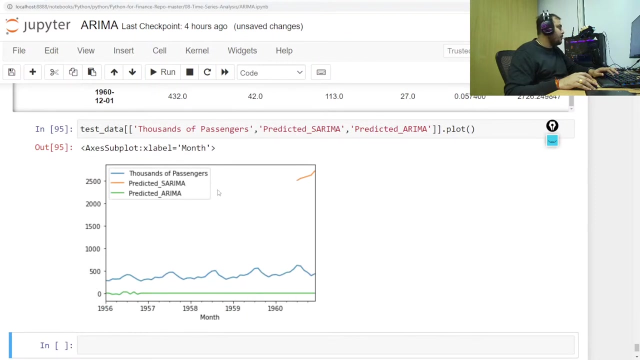 One time I did differencing. Let me just have a look. Probably it may work with ARIMAX Summary. if I go and see Okay, Bad summary, it looks like Let's do it again. Let's see ARIMAX is here somewhere here. 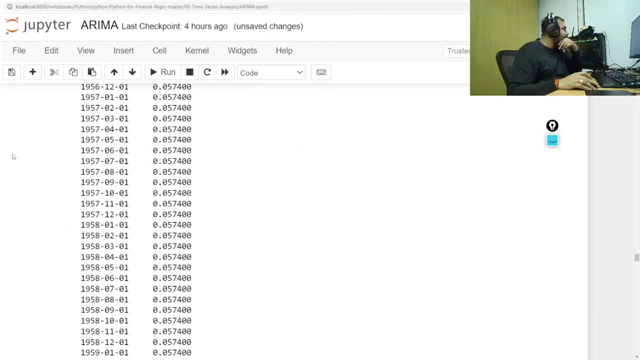 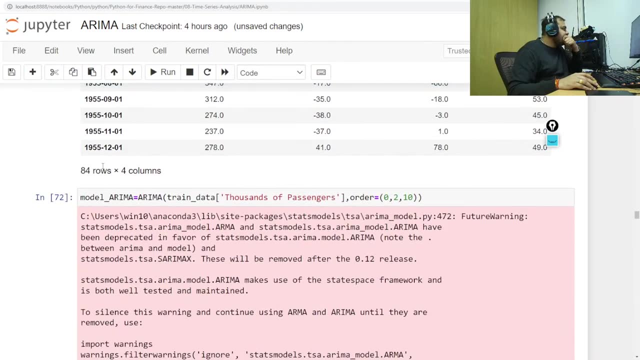 Something is missing. Okay, Anybody. Okay, Change it to: p is equal to 10 and q is equal to 0., 14,, 2,, 0., 2 and 2.. Can you please explain how the seasonal order should take place? 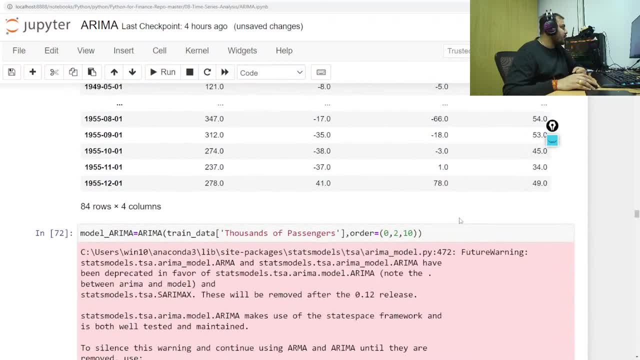 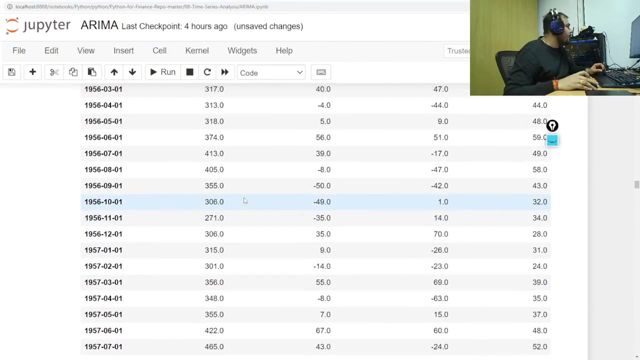 I will explain about this. first, Let's fix this problem, otherwise nothing will work. So if I probably take- Okay, Let's see this, Okay, Let's see this plot- Partial autocorrelation- Autocorrelation, Since for seasonal I don't have anything. 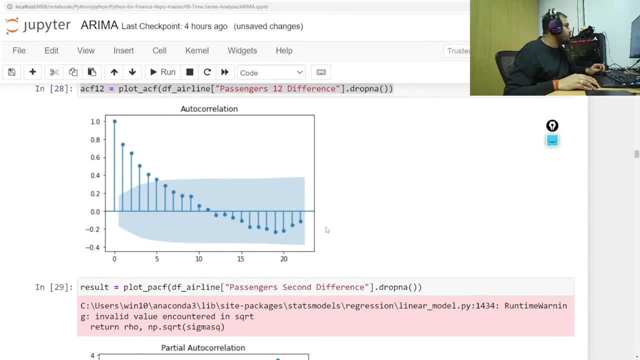 Oh sorry, I forgot to take for seasonal like this: 1,, 2,, 3,, 4, 5.. 5 is here And 1,, 2,, 3., 3 and 5.. Right So? 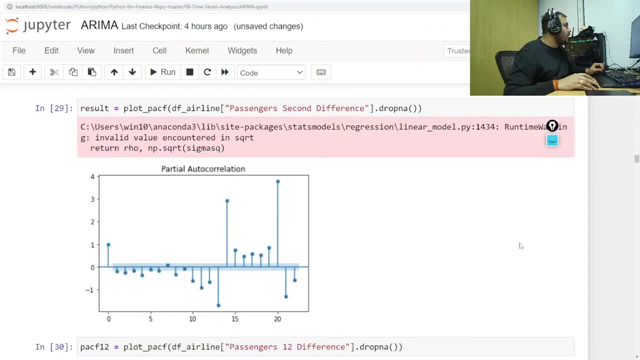 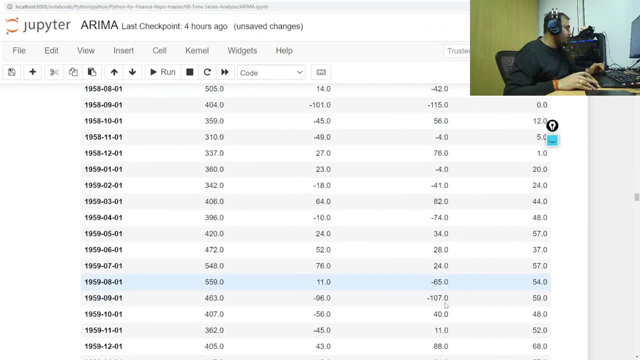 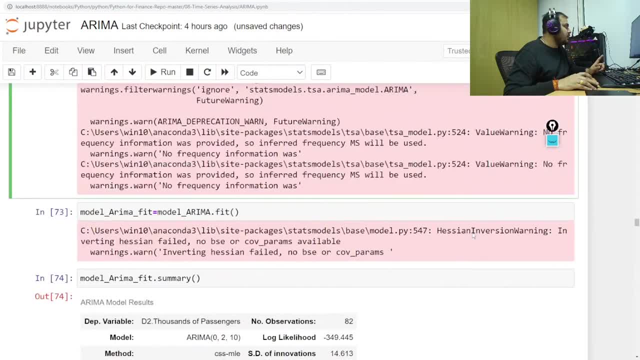 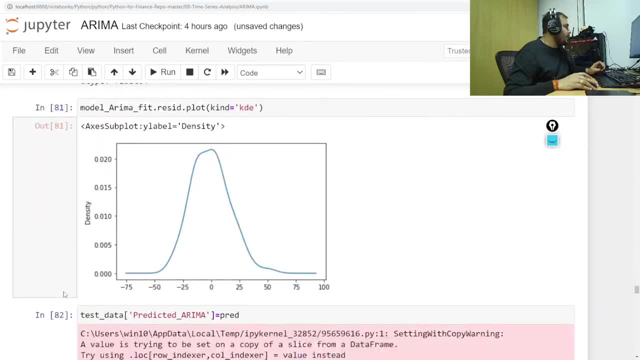 Okay, Okay, Let's see Just a second. guys, Just give me a second. Okay, I am fixing the issue For salimax once. I will also test it to that. 3 comma. Differencing: 0 comma. 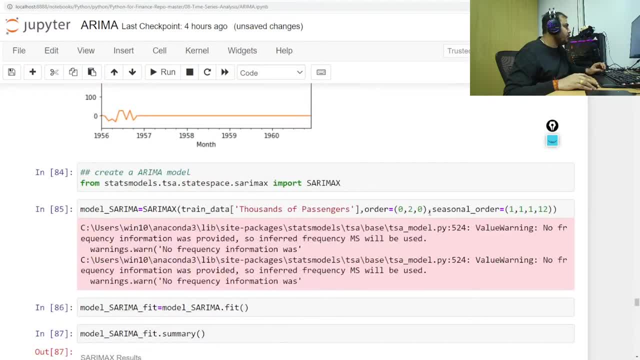 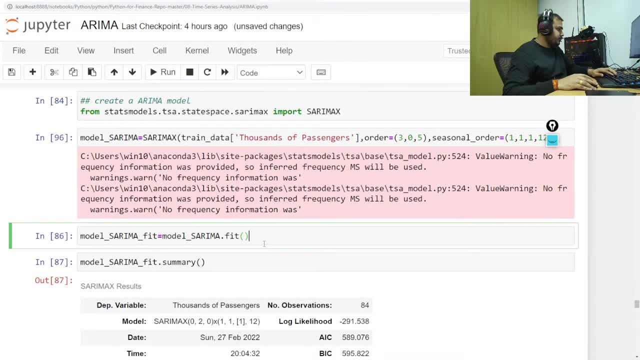 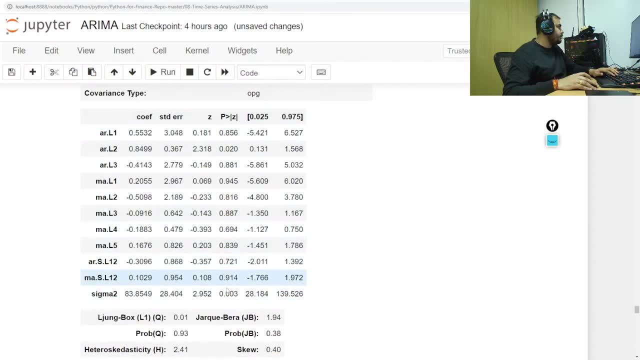 Okay, Okay, Okay, Very good, Very good, All right, Thank you for watching this video And, if you like, please share it on your social networks. Well, thank you so much and have a nice day. Rimal 123 lags, and this is basically having a moving average of this. 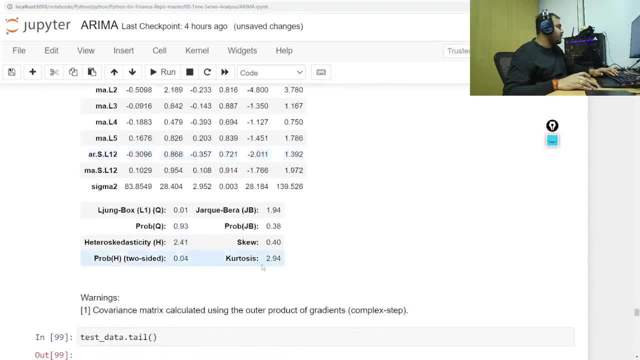 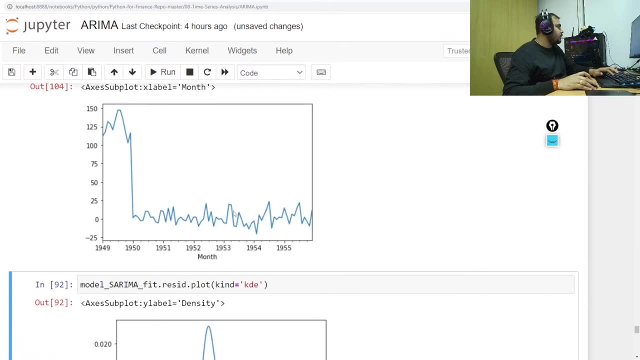 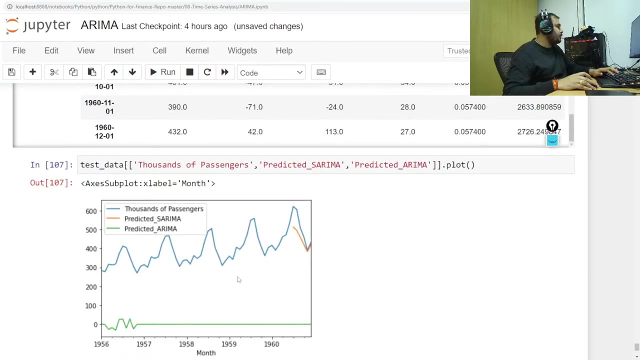 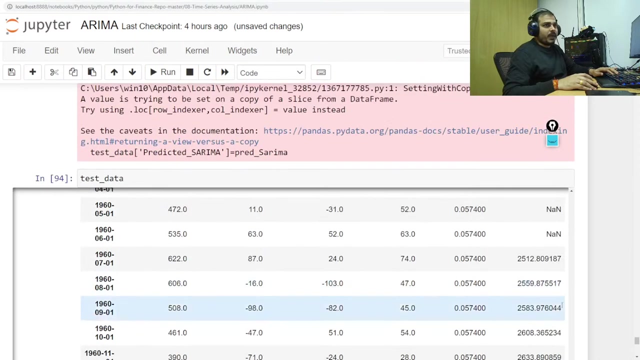 If you have a quick comment now, we'll try to start this video because it doesn't take much- 5, quase five minutes. but if you have any other questions you can also share. Wow see, predicted Serimax looks good. ok, let me. let me do one thing, guys. see the. 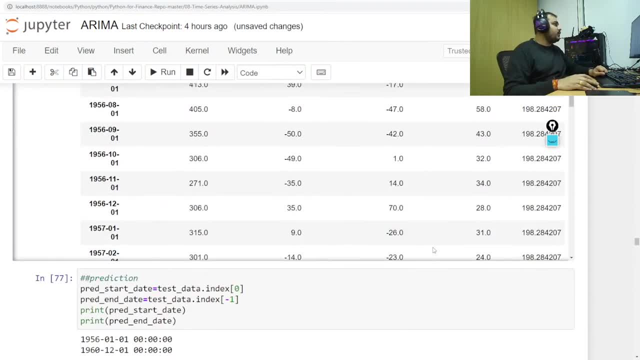 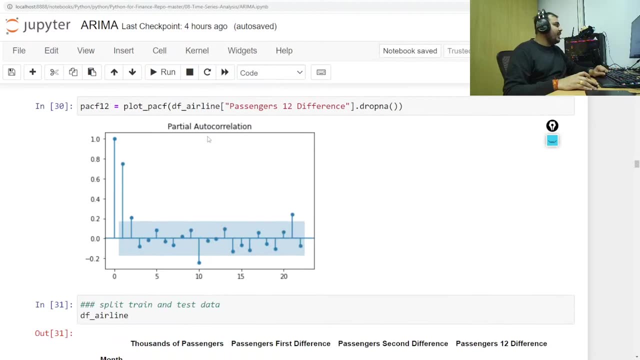 thing, probably why I think it is not working with respect to Arimax model, because this is a seasonal data. now let me just show you how did I predict. see, with respect to the PACF model, this will basically give you the p-value for seasonal data. ok, so here, if 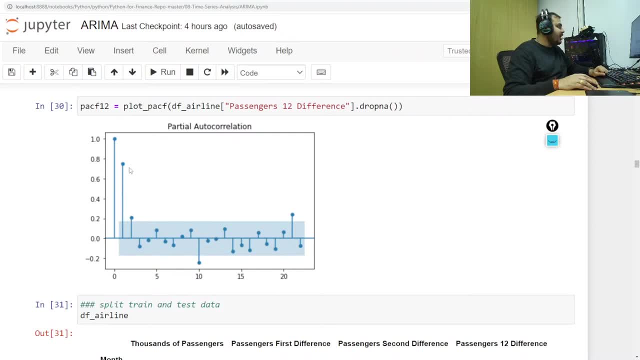 I go and do the count: 1,, 2,, 3, so I have taken 3 values over here, remaining all. I can ignore it because it is within this specific boundary. so my p-value was 3 over here. my 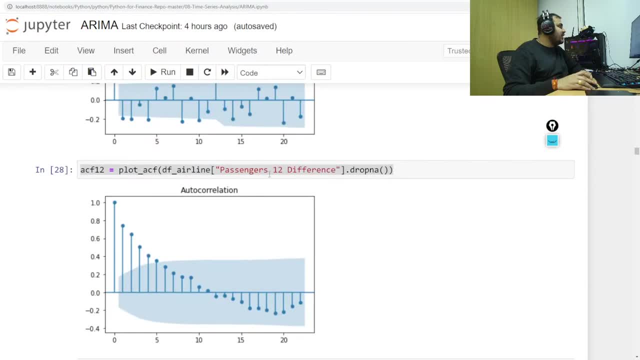 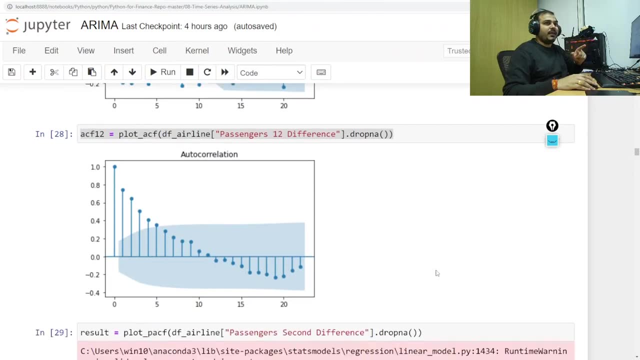 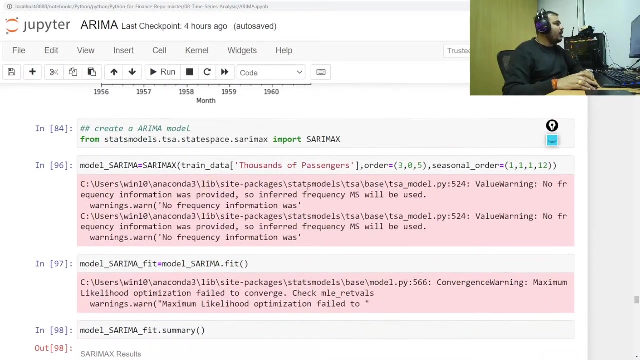 my- if I probably see, with respect to 12 difference, if I go and see this value: 1, 2, 3, 4, 5, so 5, 3, I have actually taken, ok, 5, 3, I have actually taken for seasonal data: ok, so seasonal Arimax, how? 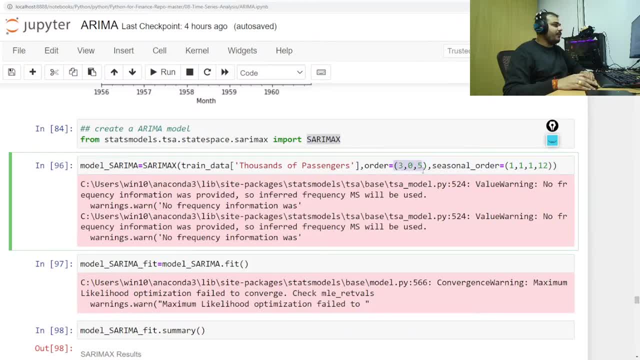 do I import seasonal Arimax? see like this: 3, 0, 5,. now why I have specifically taken this: 1, 1, 1,. ok, understand this is with respect to seasonal order. how many times differencing I have actually done for seasonal 1 time. ok, I can also keep it as 0, 1, 0,. 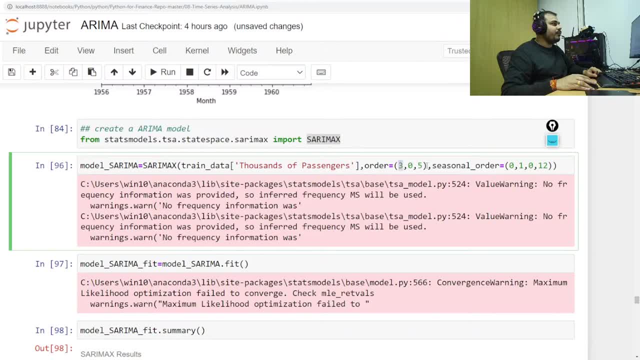 because this p and q value I am capturing from here- 3, 5.. ok, and the last value that you see over here is for the seasonal data. like 12 is the number of months in a year, right? so with respect to that, I have actually taken 12 months over. 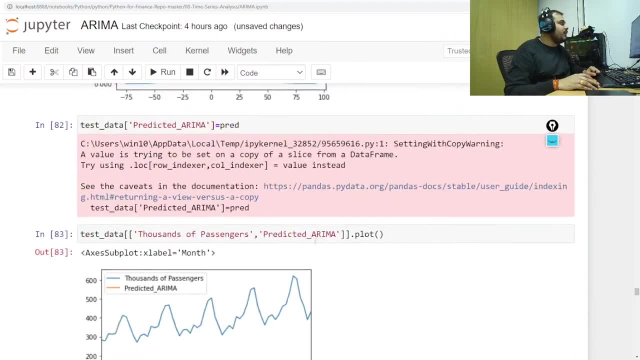 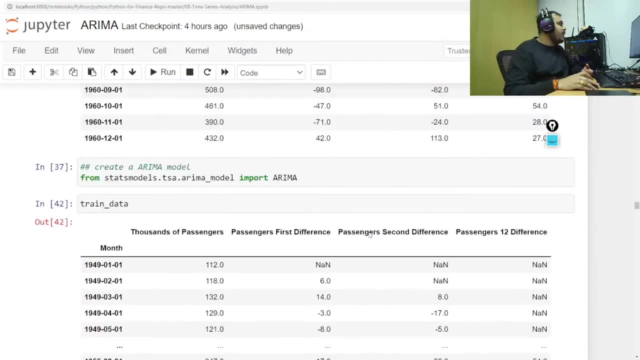 here, ok, so that is the reason I have used Sarimax for Arima. it is not giving a good model, not at all. see if I probably go and see Arima and if I see the order, ok for. 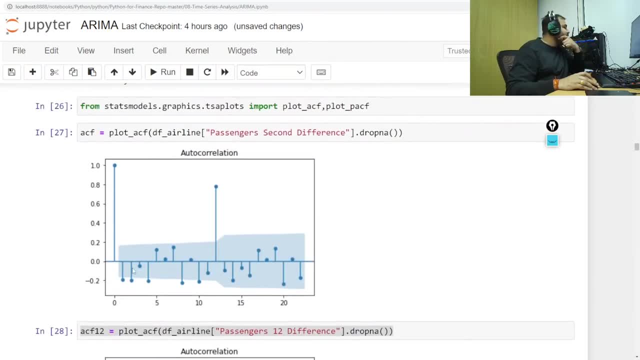 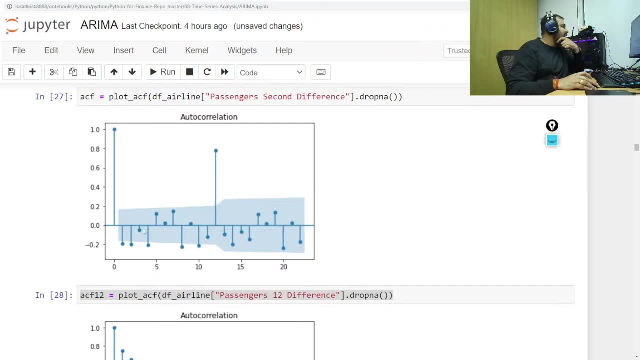 Arima. if I probably go and see the order, this is the Arima model: 1, 2,, 3, 4, 5, 6, 1, 2,. see, I can also take. I can also start by taking 3 values, ok, 1, 2, 3, because this 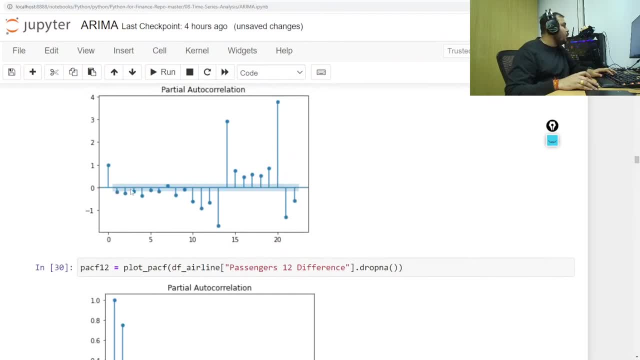 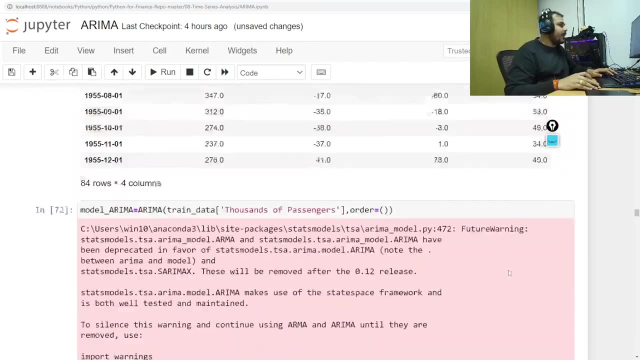 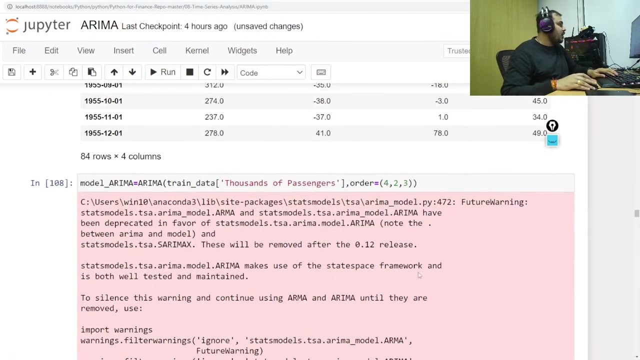 is just crossing the lower index. so let's say 1,, 2, 3,, 1,, 2,, 3,, 4, ok. so let's let's consider 4, 3, ok, I will do it wait. 4,, 2,, 3, ok, because 2 time differencing we did. 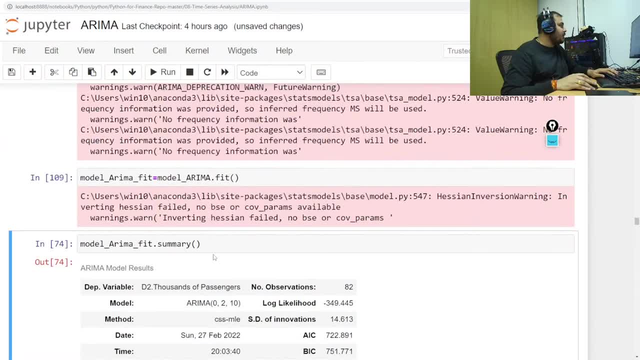 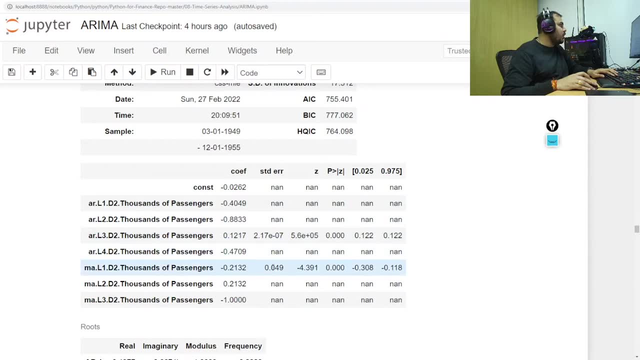 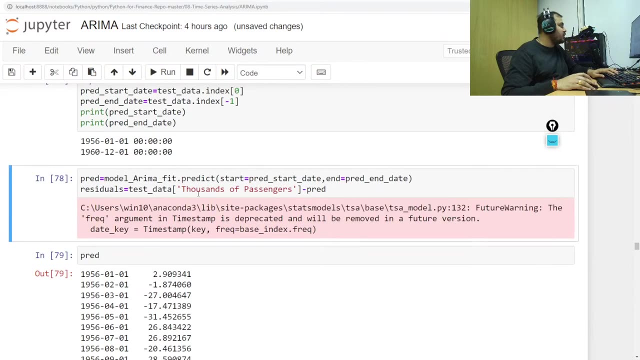 so if I probably take this up and write dot model, dot Arima effect, dot summary, ok, I will do it and here you can basically see that I am having all the nan values. ok, because it may not have any impact. so let's see the test data, let's do the prediction. here is: 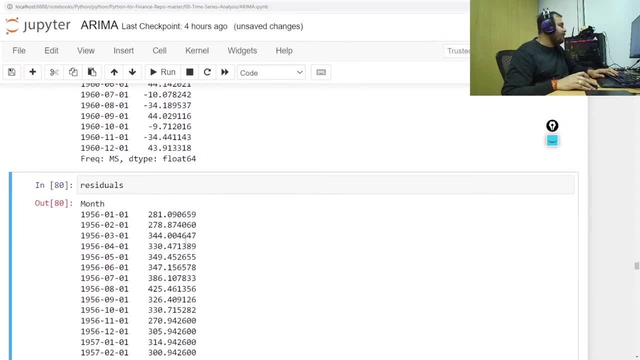 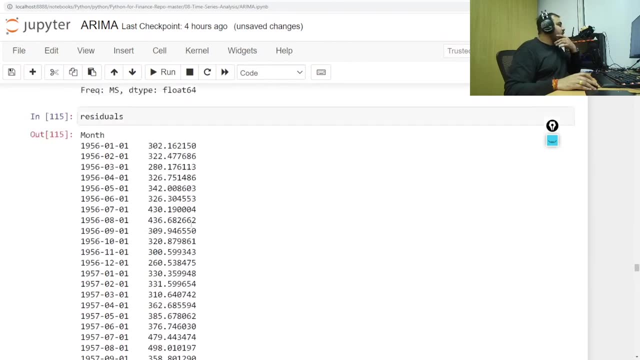 my prediction: yeah, no impact. actually, it is not giving you a good result. ok, it is not giving you a good result. so if I probably plot it over here, you will be able to see that I am getting this plot. I am getting this plot. 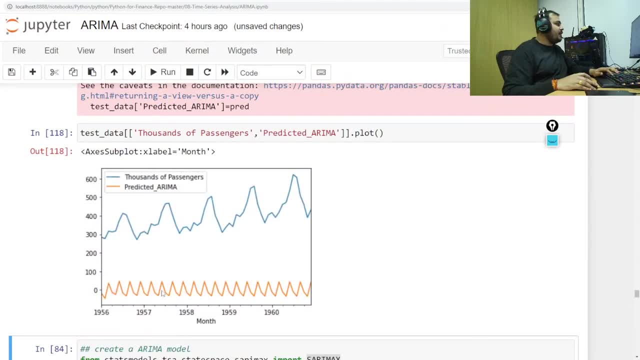 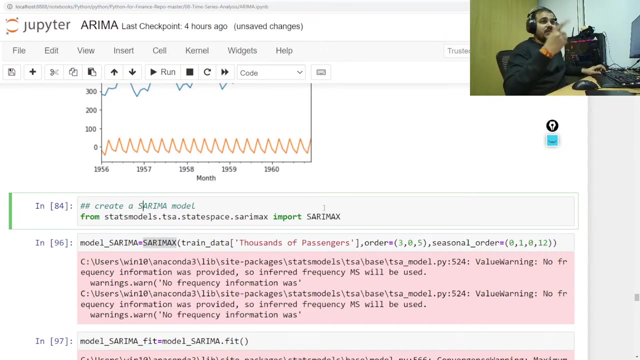 If I plot over here, it is coming like this now, ok, see this. it is a huge difference. if I am probably not having a seasonal data, ok, but I do have a seasonal data. so, similarly what I did for Serimax: everybody, you can see this Serimax, right, I know the code is. 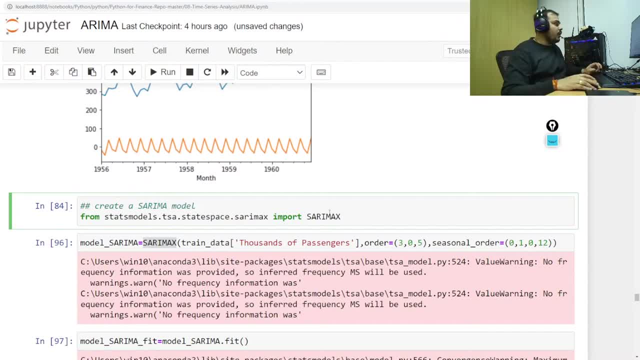 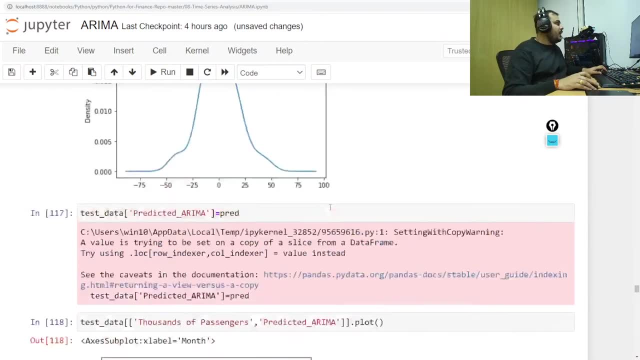 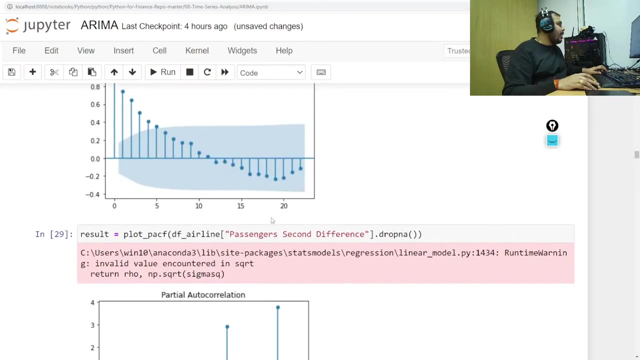 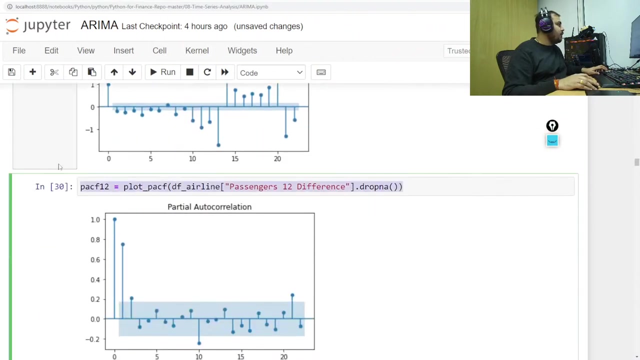 not given in your notebook, but I will give you the code. ok, I will just upload this in seasonal. can anybody tell me why I took 305?? Let me plot these 2 diagrams again. So this is for my ACF and this is for my PACF. so I am just going to copy and paste. 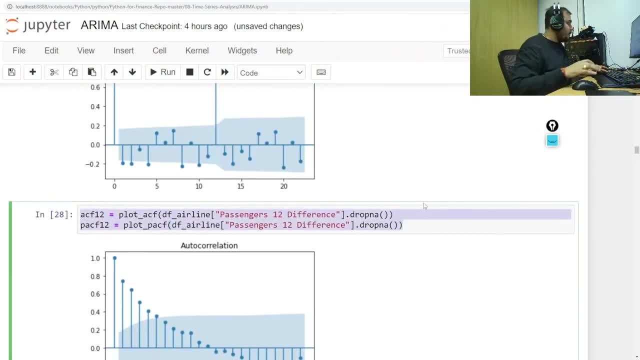 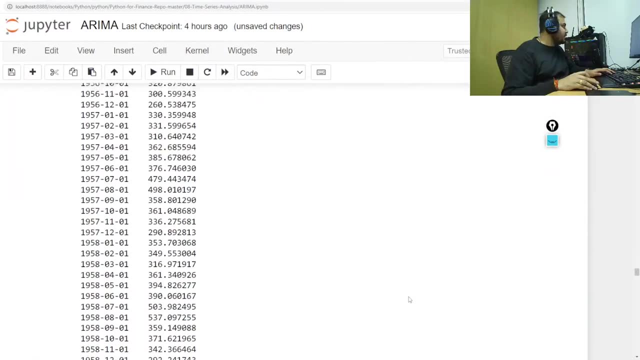 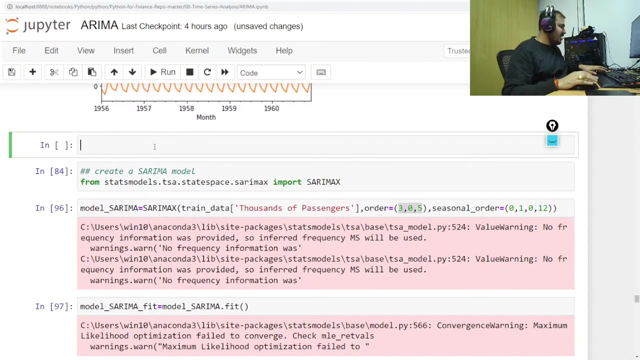 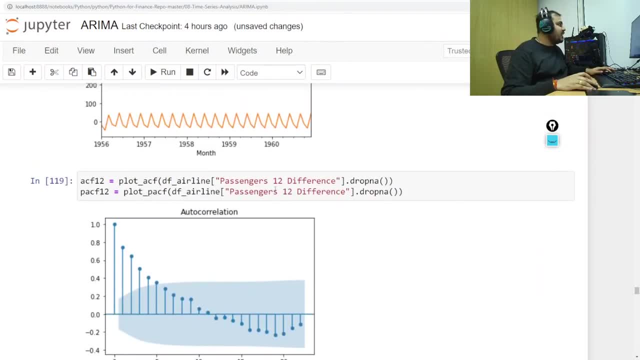 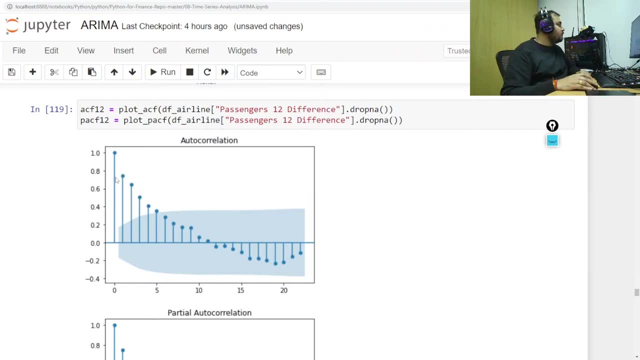 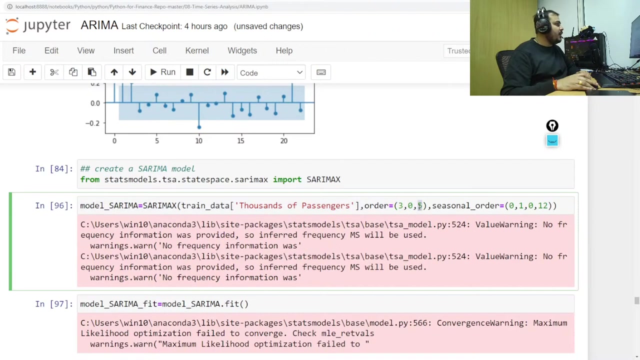 it successfully. now see in this way. why did i take for seasonal? because this is for 12 difference. this is for auto correlation. auto correlation will give you the value of q: 1, 2, 3, 4, 5. after this, everything is going down right. so i have mentioned 5 over here. okay for this. 1, 2, 3. i. 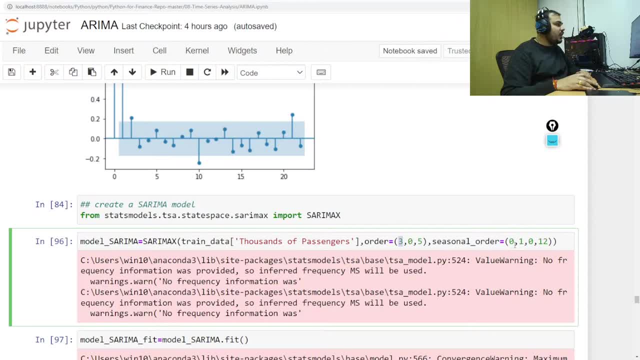 mentioned 3 over here right now in seasonal order also, we give pqd. okay, pqd, so one seasonal differencing. we have already done so. i have kept it as 1 and here i have specified as 0, comma 0, and this 12 is basically for the 12 months data. okay, so once i probably execute this here, you'll. 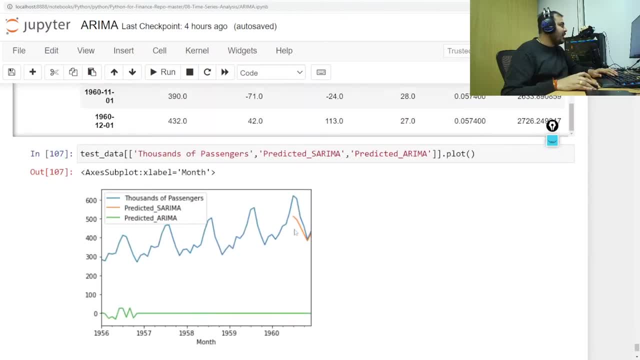 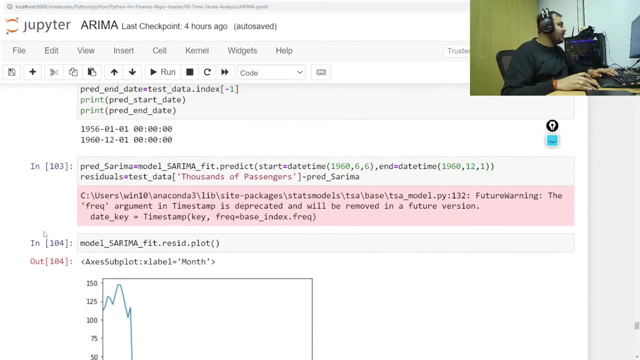 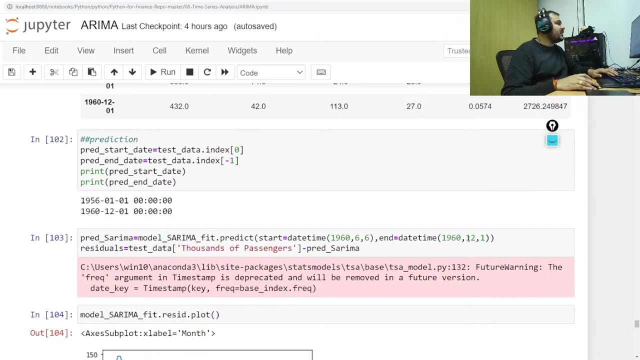 be able to see. i'm getting a good graph which looks like this: the prediction one: see the predictions one. i can also do it for the entire data data set. i can also do the prediction for the entire data set, okay, but here i have specifically told that from 1960s to 1960: 12: 1. i want to do the prediction. let's say that i want to do it from. 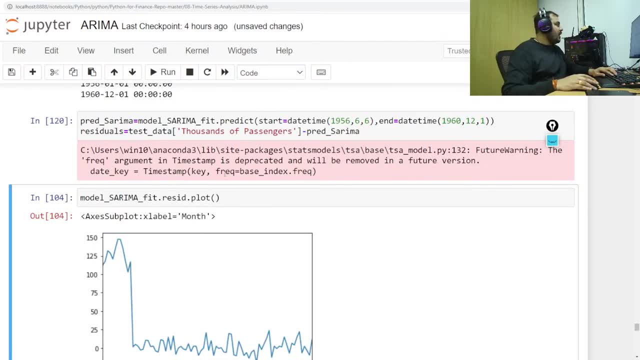 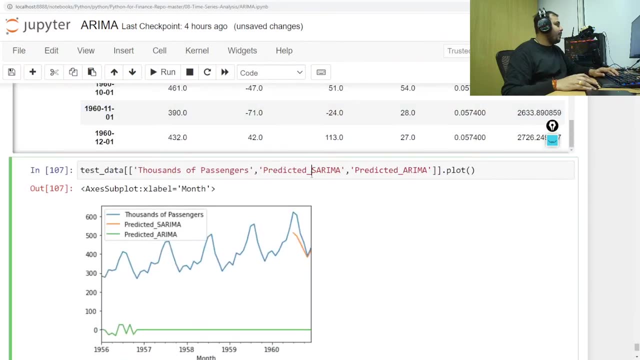 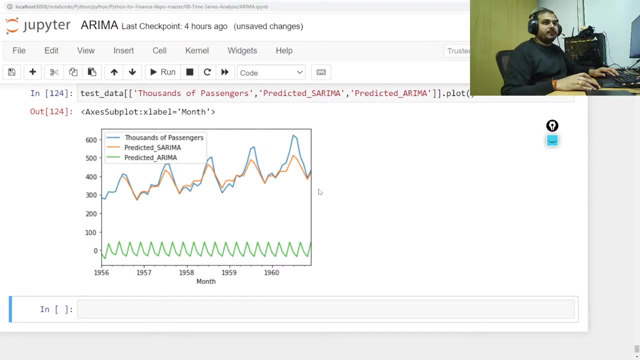 1956, and if i probably execute this plot, you can see over here how i'll get. see this graph. this looks better, right, nice. if p and q is taken to be zero, it's basically doing arima. so why is arima not working? see arima. 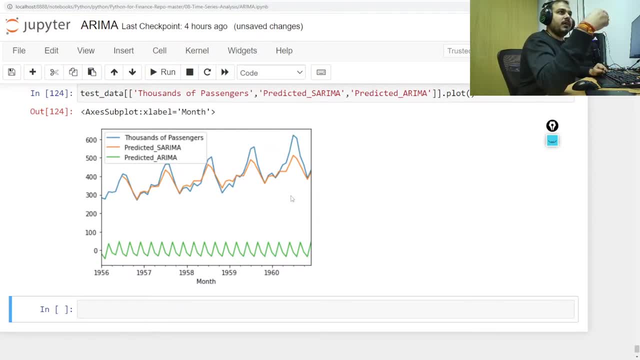 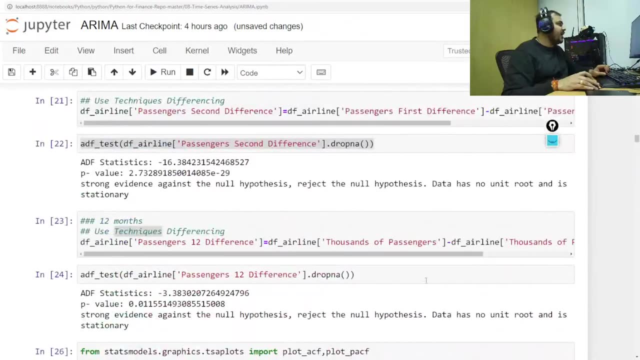 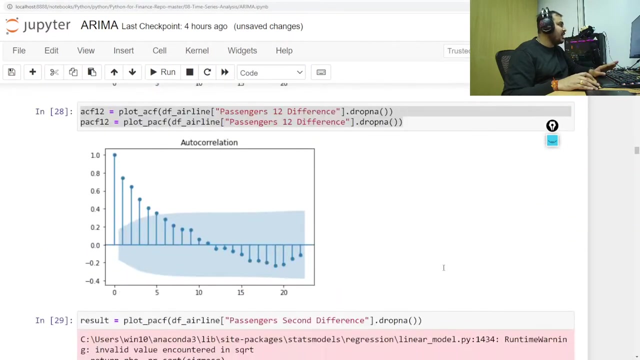 may not be working because it is a seasonal data. okay, that may be the reason. okay, internally i definitely did not do the calculation, but here you can definitely see that when i'm taking the arima value as some values over here, let's see a lot of coding, is there, guys? so don't get. 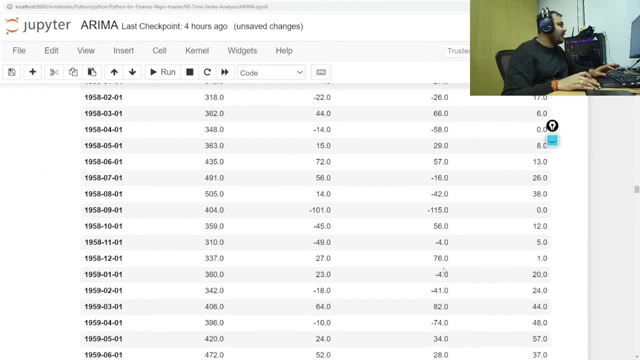 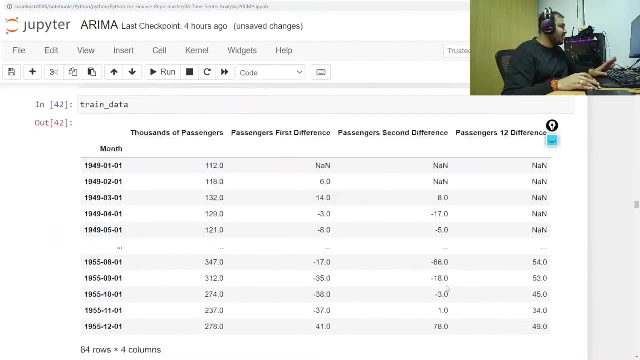 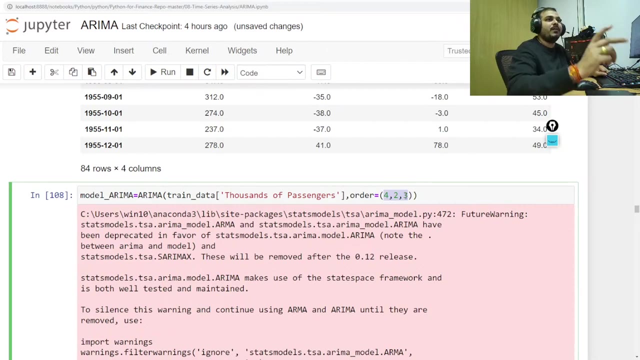 irritated? okay, there is. there is a lot of coding. okay, no need to get irritated as such, because i know it is difficult a little bit. see, here i have taken four comma two, comma three. the reason why i took it? because, with respect to the number of differencing, okay. so very simple here, even though you take zero, 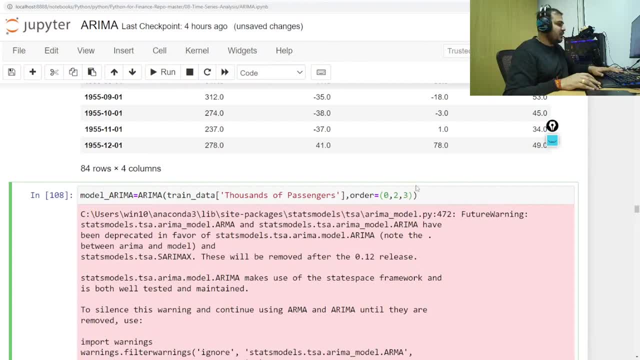 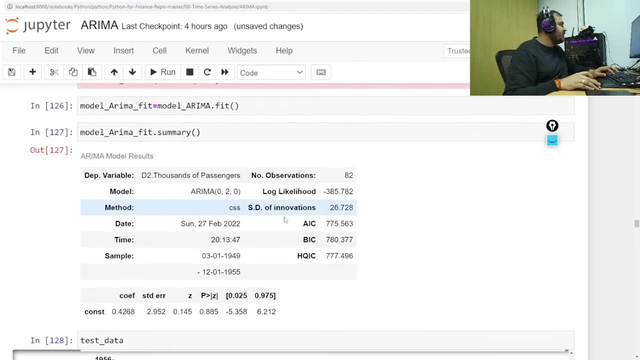 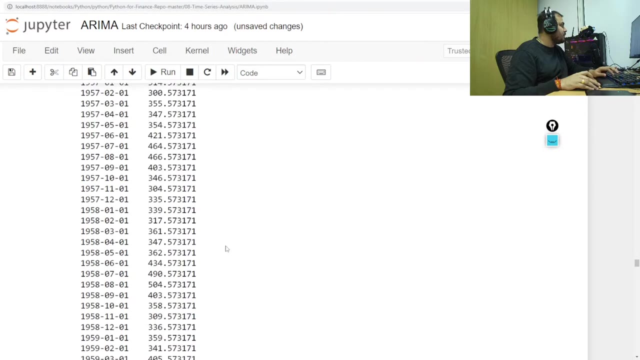 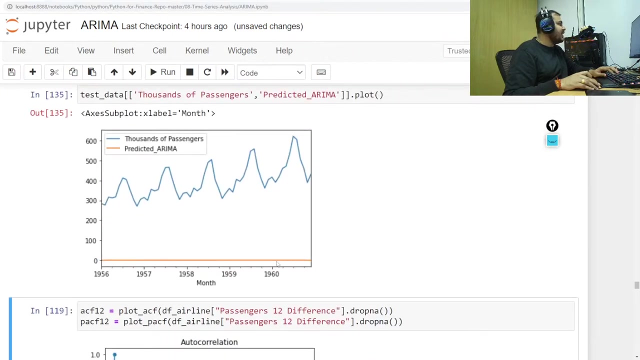 comma two, if you probably take zero also here also you take zero. i don't think so it will work because this is a seasonal data. see over here, let's see i'll talk about how you will be able to find it out. so here you can see that it is just coming as a 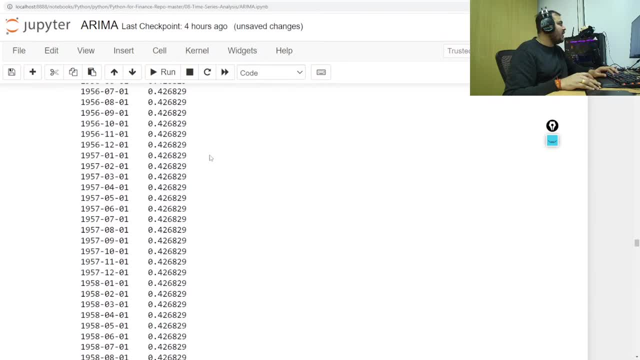 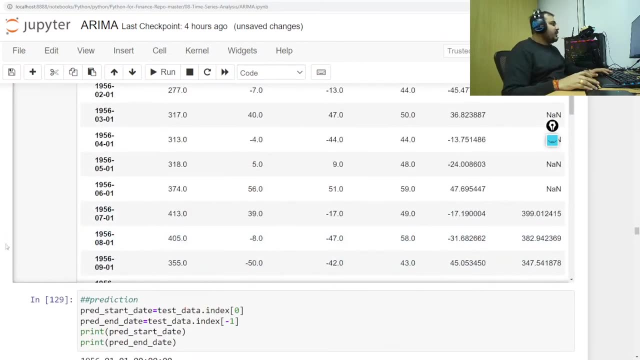 straight line. it is all point, point, point, point, point four. so usually seasonal data will not work with arima. okay, if you probably take any stock data- yes, i will talk about that later- but if you don't take any stock data, arima may work for that, but not for seasonal. that is what is basically getting. 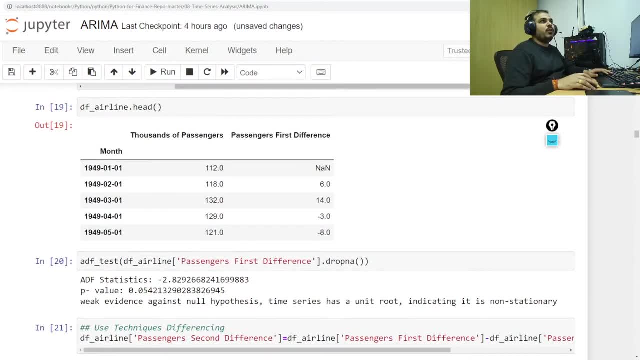 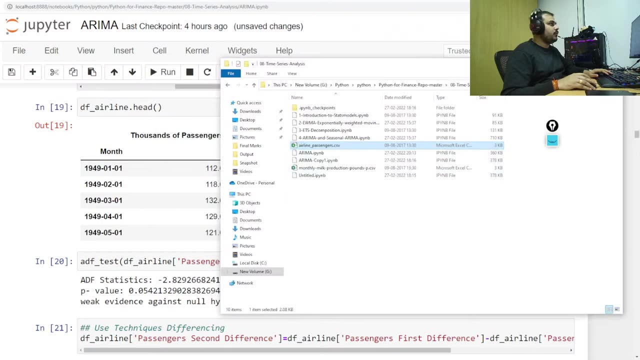 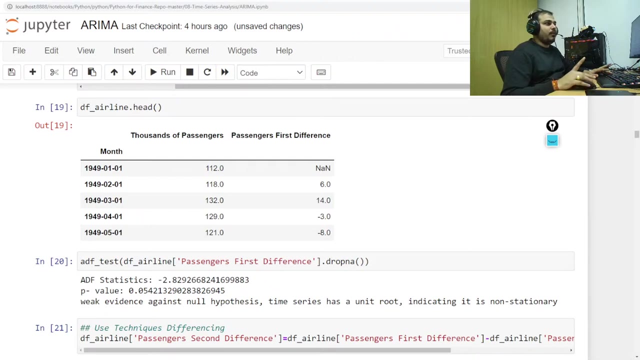 proved in this entire information. guys, do you want this notebook? everybody, let me just upload this notebook and give it to you all. i will upload this notebook in my github so that you will be able to see this, you? okay, guys, the notebook file has got updated. now you can reload the page and you can just click on the github link. 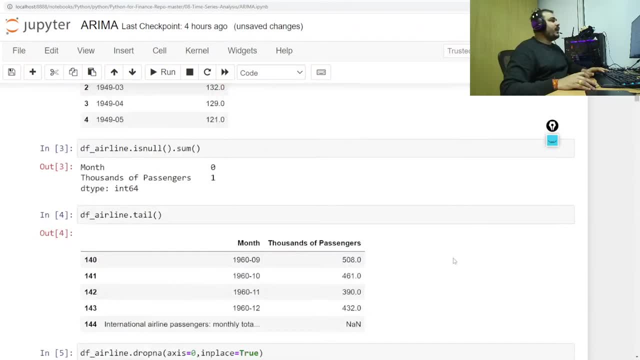 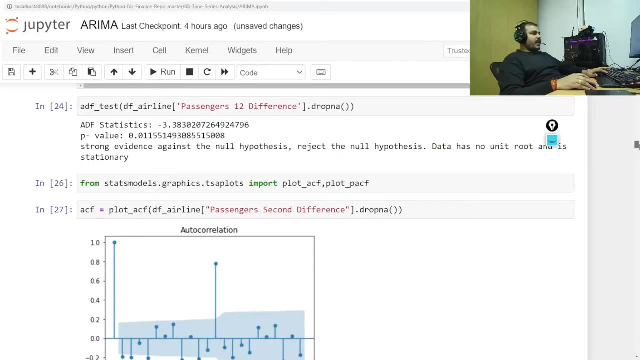 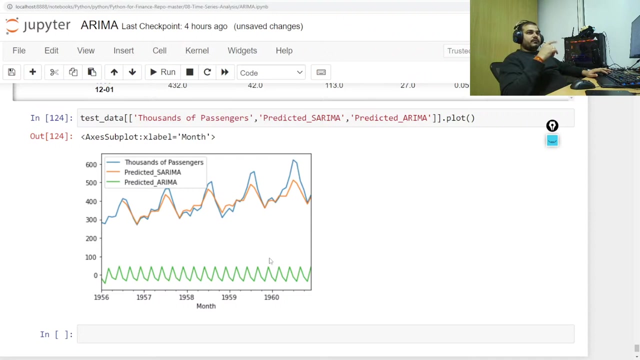 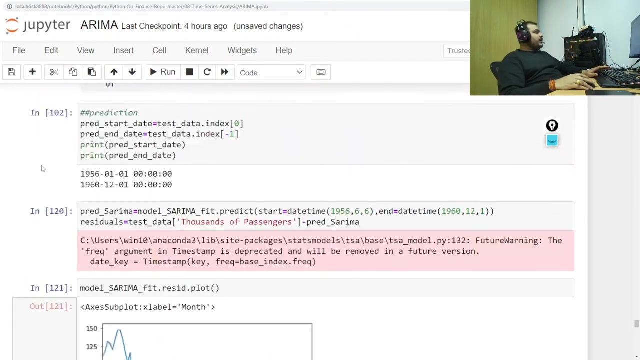 okay. so everything, all the materials that i've given over here will be available over there. see for seasonal only. it is working. it is not working for arima: see over here, Predicted Sarima is basically working. This is not working. Okay, Again, I am going to repeat: How do you find out the PQ value? 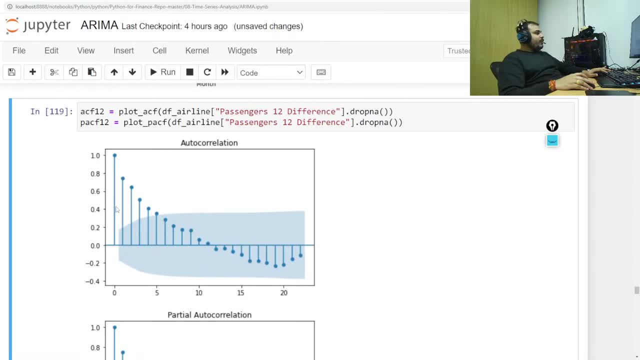 PQ value is very much simple. Just go and see that. how many lines are actually coming above this band? the upper bound and the lower bound? So here you can see. with respect to ACF, this is my autocorrelation plot. This will give you the Q value. 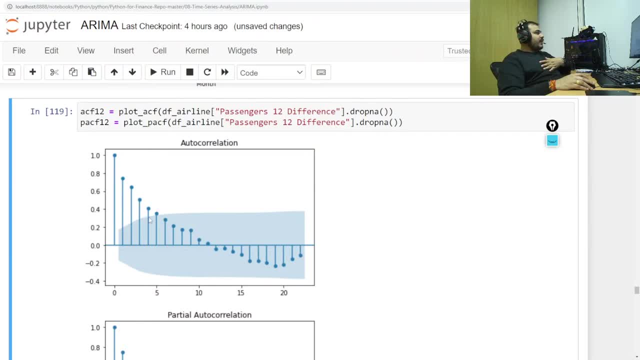 So here you have 1, 2,, 3,, 4, 5.. So 5 is there. Let's try with 6 also. and here it is 3.. Let's see, Let's try with 6 also. 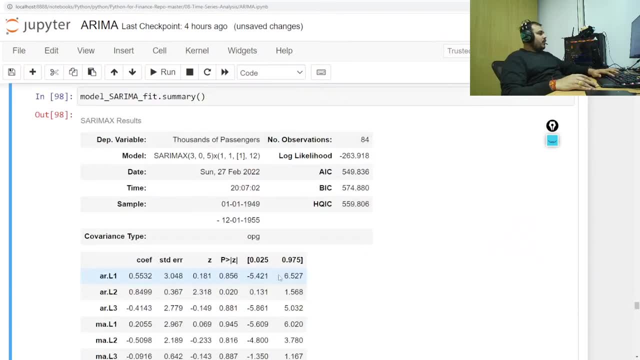 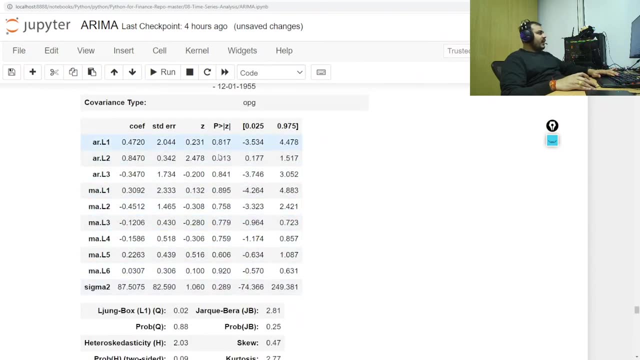 Then also you will be able to see that you will be able to get a very good value: ModelSarimaFit, ModelSummary. So here you can see all the impacts with respect to the negative values, positive value, everything you are able to see. 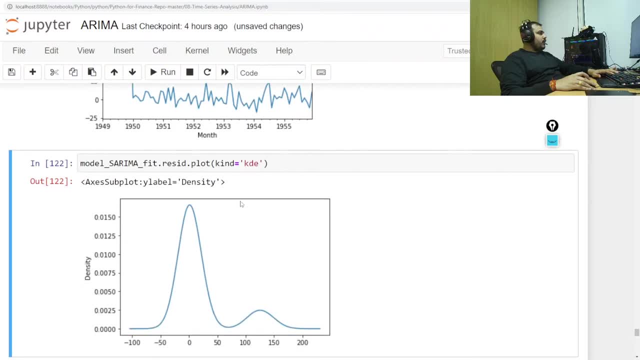 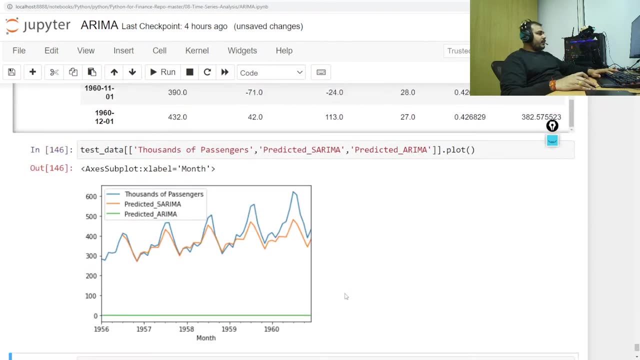 This will be your tail. This, this Residual plot. Not much difference, but, yes, You will be able to. You will be able to see something, but a good graph you will be able to get. So like this it is basically looking: 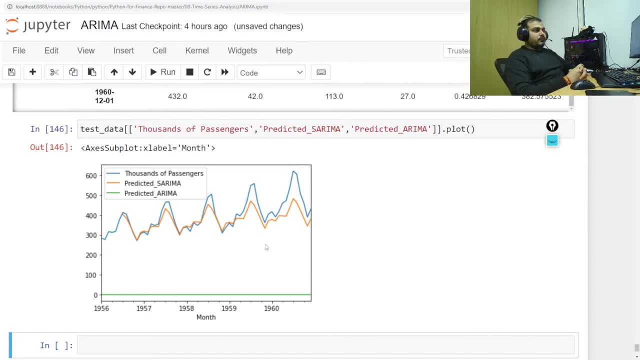 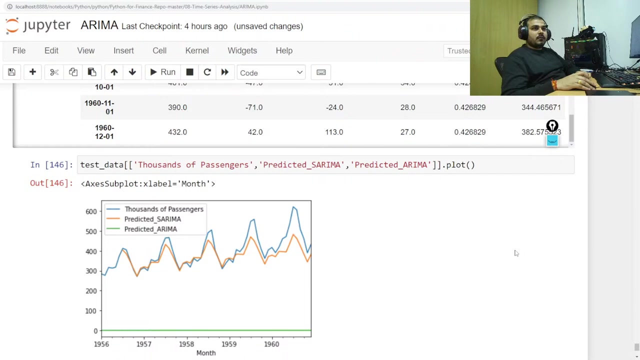 Please download the code, everybody, Everybody. download the code in the GitHub. Arima failed in this data, In seasonal data. Arima failed. Yeah, Do we not consider the boundary below? Yes, we are considering over here also. no, 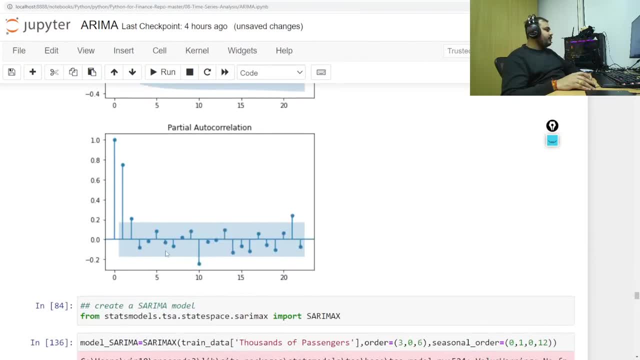 Do you see any points? that is crossing the lower boundary. From here you can see right after many range of values. here it is coming down. Okay, So I have taken this first: 3.. 1,, 2,, 3.. 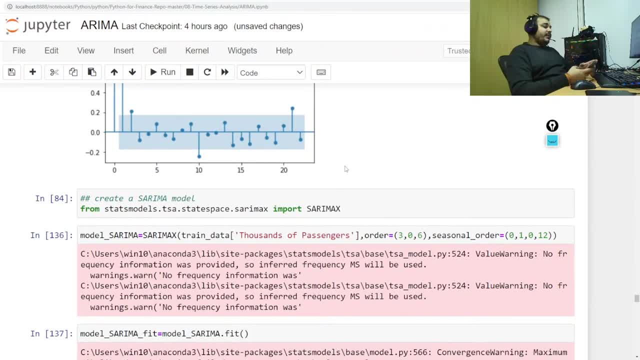 But definitely seasonal. Arima is working in this. Try it with stock data, Try it with stock data. I think it will work. Arima will work with stock data. Arima may work with stock data. guys, You want to do stock data everybody. 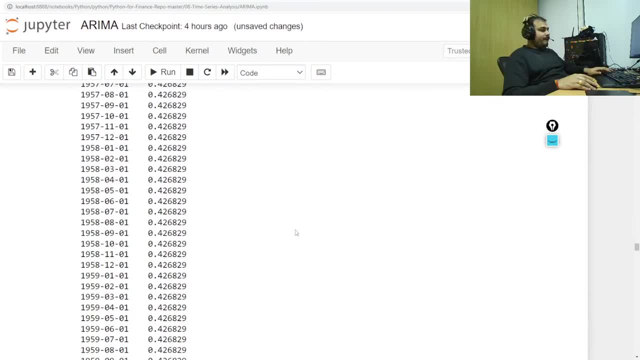 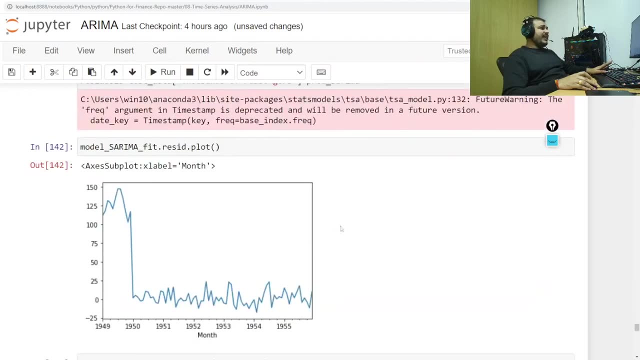 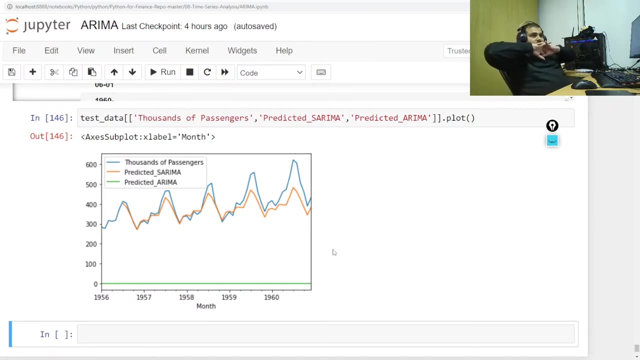 Stock data. But don't worry, What I will do is that I will create a separate playlist with respect to time series. I want to create in a better way all these things. See again, it will take one hour time, Okay, So don't worry. 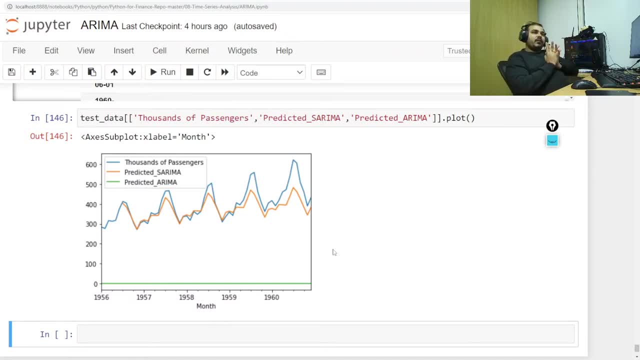 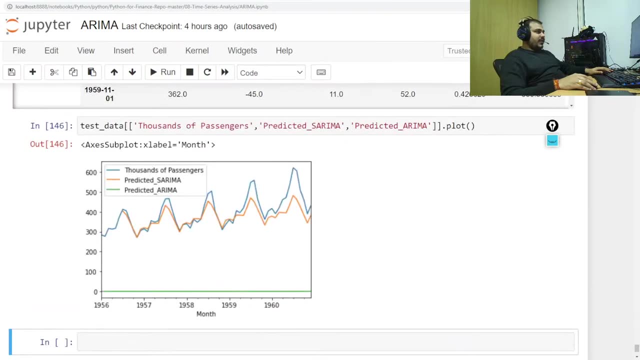 I will create a playlist and entire videos. I will create it for you, Okay, And that will also include mathematical intuition. So did you like today's session? Everybody? I know it is little bit tough to understand because in finance a lot of math things are used. 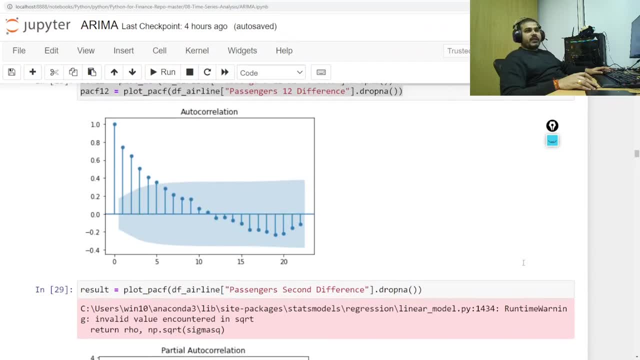 Okay. So if you are probably understanding math, that is well and good. So tomorrow I will not be taking any session, guys, because I am not going to use deep learning right now. because deep learning, I want to take a 7-day session and then probably cover all these things- how we can do time forecasting with the help of deep learning techniques. okay, 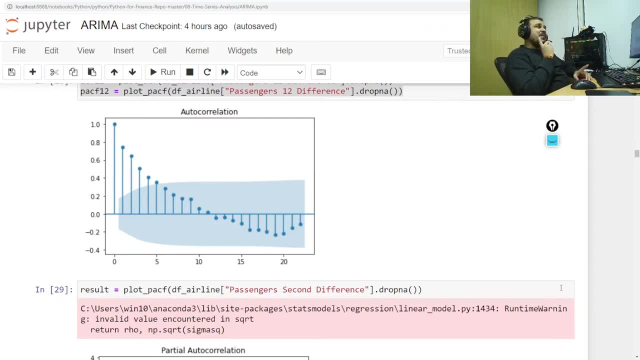 So, yes, try it out entirely and just wait, and just give me a 1-day session, and then we will see how it goes. Okay, So I will see you in the next session. Bye, Bye, Bye, Bye, Bye, Bye. 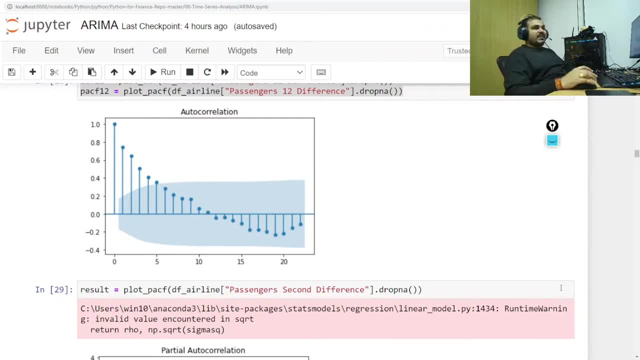 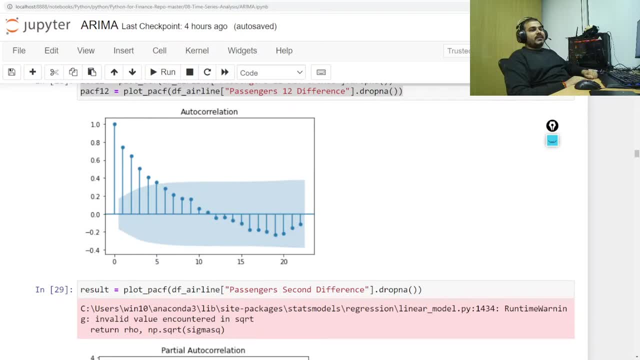 So, thank you everybody, Have a great day. and yes, probably in just 3-4 days I will be announcing the deep learning session also, okay, So, thank you guys, Keep on rocking. Hit like, At least make it 200, okay.